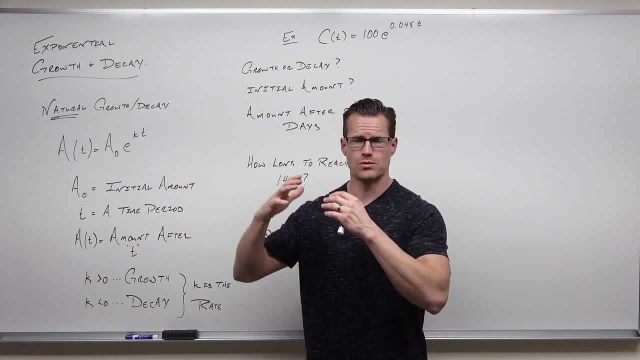 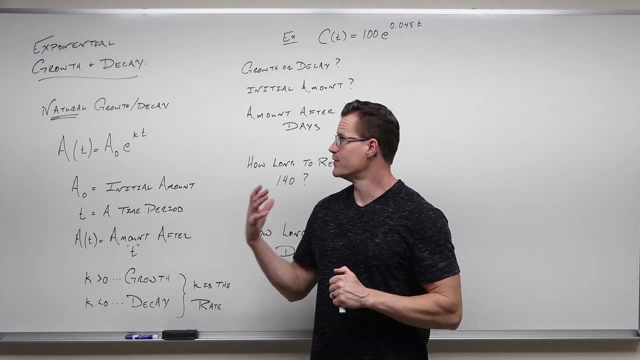 opinion, you need to understand a little bit more about this in order to really make that make sense. Otherwise it's just a formula and you can do it with a formula, but it's much better if you really understand it. So this: 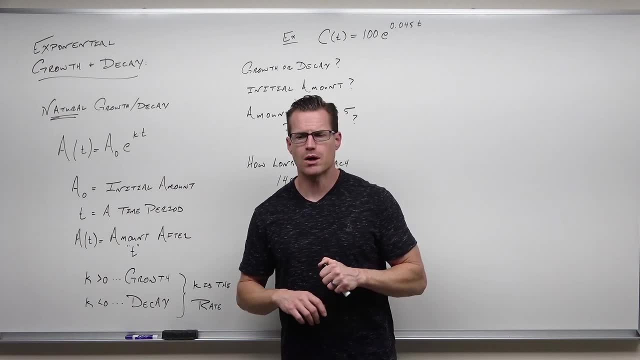 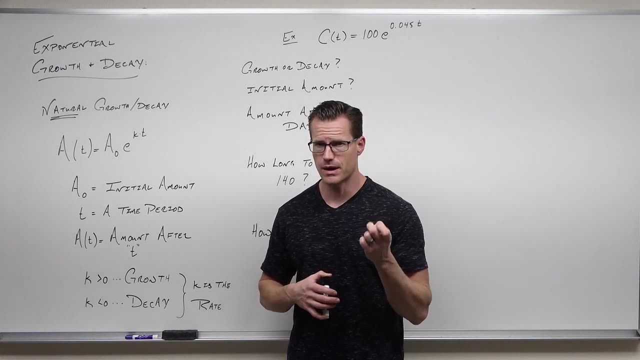 we can understand because it's based on exponential. So we're going to get into it. We'll talk about what it means. We'll take a look at it as an exponential function. We'll notice it's very, very strongly related to continuously compounded interest. It's the same, And then we'll deal with. 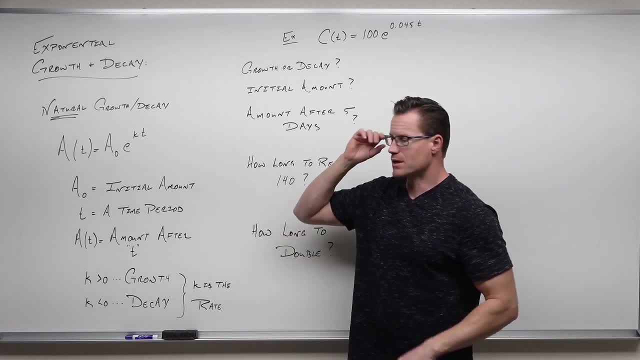 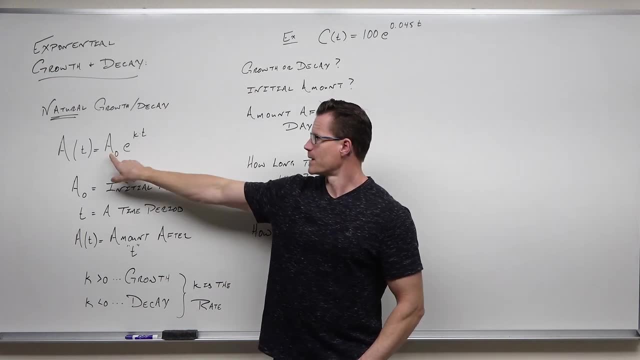 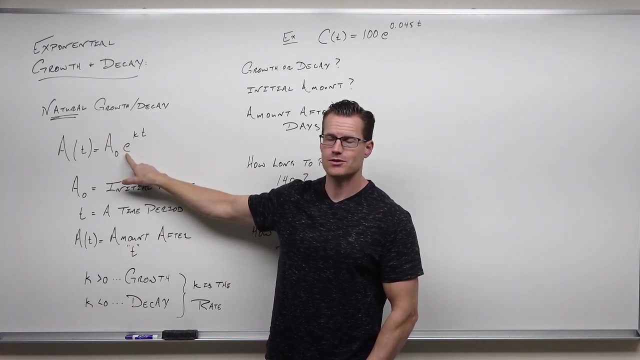 three examples on on on working through this. So firstly, the the look of it. this looks just like continuously compounded interest. It gives you a present value or an initial amount. It says you are adding to it All the time, just like continuously compounded interest. was every moment, every minute, every second, every day. This 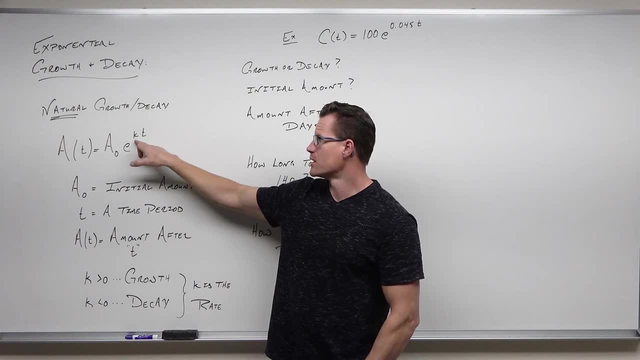 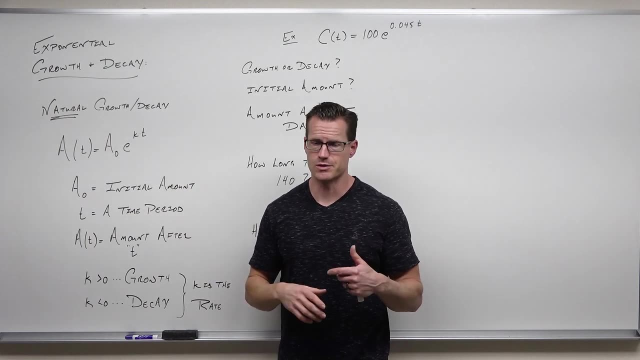 population is growing or declining based on some sort of a rate- That K is your rate- and some time period. Now, the T does not have to be years, it can be minutes, can be hours, can be whatever we want it to be. 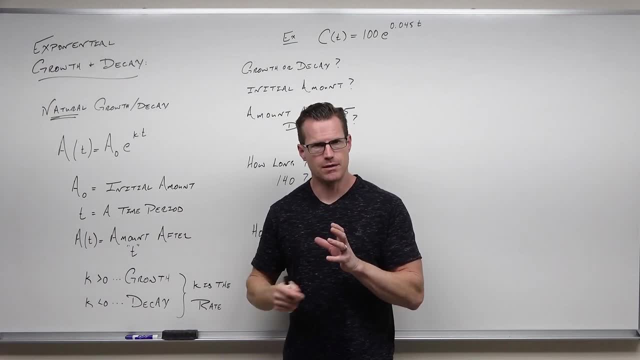 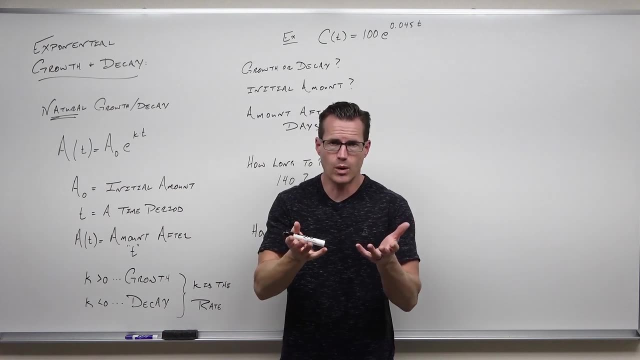 But it is a period of time. I hope that you're seeing that this is just like continuously compounded interest. It's just we're we're growing population instead of money. A population of whatever it is is just a population of dollars and cents Very, very valuable for us. Now, one thing that we're 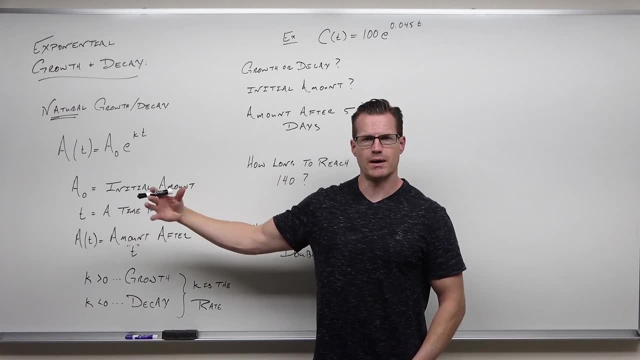 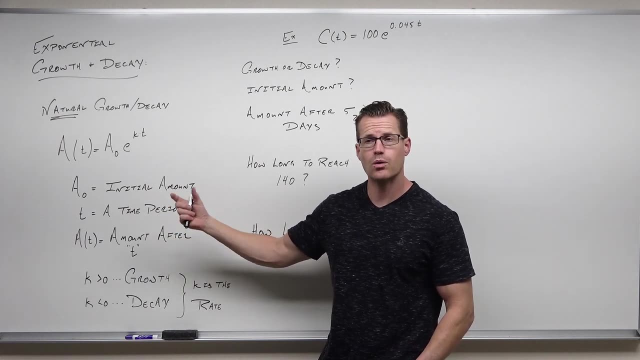 seeing. I've just already defined them. but A sub zero is your initial amount. It's like your principal or your present value. T is a time period, not necessarily years, And A is your future value, or how much is going to be in that population after a certain amount of time. 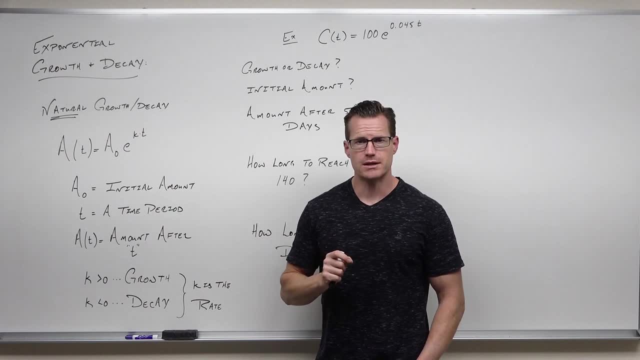 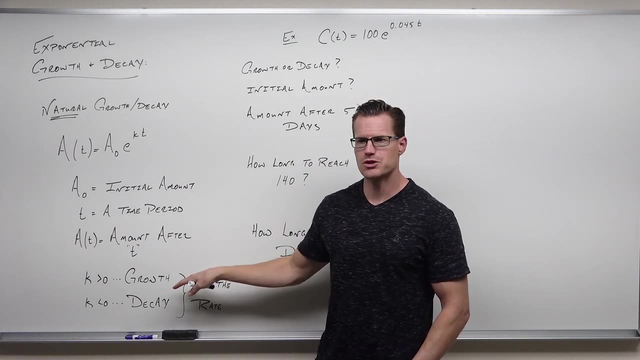 after whatever that time is, The issue here that we have is the rate You see in compounded interest. your rate is positive, meaning you're always growing money. Well, for population growth or decay or decline, we have to have the ability to have a downward or decreasing 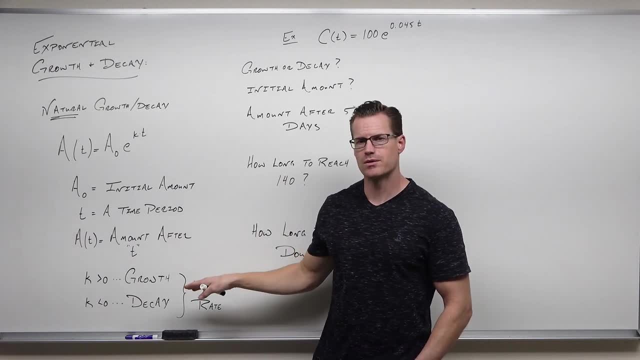 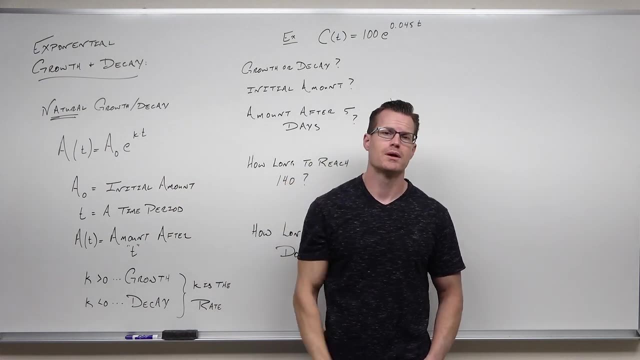 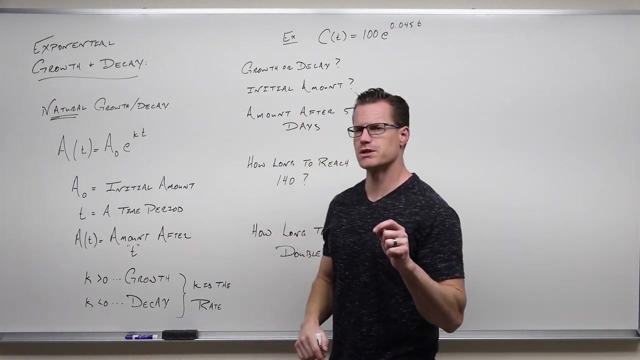 graph, And that would be exponential decay. That depends on whether the K is positive or negative. Positive Ks mean growth, Negative Ks mean decay. So why? Why would that be the case? I really want you to focus here, because if you put a negative right there, what does? 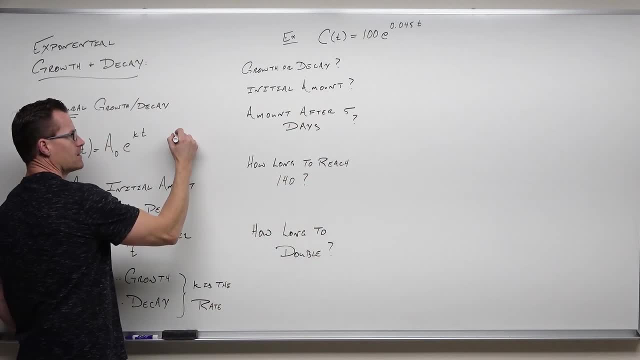 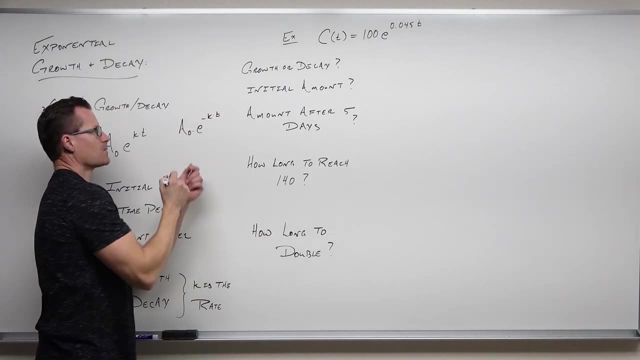 it actually mean. Check it out. If this had a negative K, then this piece right here. you could move that to the denominator of some fraction, or you could create a fraction itself. Do you remember? I've showed it to you one time before. 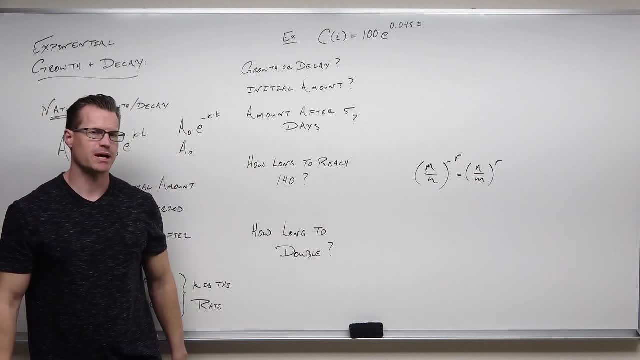 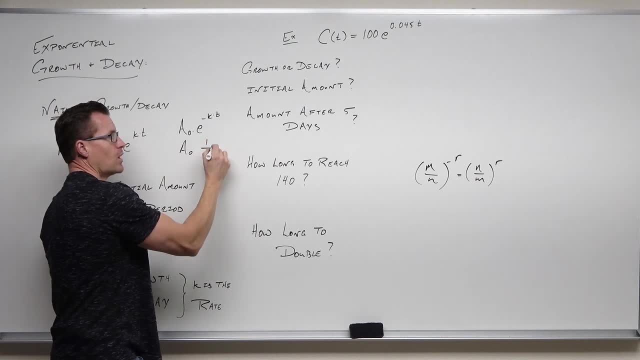 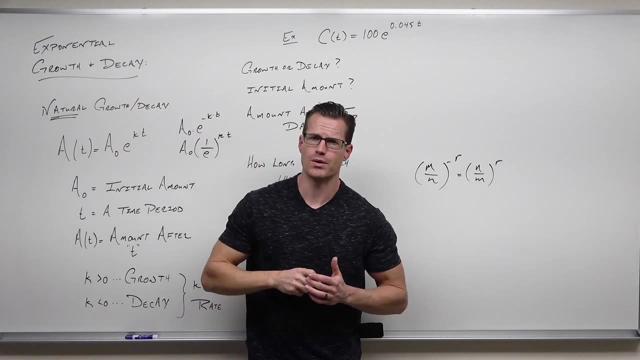 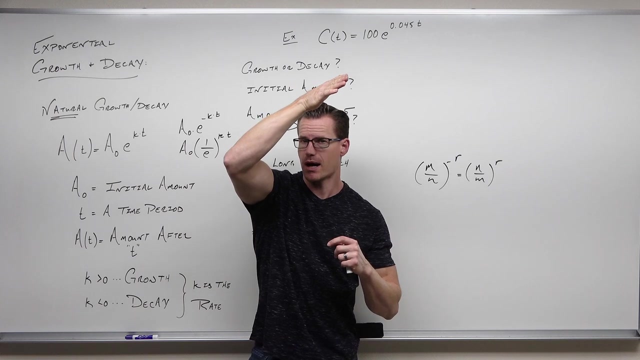 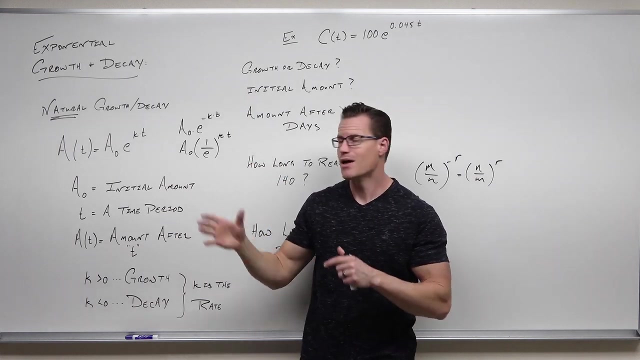 to the negative kt, I think is 1 over e to the positive kt. I really need you to make this connection. Do you remember that with exponentials, if bases are more than 1,- 2.7, we get climbing graphs. If bases are less than 1, that's 1 over 2.7, we get declining or decreasing graphs. This 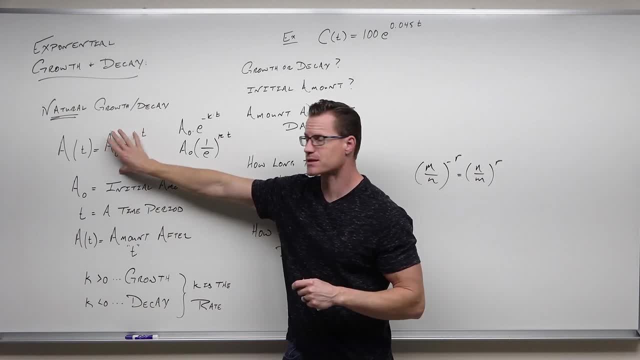 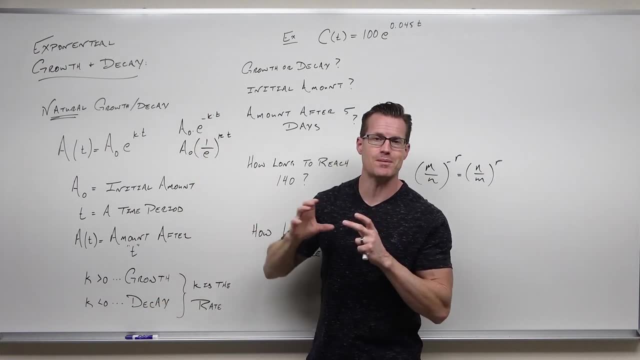 is why a positive k means grow- It's this- Or a negative k means decay, decline, decrease. That's because it's this. That negative exponent creates that base that's less than 1.. I hope you're seeing it. We don't really show this very often, but I wanted to make that connection. 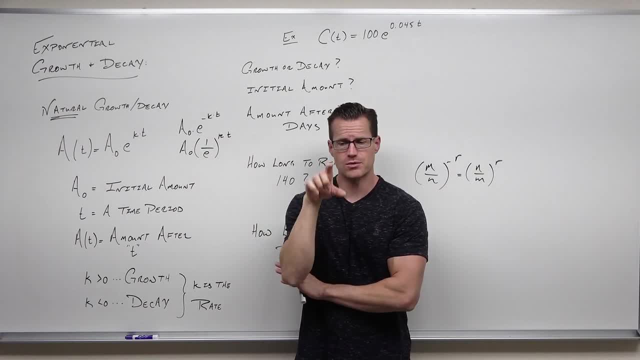 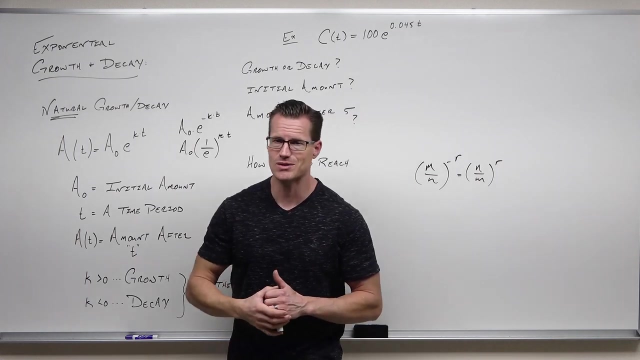 Otherwise you go. why does negative k actually do that? Because it creates a fraction. Because it creates that fraction that's less than 1, giving us an exponential function with a base less than 1.. That is a decreasing. That's why a negative exponent here decays. I hope it's making sense to you. 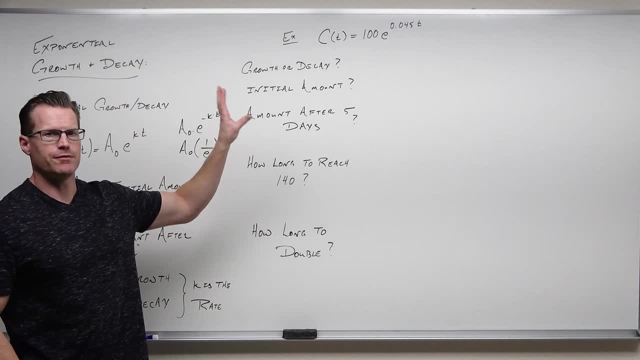 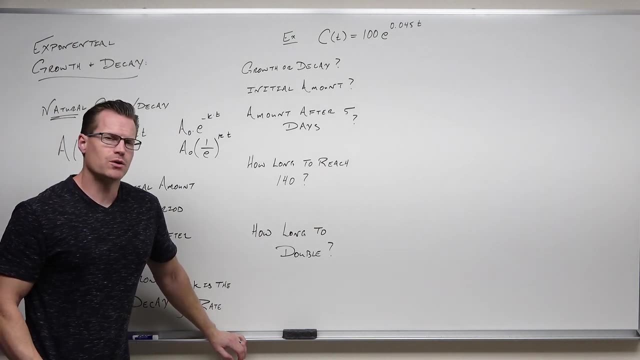 We're ready to go through a couple examples. We'll go through a very basic one, one that I've contrived for you here. Then we'll go ahead and come up with a couple on our own, one with growth, one with decay. Then we'll do Newton's law of cooling, which is kind of cool, and we'll be. 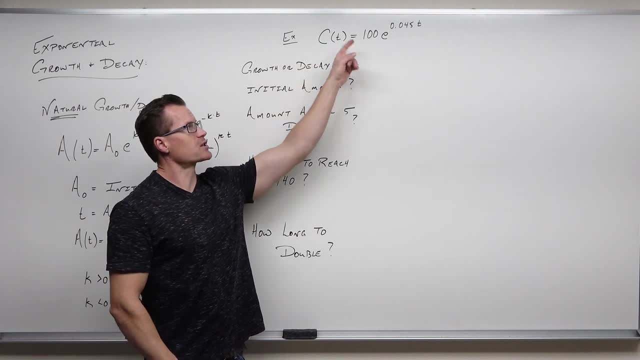 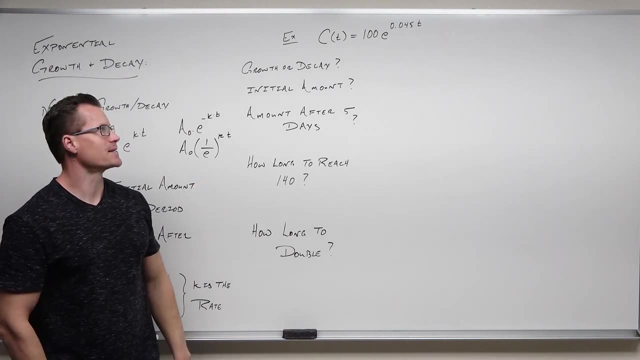 done. Let's suppose that we're given some sort of an exponential model of a population. This, in this case, was bacteria. I think It starts with 100 units of bacteria and it says that you have this 0.045.. What's that mean? For a certain amount of time, let's say it's 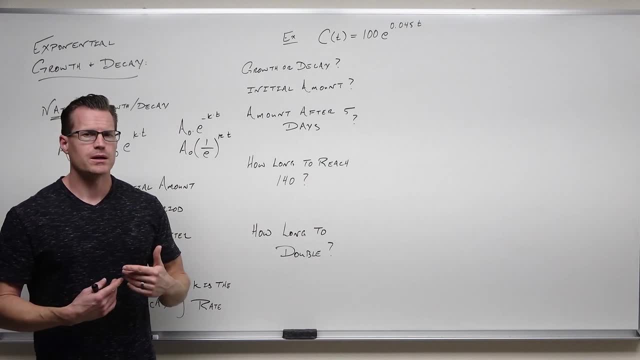 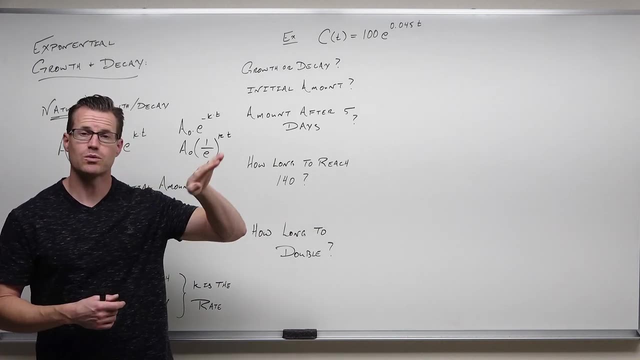 in hours. Can we figure out a few things about it? Number one: can we determine whether this is growth or decay? If you look at your rate, positive rates mean growth For some reasons I just explained to you. negative rates mean decay because they would create a base, that's. 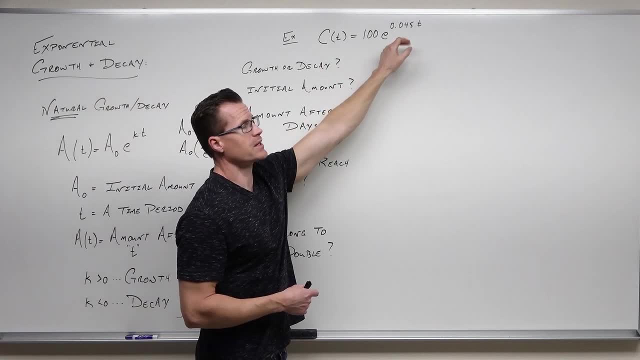 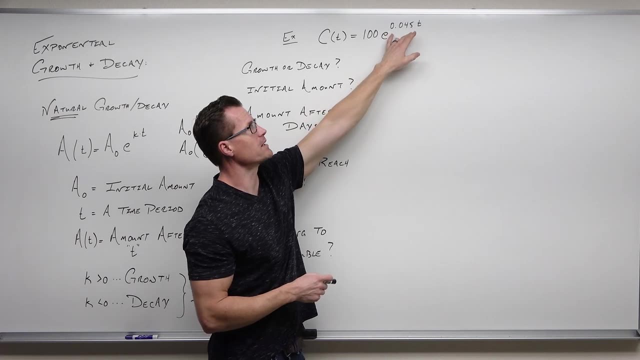 less than 1.. This is a base greater than 1, because that is positive. If that's negative, we could create a base less than 1.. That would give us a decline. Positive rates cause us to grow. This is definitely growth. 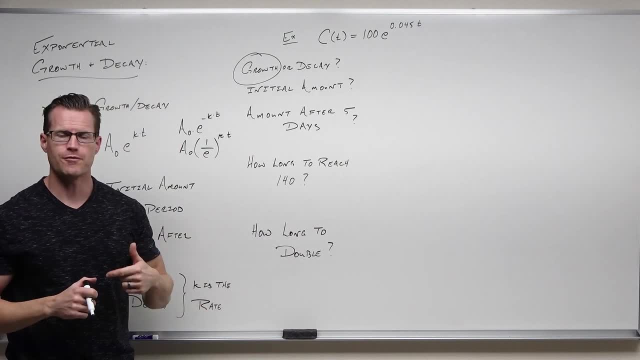 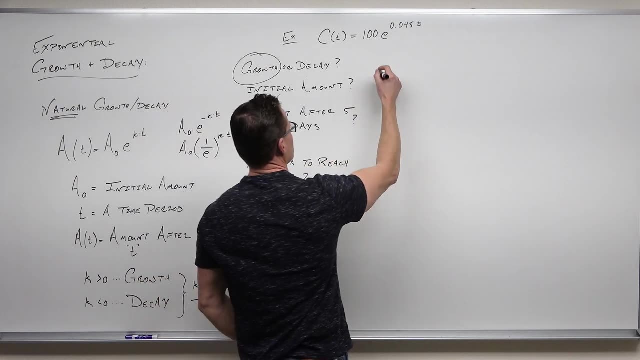 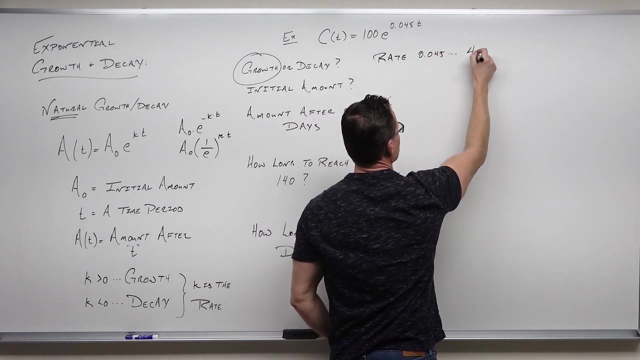 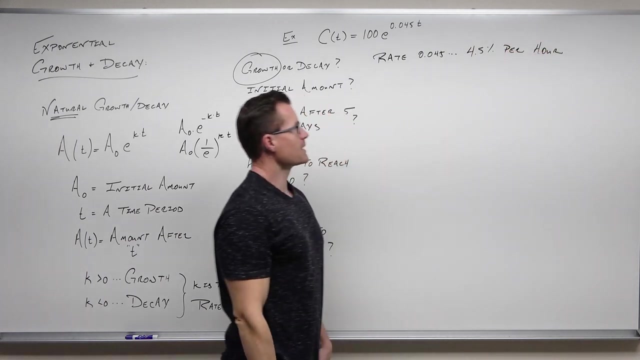 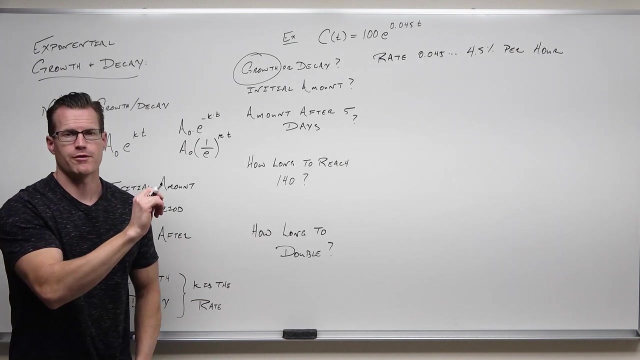 You could write the rate. The rate is 0.045, or 4.5% growth per time period. Let's say that if our time is hours, that would be 4.5% growth in hours Every hour. this bacteria is growing 4.5%, 4.5% every single hour that's happening. 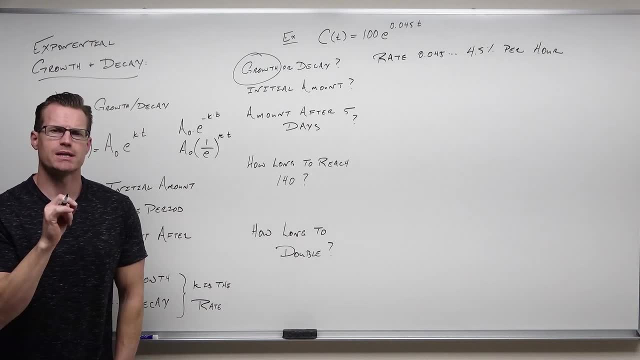 Now, how about the initial amount? The initial amount is always that number in front of your E Man. just think about doing the continuous compounded interest, how your initial amount was your principal or your present value. It's the number in front, Your initial amount. 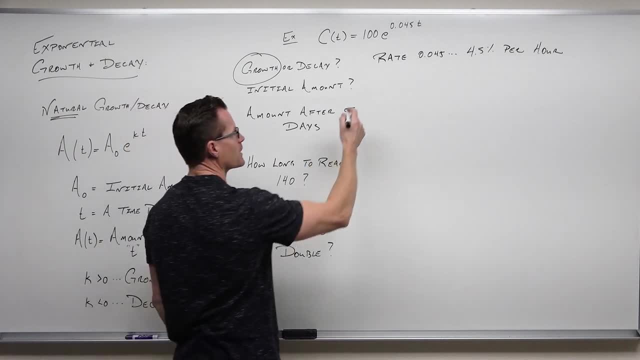 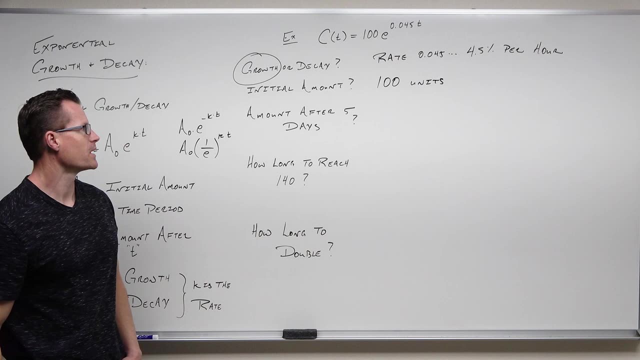 is 100, whatever this is units of bacteria or grams, Something like that. I'm going to leave this unit list, I'm just going to put units. How about the amount after five days? Well, because this is asking you for a certain amount. 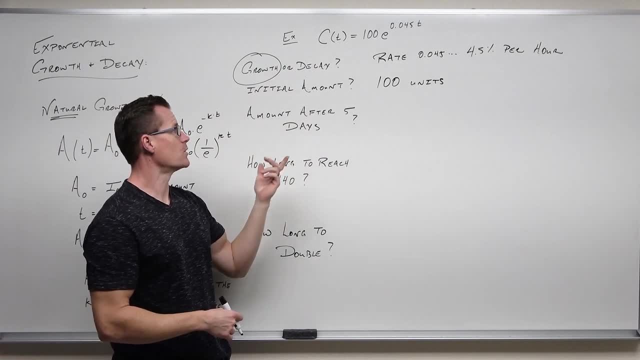 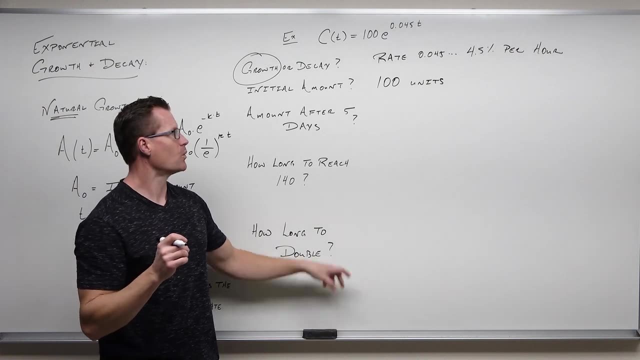 the colony size after five days' time. oh, you know what It says: days, so our hours was wrong. We always have to match this up. This would be a mistake and I'm glad I put it. I want you to really learn from it, Whatever unit of time they're telling you, so this. 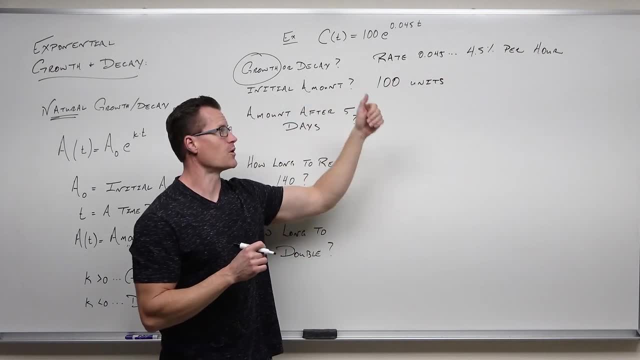 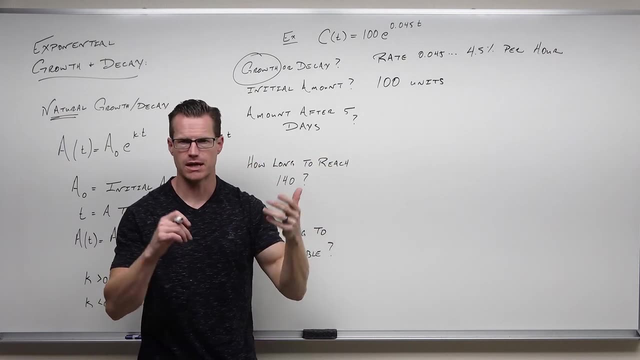 would be days. you need to match that. If I say 4.5% per hour, that really conflicts with our days. so make sure that your units of time- because they can be hours or minutes or days or weeks or whatever- make sure they. 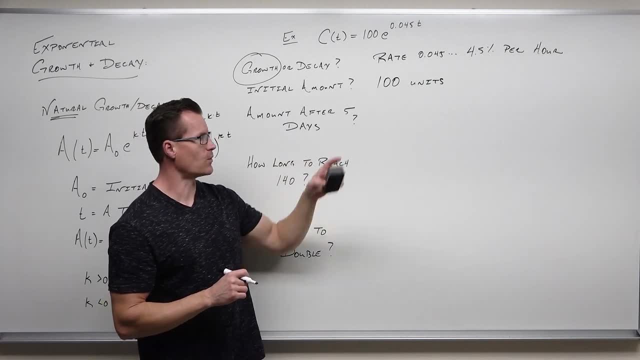 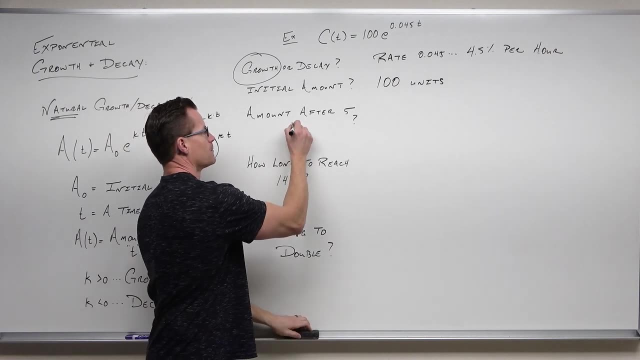 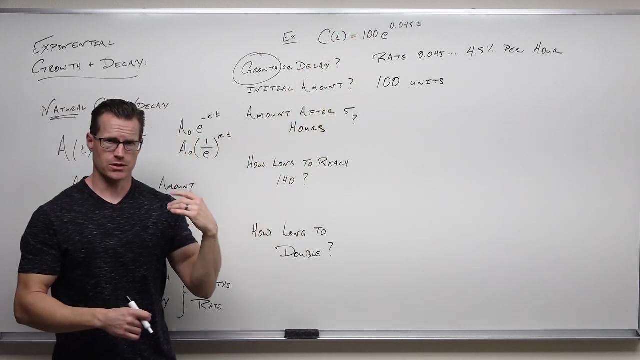 mesh together. I actually meant hours here, which is why that was I just wrote days. so good thing we got this. I'm going to change that to hours so that I can match that up. 4.5% per hour, 100 units initially. It's called our initial amount, It's like the present. 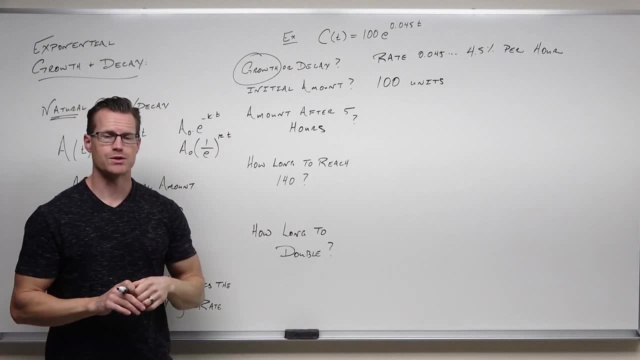 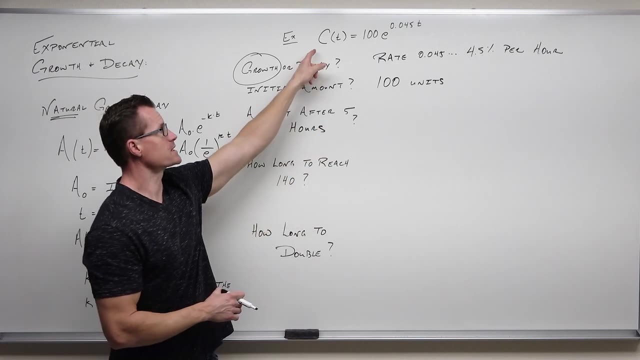 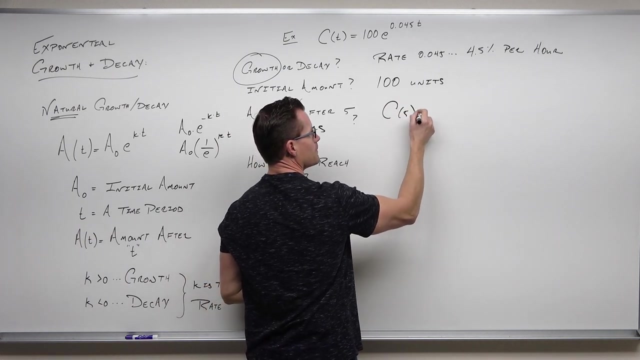 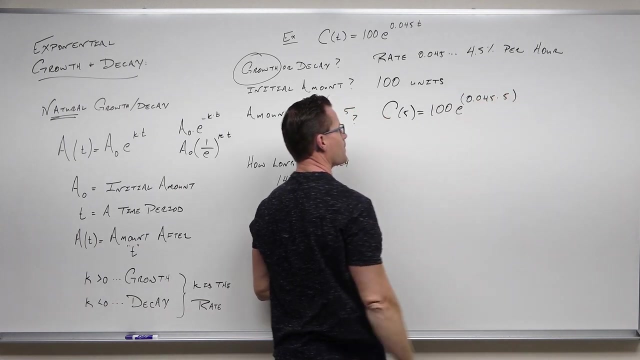 value. We're going to do a calculation: How much after five hours? Well, because this is the colony size after a certain amount of time, all it's really asking you to do is plug in five. So C of T. well, our T is five hours now, Just plug in the T of five. 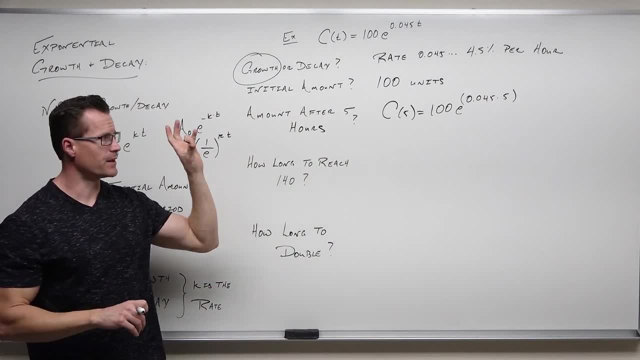 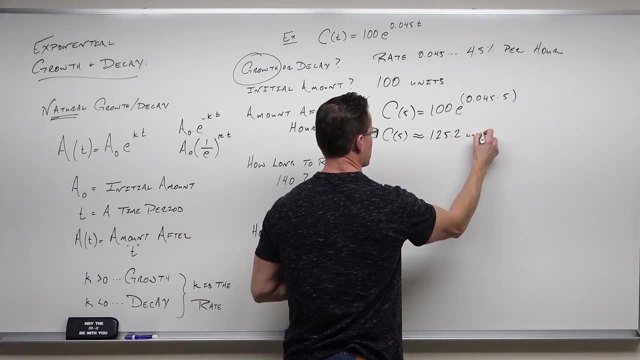 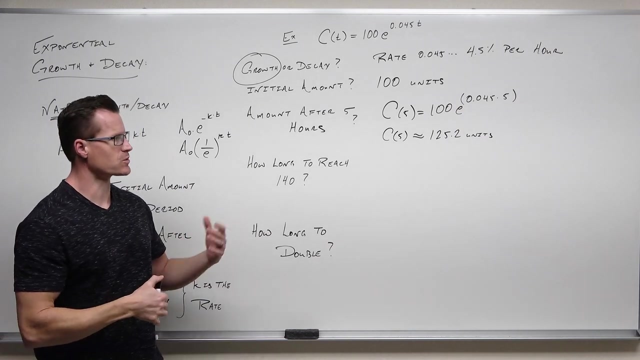 So on our calculator we'll put 100 second LN and then we'll have our parentheses of 0.045 times five. I get about 125.2 units. whatever that is, If it's grams it would be 125.2 grams, or. 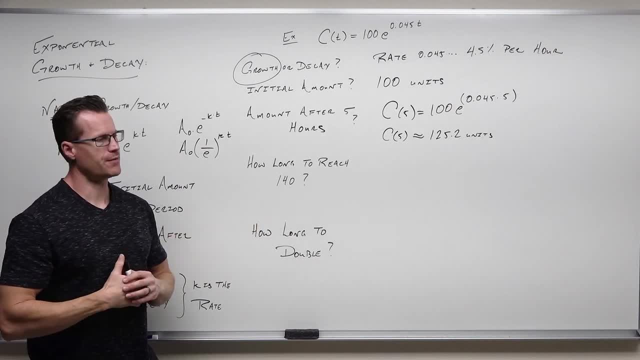 sometimes we do call it units of bacteria. We would get that many after five hours. I hope that makes sense. I hope you're seeing that this is very much like compound interest. What about a different question? What about how long would it take to reach 140 units? 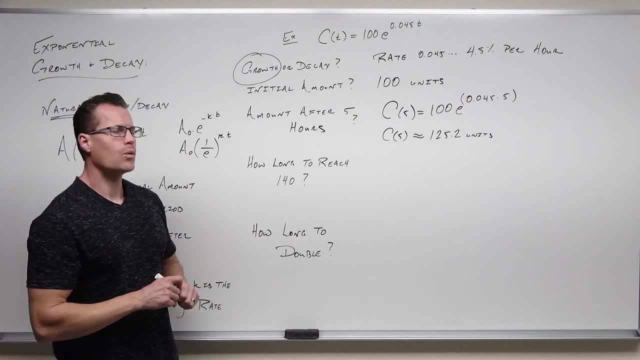 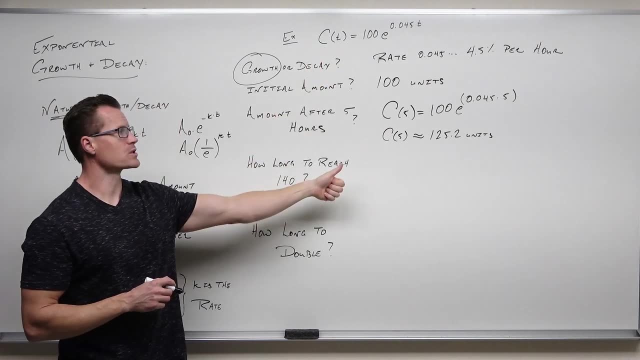 or 140, whatever, these are 40. these are: Well, that's different, isn't it? That's saying, if you start with 100, well, that's a given. That's there for us. This is our formula. How long is it going to take to? 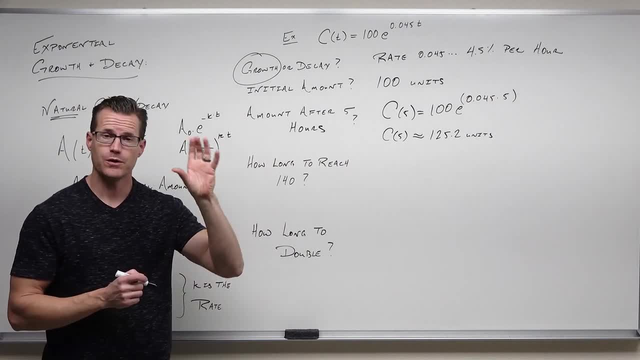 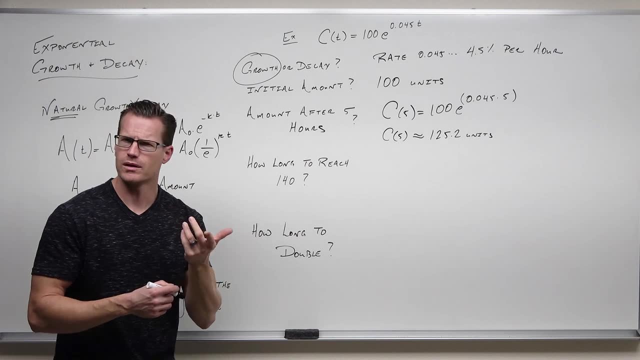 reach 140? Well, 140 is a future value of this population size. Let's make it that. Let's consider this to be what it would be in the future. Well, how long is the future? Well, that's what we're trying to find out. We're trying to figure out the T. How many hours would it take? 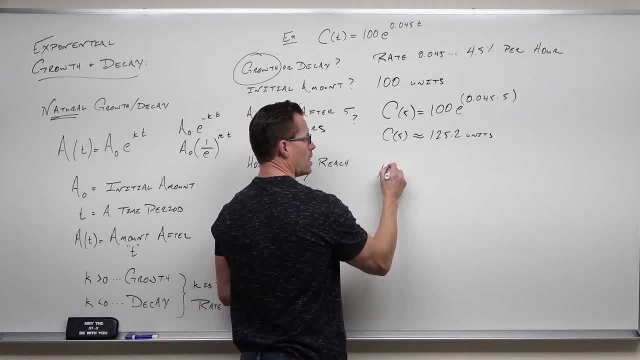 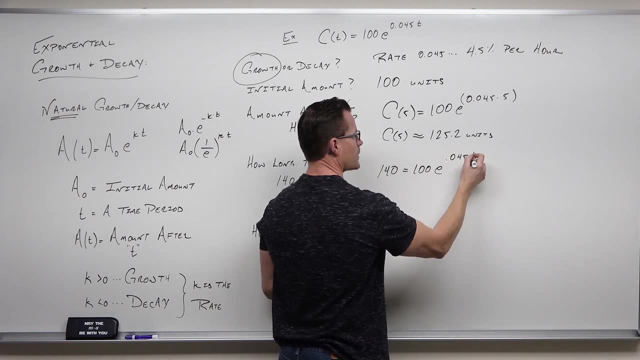 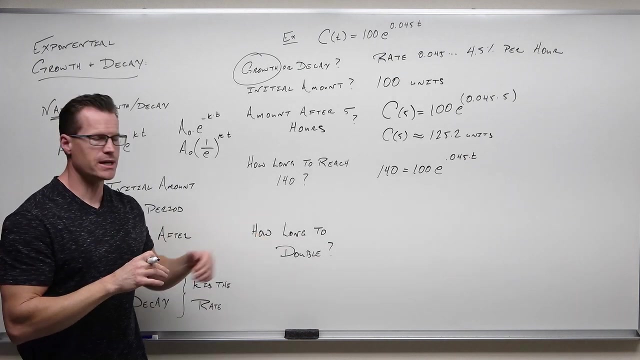 to reach that. So we're going to take a formula and say I want it to be 140. But I don't know what the T is. I hope that this looks a lot like doubling an investment, because we're going to do that next, But in this case we're not doubling it, We're just reaching a. 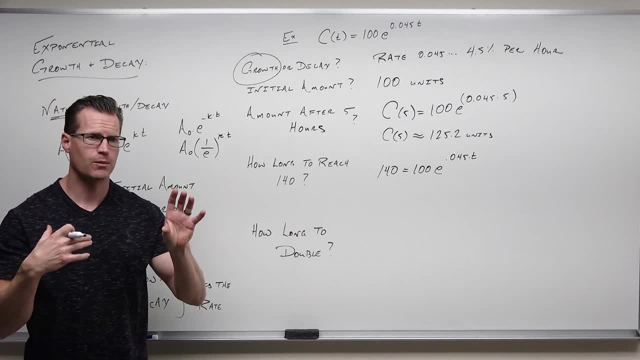 goal. We're saying we're starting with 100.. How long is it going to take to reach 140? 140 would be the idea of that's going to be a value in the future. Let's solve for the T In your head, right? 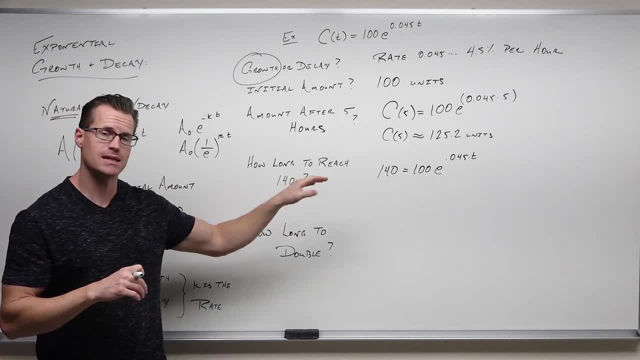 now you should be thinking: well, I want to reach 140.. I want to reach 140.. I want to reach 140.. I'm going to be using a logarithm. at some point I have to, because that's an exponential equation. 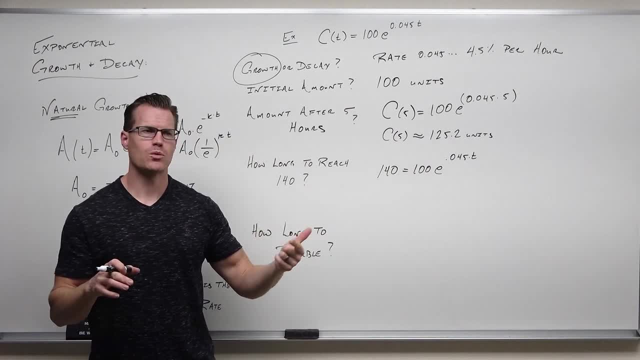 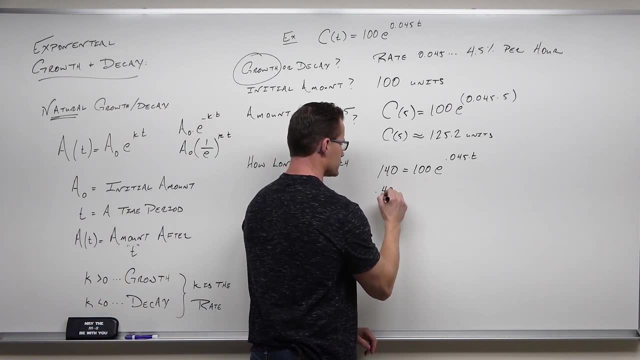 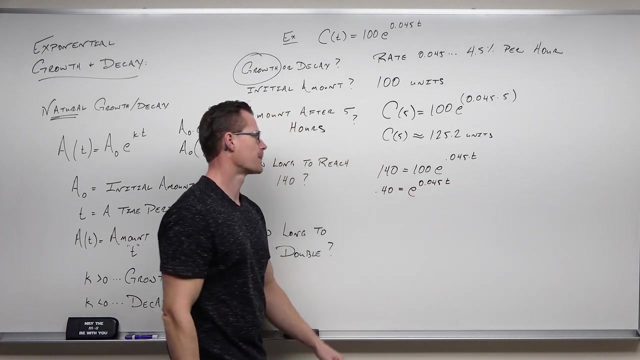 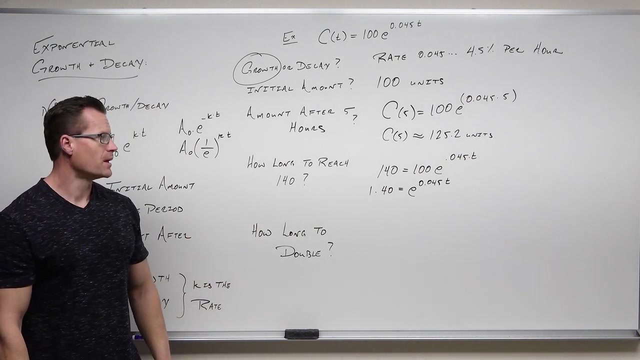 I'm solving for T. That's a must. But before we do that, before we're able to use logarithms, you must isolate the exponential. So we're going to divide by 100. So dividing by 100, 140 divided by 100 is 1.4.. Now we have an exponential equation. 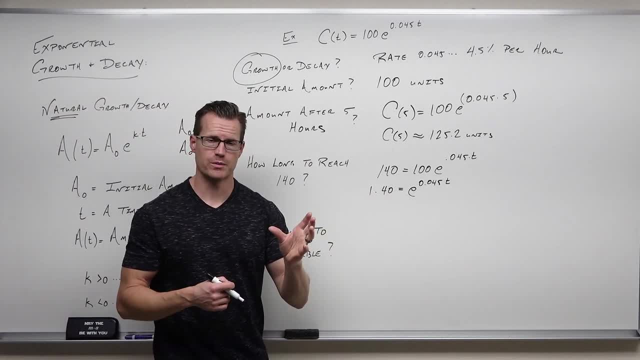 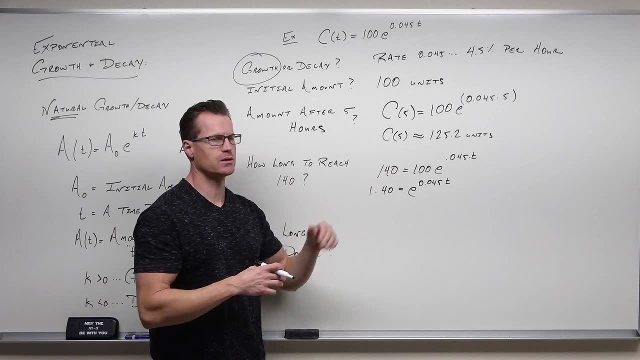 It doesn't matter if it's a decimal or not. We're going to do a logarithm of both sides For this. just like always, use ln. Please use ln, especially when we're dealing with exponential growth and decay, because you're going to get a lot of simplification. 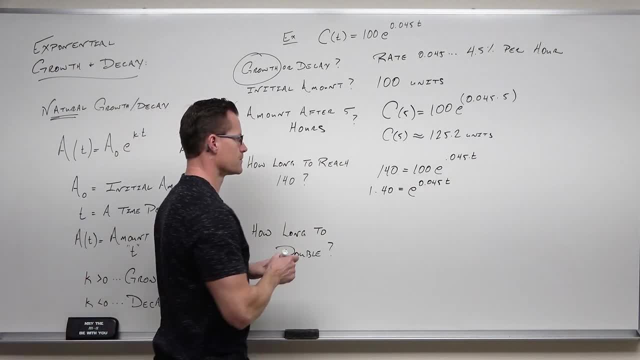 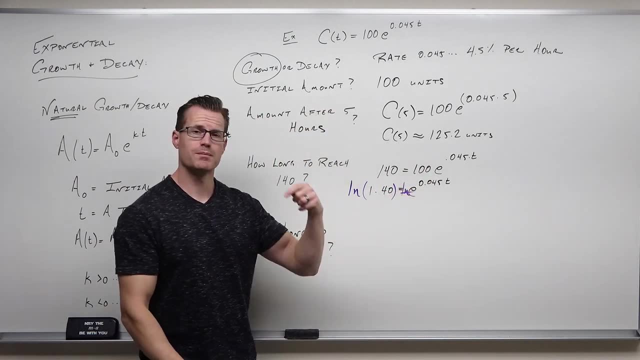 So we're going to take a natural log of both sides And, because we match up our bases, we compose an exponential onto a logarithm of the same base. This is going to simplify. We get ln of 1.5.. 1.40. 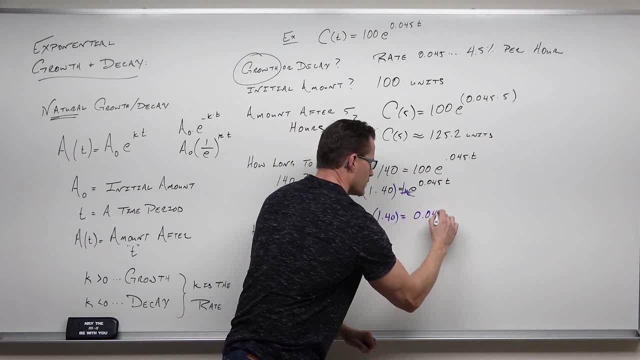 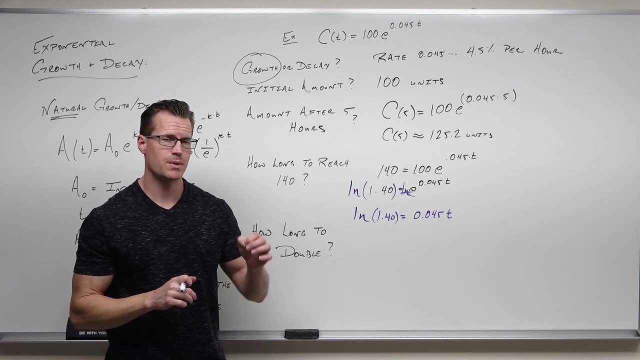 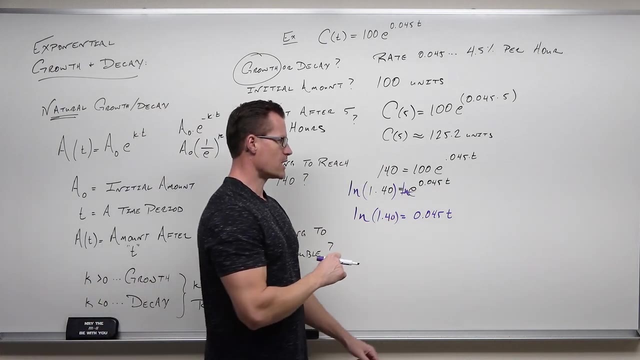 equals 0.045T, Just like doubling your compound interest when it was continuously compounded in the last video. we're doing the same thing, It's just that we're not doubling. We're reaching a different goal If we divide both sides by 0.045,. 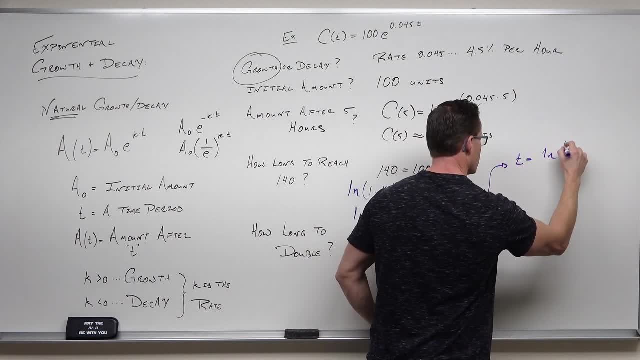 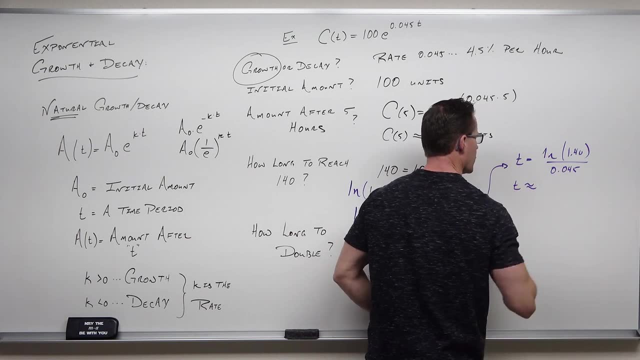 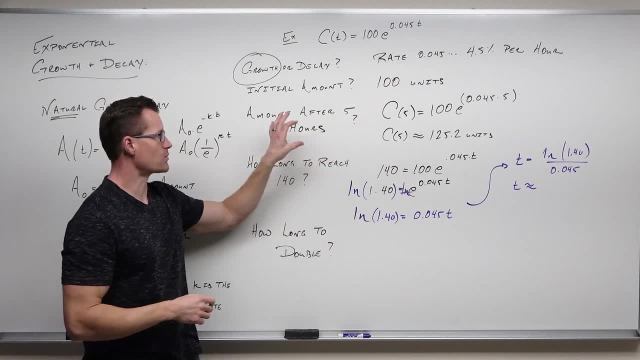 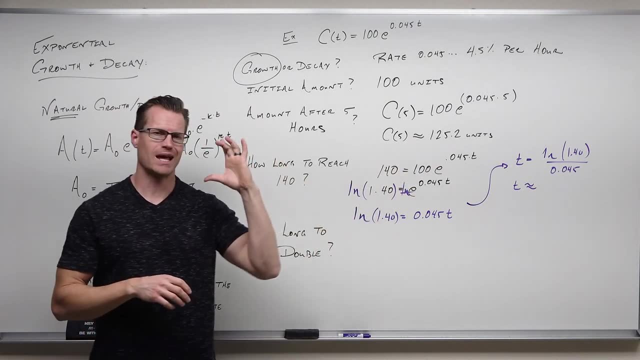 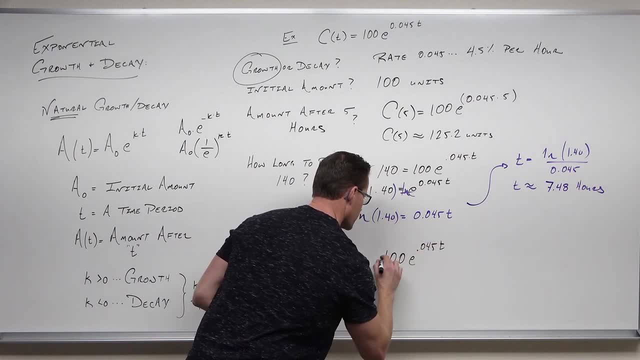 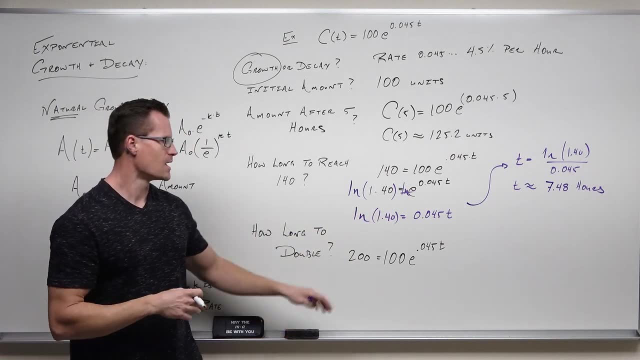 0.050, 0.050, 0.065, 0.050, 0.055, 0.056, 0.076, 0.077, 0.0 și 05, 0.011 0.0ście 0.024. 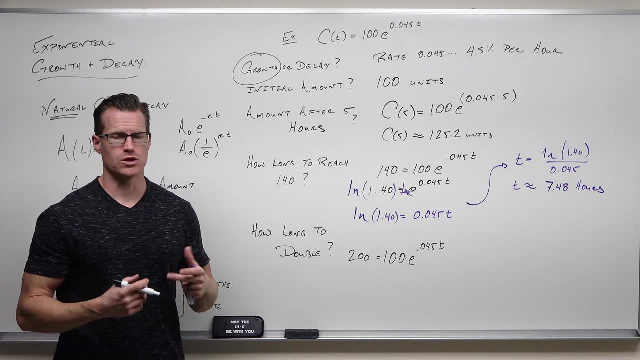 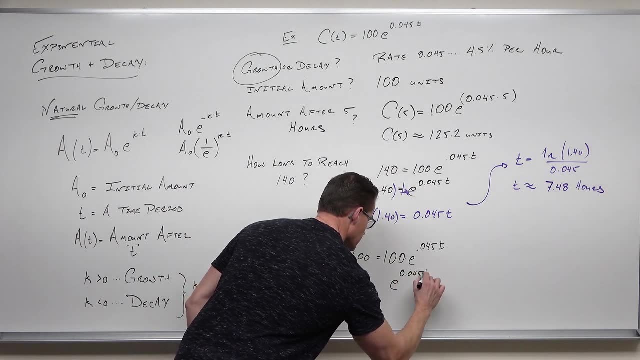 0.2, 0.035, 0.1, 0.6, 0.8, 0.4. So 2 equals e to the point 0,, 4,, 5, t. That is an exponential. There's no common bases. 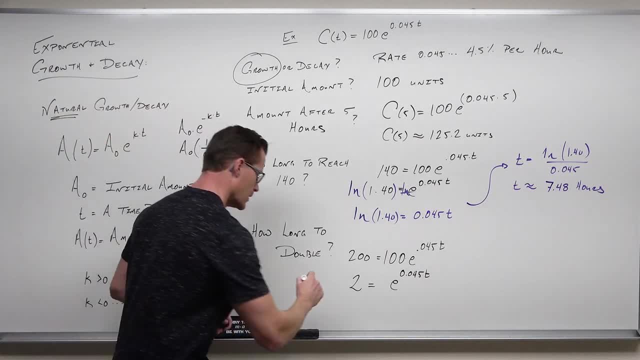 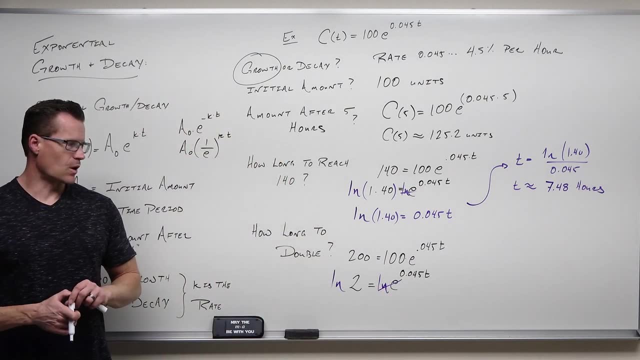 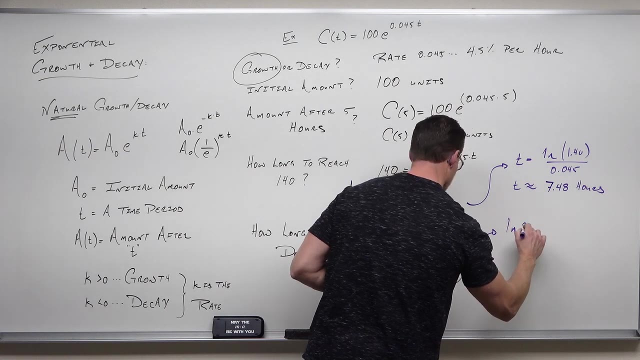 We have to use a logarithm and in general we just use ln almost all the time. This naturally composes your base of your logarithm with the base of an exponential, a function, with its inverse cancels. We get ln. 2 equals that point, 0,, 4,, 5, t. 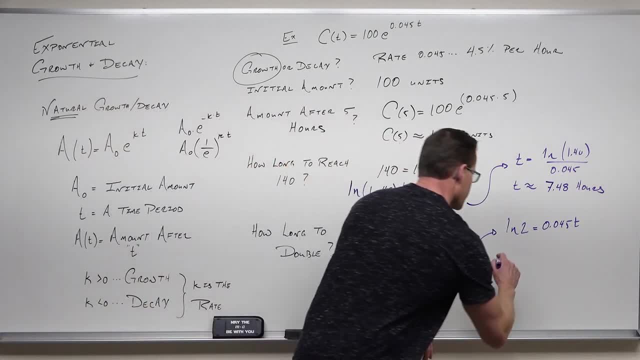 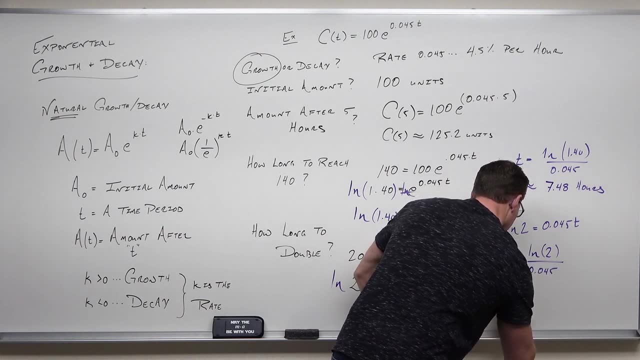 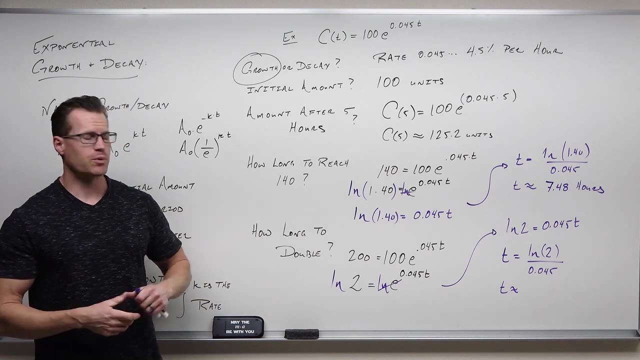 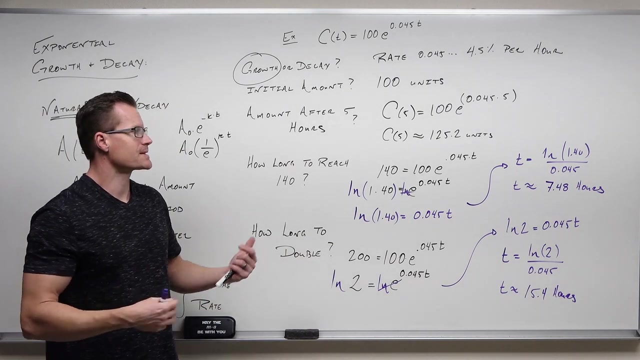 We're going to divide both sides by point: 0,, 4, 5.. We have parentheses after the ln 2.. It's really important for your calculator and it should be a bit more than 7.5. So I got 15.4 hours and that makes sense. 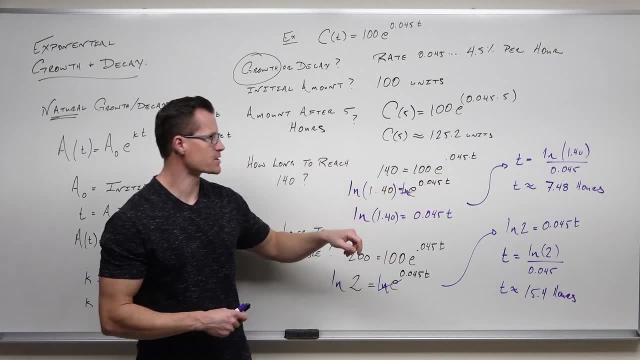 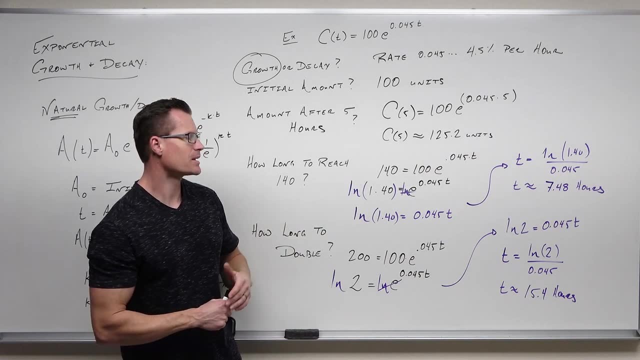 To gain 40 units costs us 7.5 hours. To gain 60 more units on top of that would be an additional almost double, Well a little over double that, but we're gaining 60 additional units. So 100 to 140 was 7.5 hours. 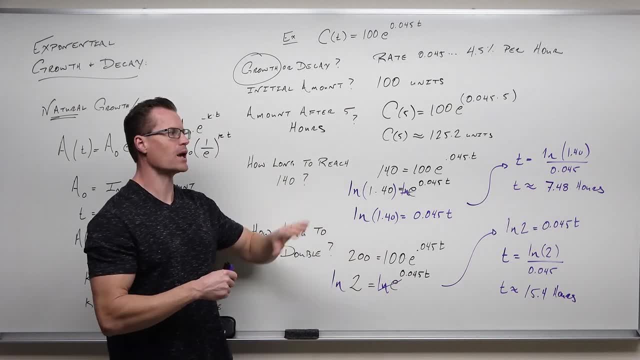 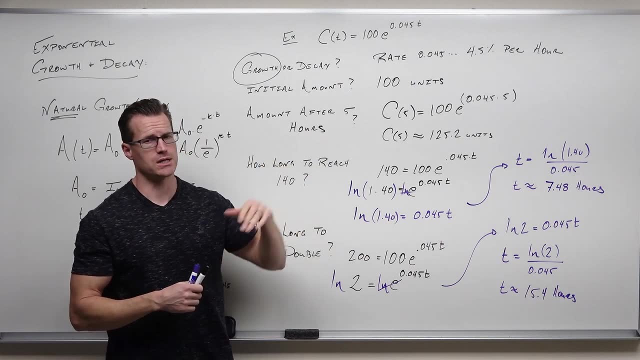 100 to 200 was 15.4, so it makes sense. It's not way, way out there like 100 hours or something. Remember this should be gaining faster and faster. It is positively increasing exponential growth. I hope it makes sense. 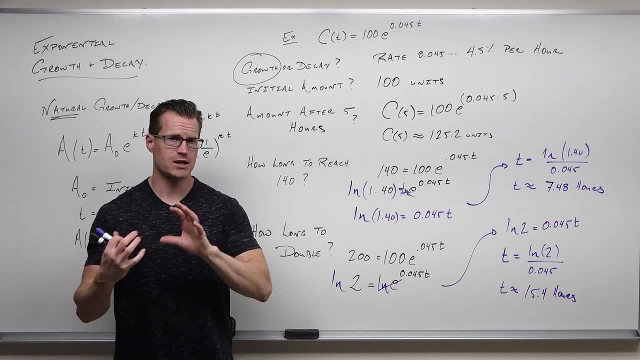 I hope you're seeing all the interplay between this and I hope I'm really making the connection between exponentials, this stuff and the finance that we just did. I'll come back with another one that we're going to start from scratch. 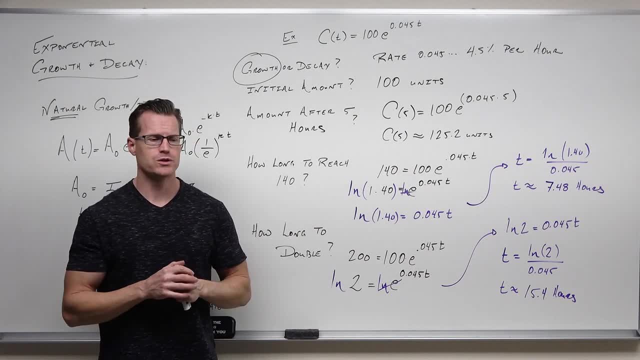 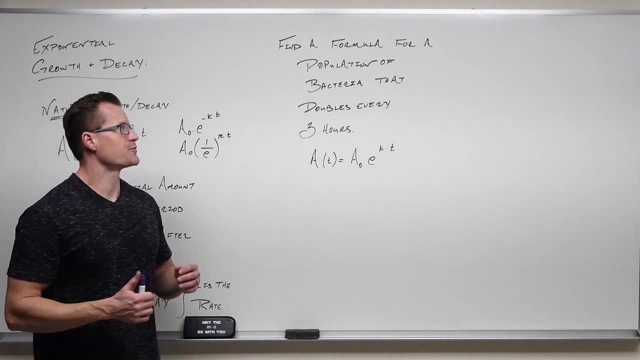 and create a formula that models exponential growth, Then we'll do a half-life for decay and Newton's law of cooling. All right, we're ready for another problem. Let's give it a try. We're supposed to find a formula for a population of bacteria. 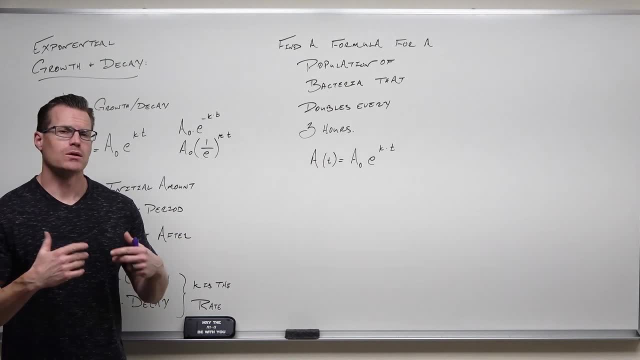 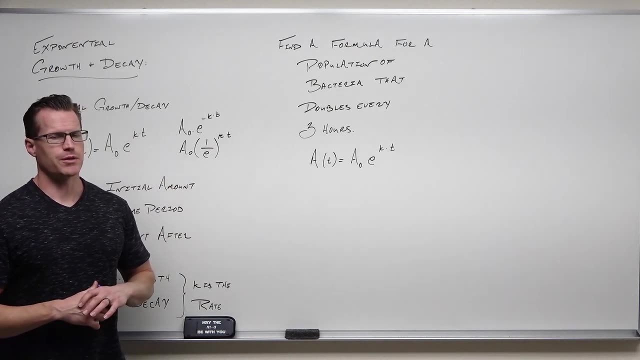 that doubles every three hours. So let's take a look at this formula. Let's take a look at this and model this with an exponential growth formula. In order to do it, we just have to understand a couple things about the process here. 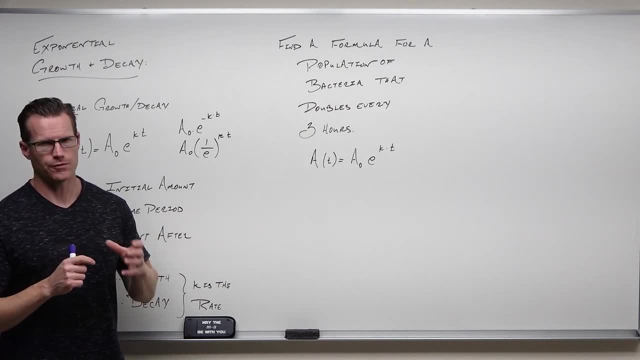 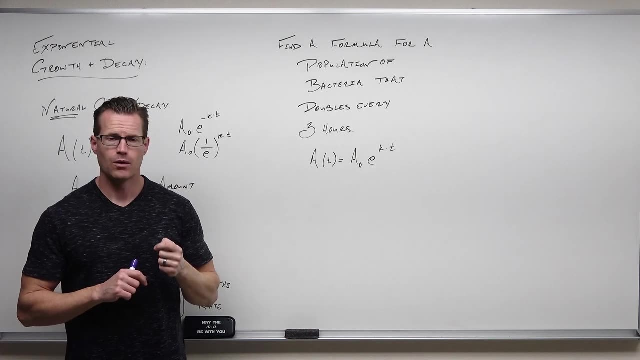 What's going to happen is we have to find our rate first, So it's going to give you enough information to plug in everything and solve for your K. That is your first thing to do. Once you've found your K, you can ask any other question that you want on this thing. 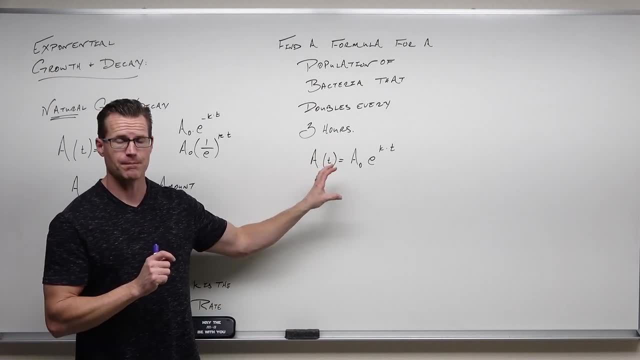 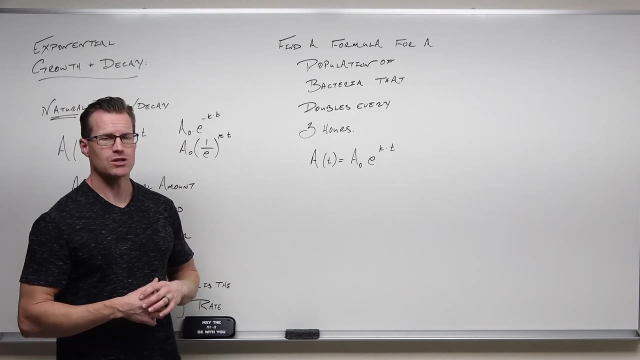 So it's all about finding the K first and then plugging that back in. Then you answer the question. So let's take a look at it. We've got a formula for population bacteria that doubles every three hours. There's a lot of information there. 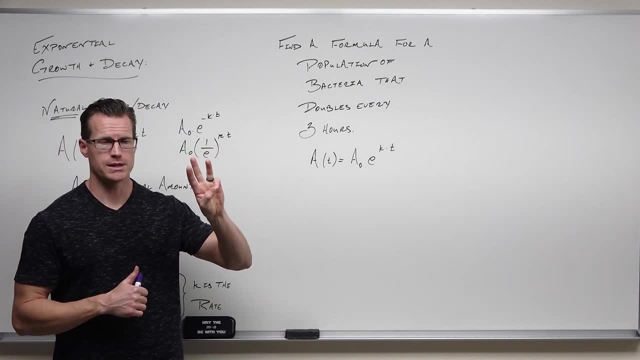 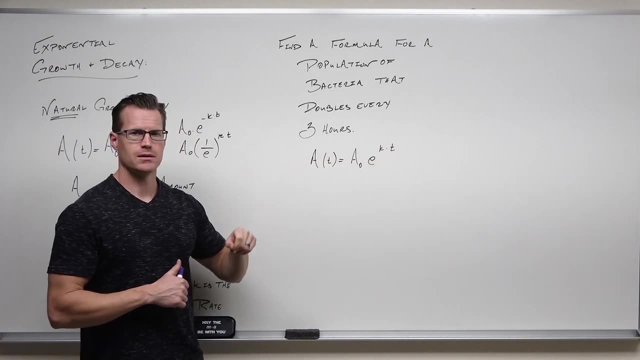 Number one. it's saying there's a time period, We have three hours, So we're in a time unit of hours and saying after three hours we're going to put a three here. this should be two times that. Now, what is that? 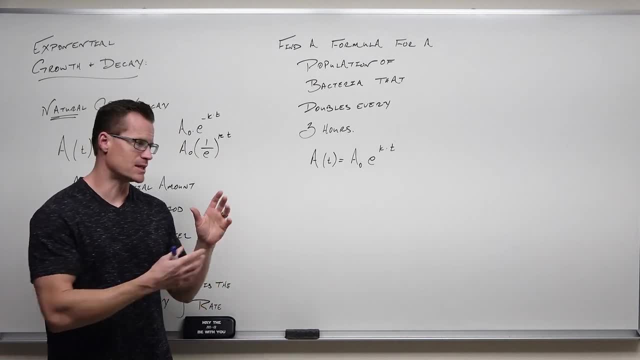 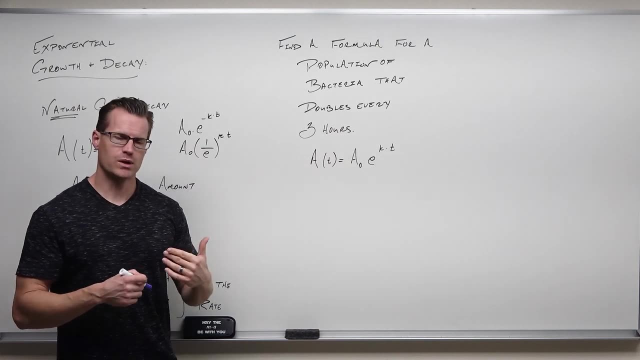 Who cares? It doesn't matter. We dealt with this in doubling investment and doubling bacteria. It doesn't matter where we start. If we start at one, this would be two, Start at 100, this would be 200. It doesn't matter. 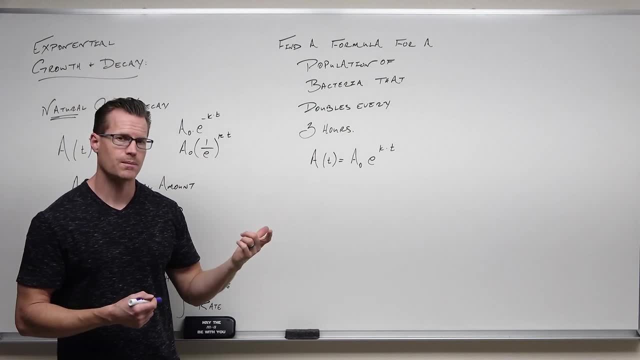 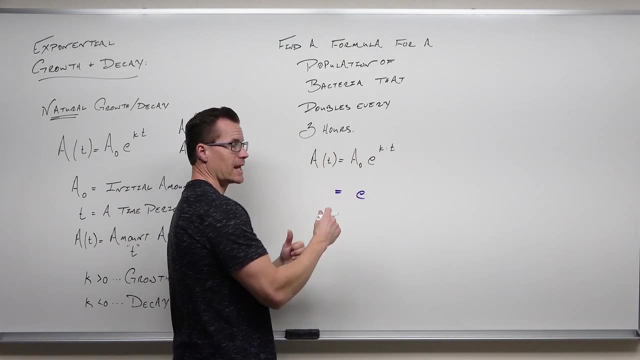 And it also doesn't matter because we divide in the very first step to try to solve for our K. So let's plug in a few things. We know that we're trying to solve for K. It's not telling us the rate. We need to understand that. 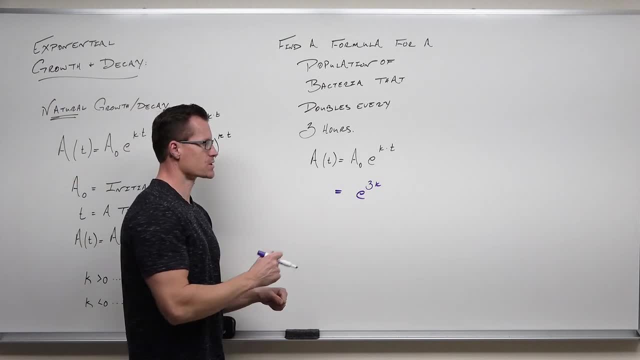 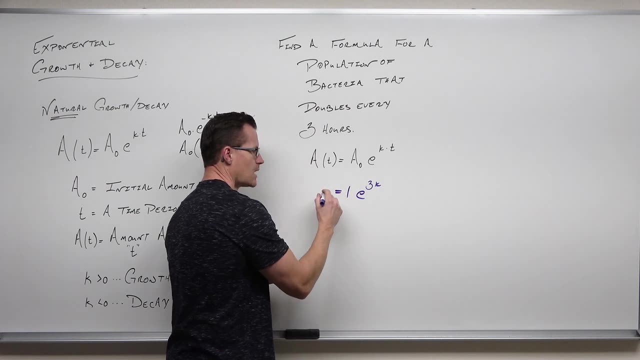 But it's telling us, after three hours- that's our three hours- this future value or the population will attain this amount. that's double what our initial amount was. If that's one, that's two. If that's 10,, that's 20.. 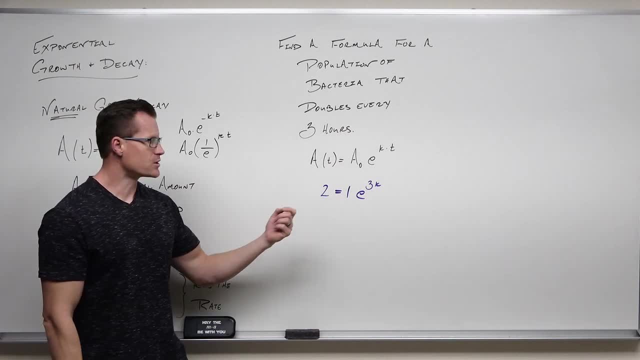 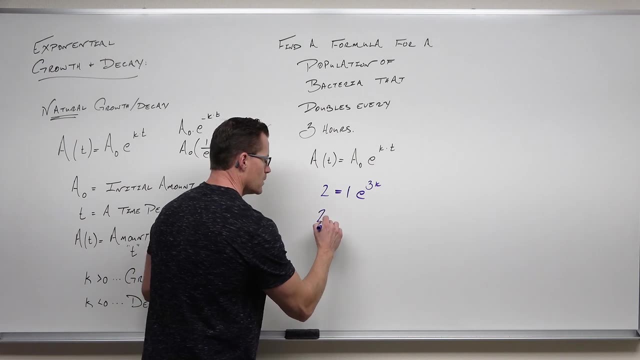 If that's 100, that's 200.. The very first thing we would do is try to solve for K by dividing the isolated exponential. We divide both sides, But whatever the initial amount is you're going to get. 2 equals e to the 3K. 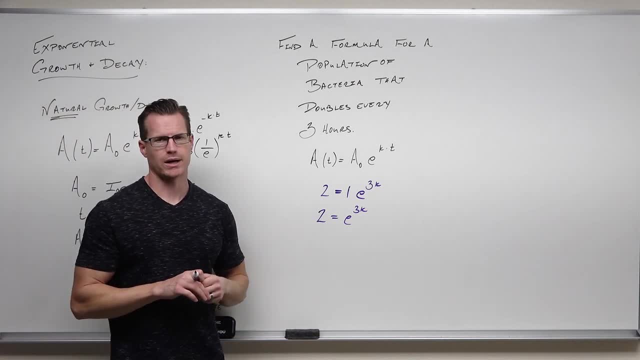 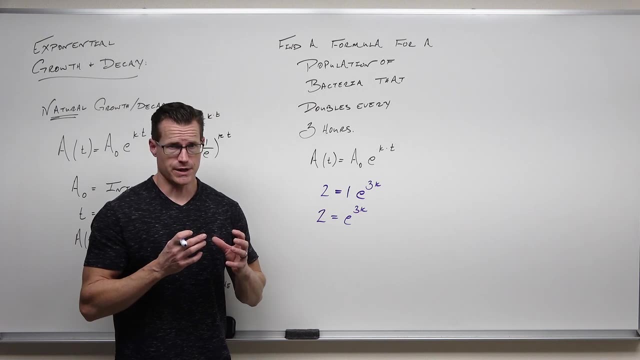 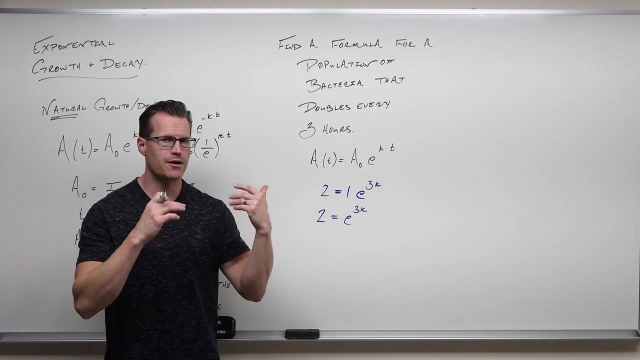 This is what doubling looks like all the time once you have isolated your exponential. A couple other things about this that I would like to mention. You can see a few different things. They could say something like: hey, your population of bacteria is growing at a rate of 5.2% per hour. 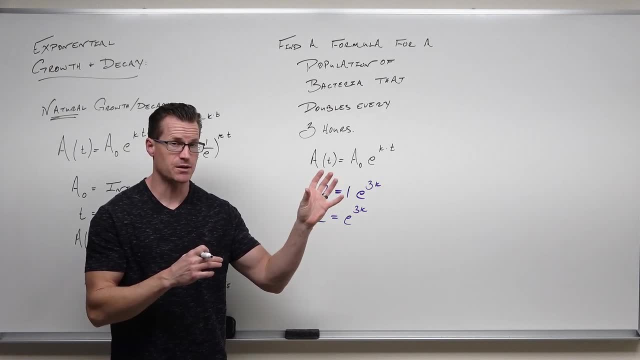 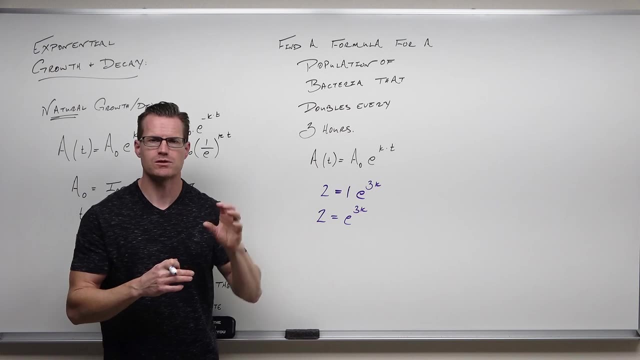 If they tell you that 5.2% per hour, well then that's a K of .052.. You can always find that That is your rate. So if they're telling you the rate, you don't need to do any of this. 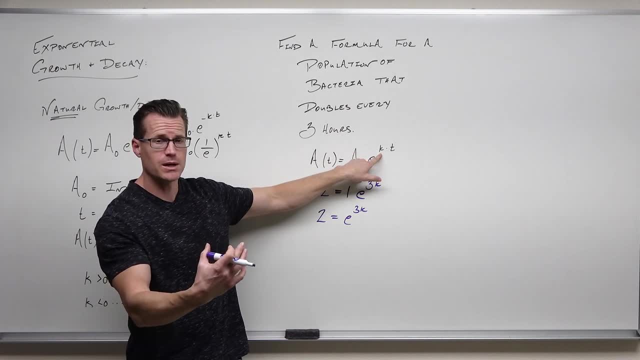 You just say, hey, that rate would be whatever percentage you're telling me as a decimal. You can always do that. The other thing I can tell you is: instead of doubling- I just want to make sure that that's fresh in your head. 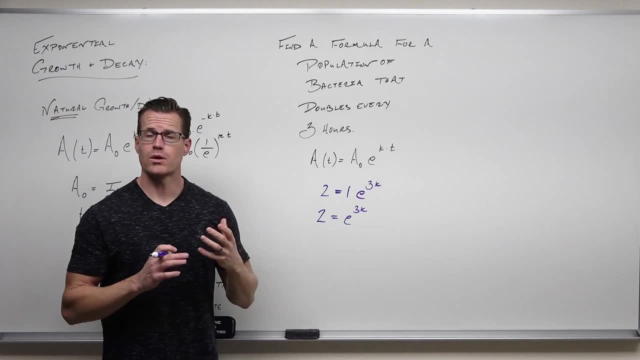 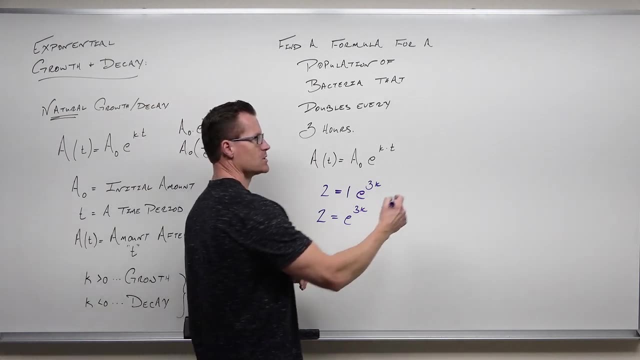 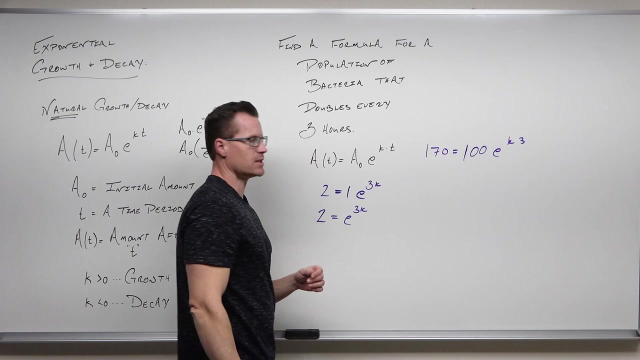 I could say a population of bacteria started with 100 units. After 3 hours it had 170 units or something, And so in that case you'd say I started with 100.. After 3 hours I had 170. 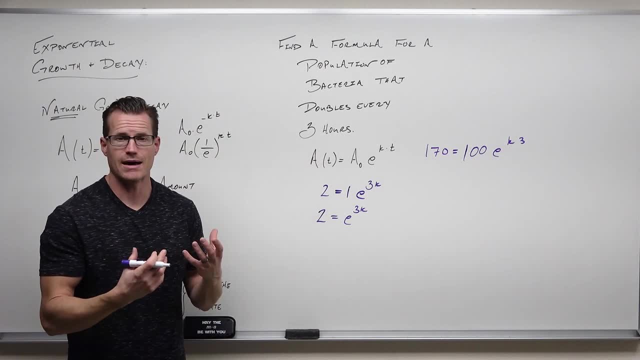 It's the same exact thing. I'm just telling you a double, because students tend to have a harder time with a double. If I say you start with 100 and after 3 hours you have 170.. Sure, you can divide by 100.. 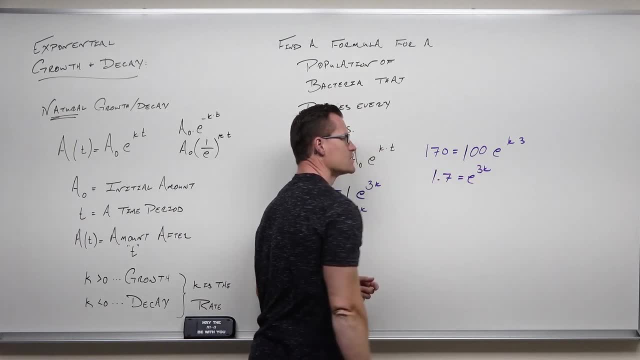 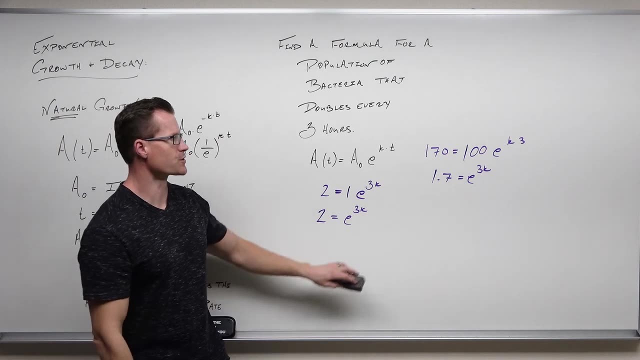 We saw this in the first example And it gives you something very, very doable, very similar to this. It's just a different way to look at it. If you wanted to see the first way right now, if I told you that the increase was 5.2%, 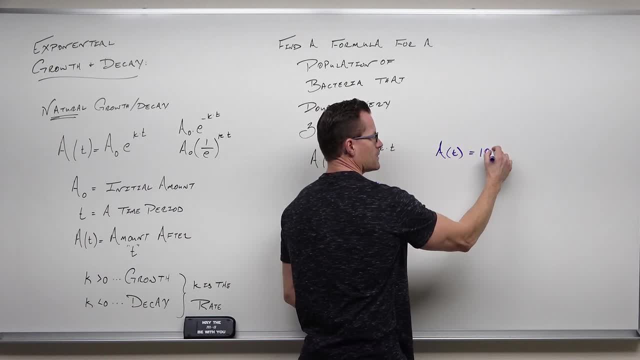 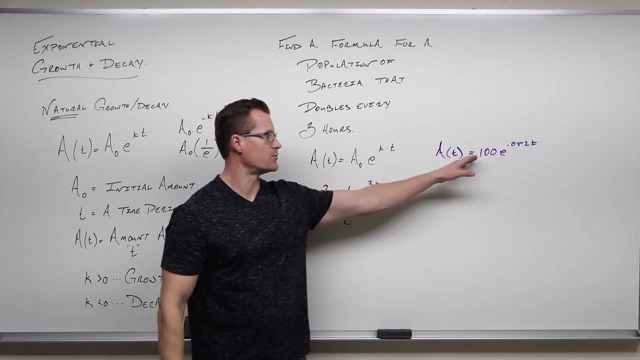 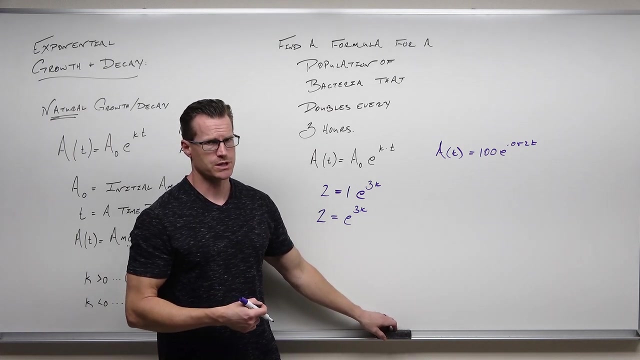 and they said: you start with 100 units and your rate of increase is 5.2%, then you are done. There's your initial value and there's your rate of increase. It said rate of decrease. Well then you would have negative 0.052%. 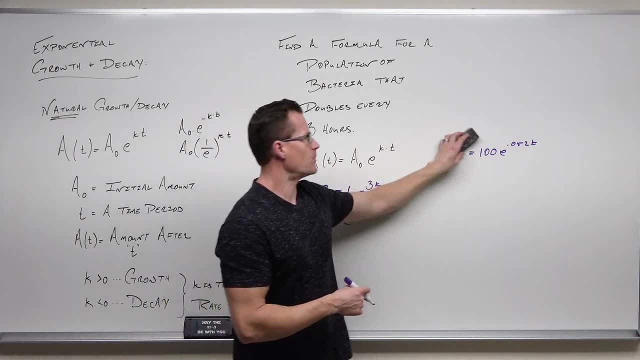 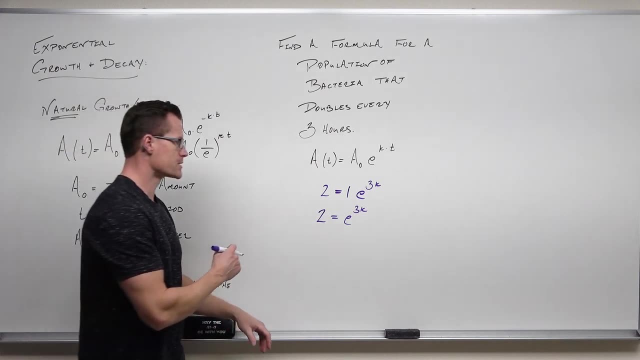 So there are other ways to look at it. I'm giving you the most common, though. All right, So we're down to here. We've got to solve for our k. We need to take an extra log on both sides, So we're going to do that. 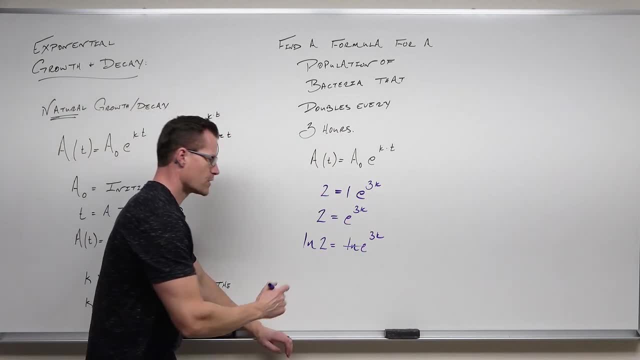 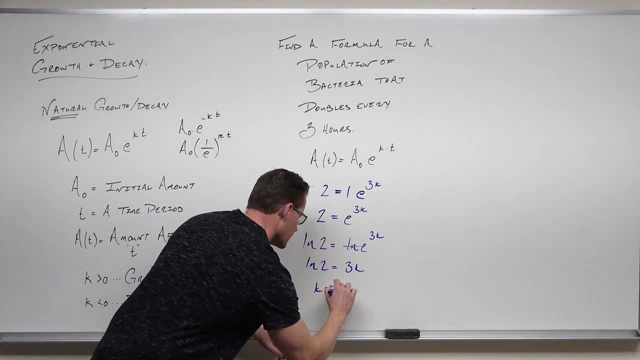 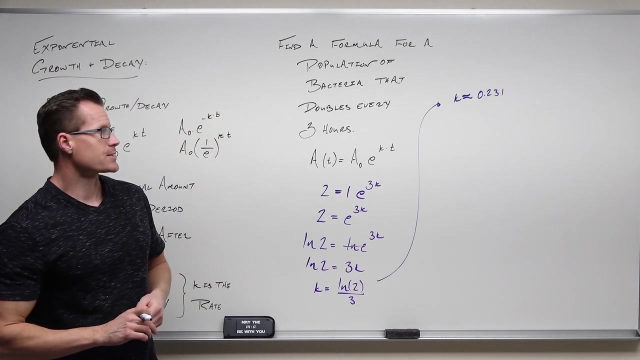 Because our bases match on our function and the inverse of the function. we end up getting ln2.. So k equals 3k divided by 3.. We get k equals ln2 over 3.. So I got k is around 0.231.. 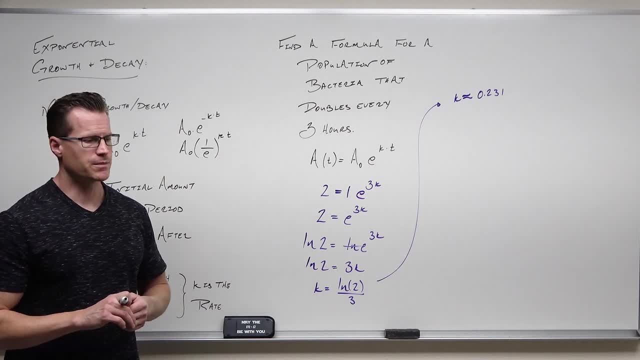 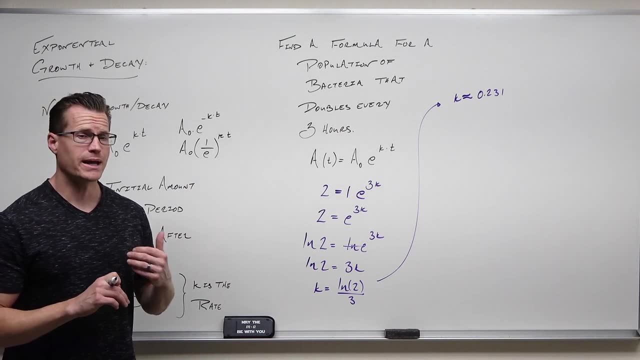 Now I'm going to encourage you to not round that number. very often Those can be very, very, very small numbers, very close to 0. And if we end up rounding them a lot, that's a problem. You might actually choose to leave it. ln2 over 3. 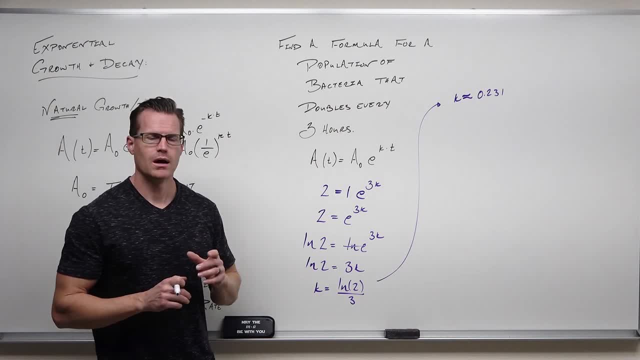 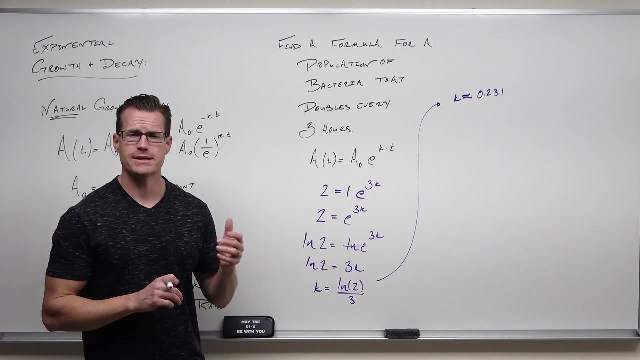 and just put that here. It looks a little awkward. I'm not doing that because I want to show you the rate. The rate of increase here is 23.1%. 0.231 is 23.1% per hour. That is how fast this colony of bacteria is actually growing. 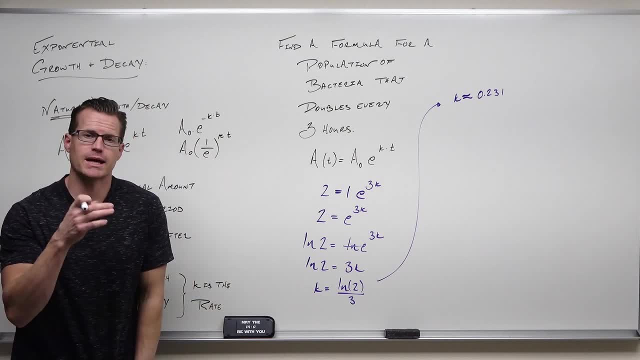 So what does that mean for us? Now that we have our k and our k is a constant, It's like the rate in finance: Your rate doesn't change every day. I mean it can, but if it's a fixed rate, 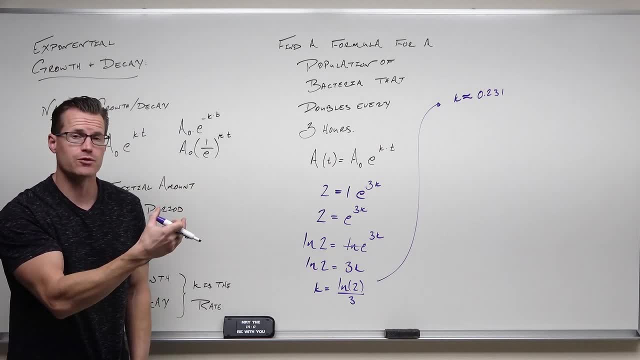 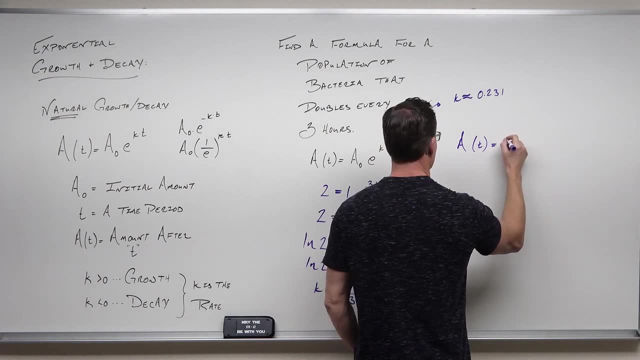 it's going to stay the same all the time. We're assuming this is a fixed rate of growth for this. So what does that mean for us? Well, we can see with that k that that is positive. That should be exponential growth. 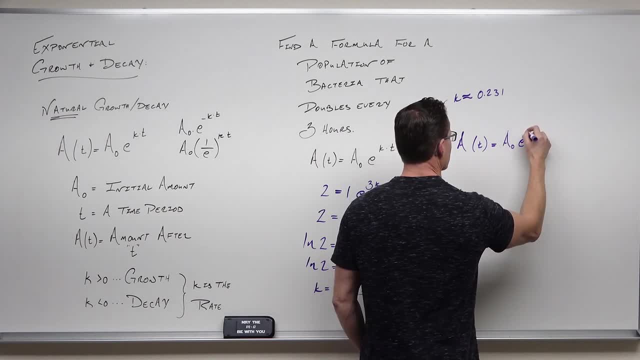 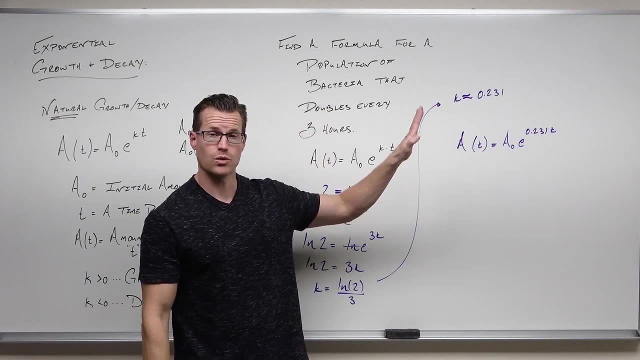 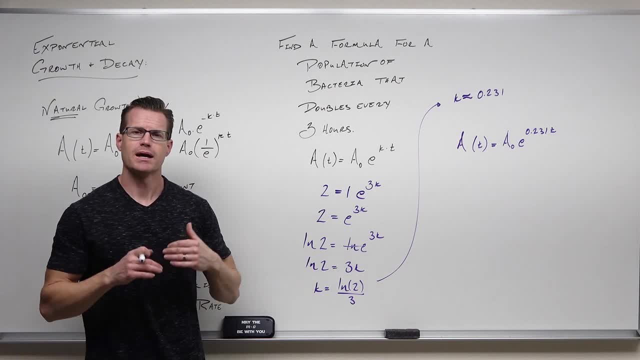 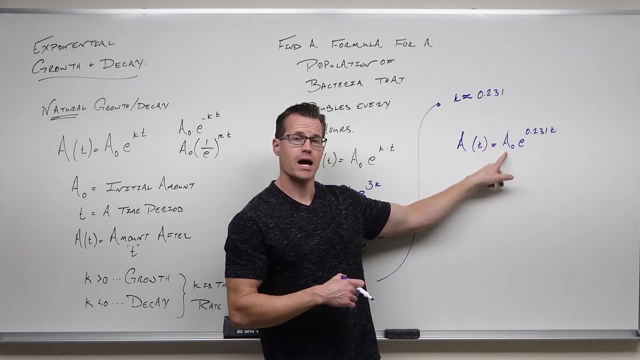 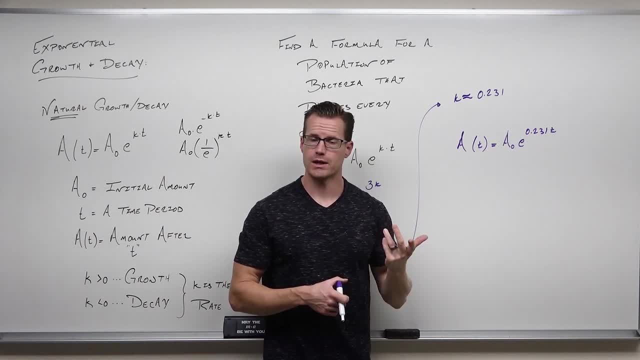 We put 50 here and 10 there. I said: how long would it take to triple this colony of bacteria? Then I put 1 here and Yeah, let's go ahead and do that one. How long would it take to triple this? 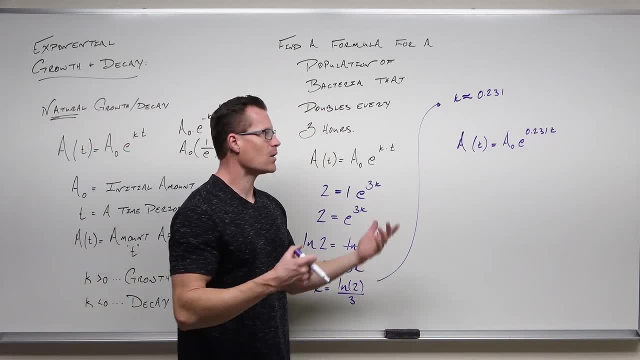 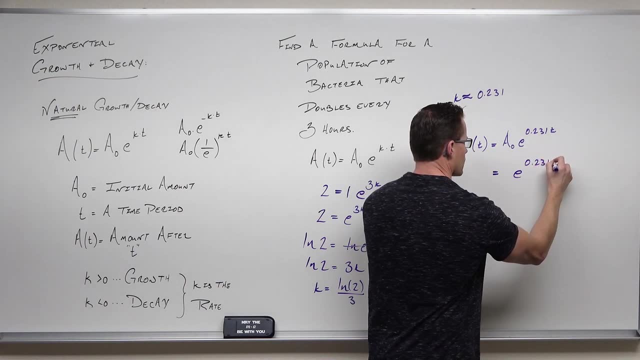 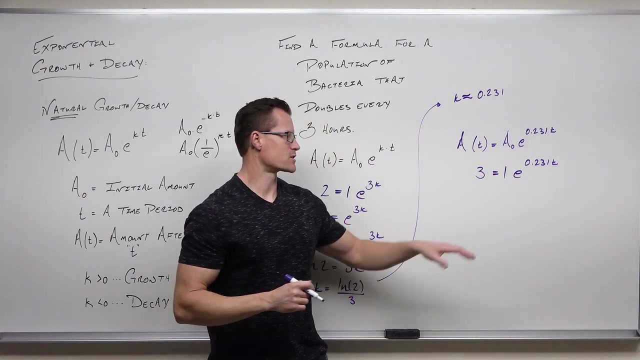 Better be more than 3 hours, right, Because 3 hours is how long it took to double it. But how long would it take to triple this? How long? ask for a time. Triple says if you start with 1,, 1, you'll get 3.. That would be triple. I start with 100, I get 300.. Your first order of business. 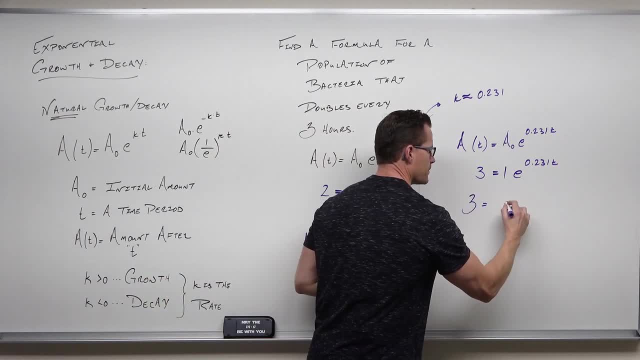 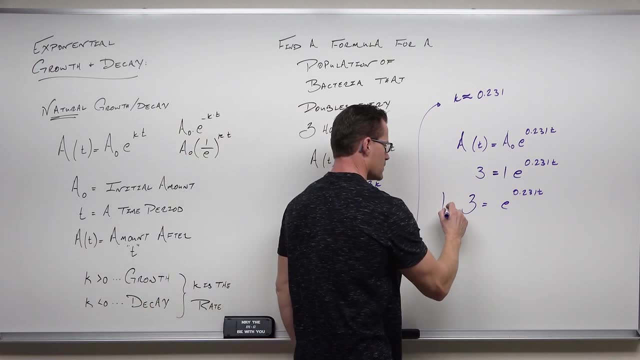 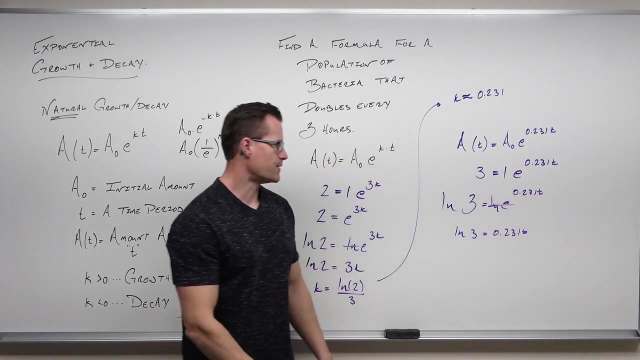 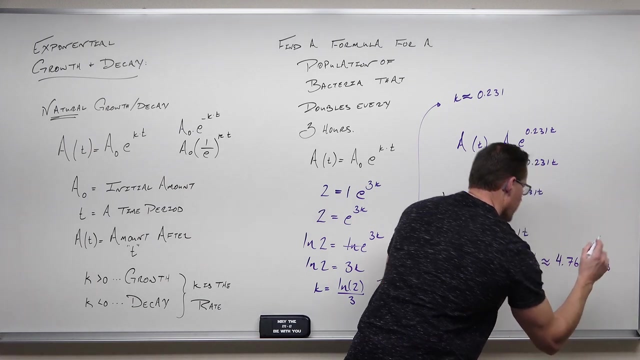 would be to divide. So we're going to end up getting 3 equals 0.231T. If we do an LN on both sides and we divide by 0.231, we get about 4.76 hours. I hope that makes sense. I hope that if it, 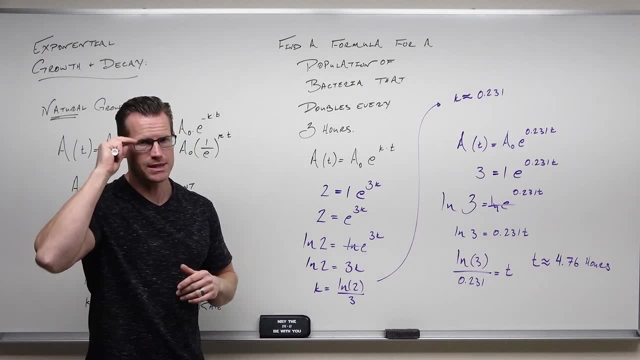 doubles in 3 hours, it should triple in 4.76 hours. That should make sense in your head that it's more than 3.. It's not way, way out there, but it's definitely positive in more than 3.. 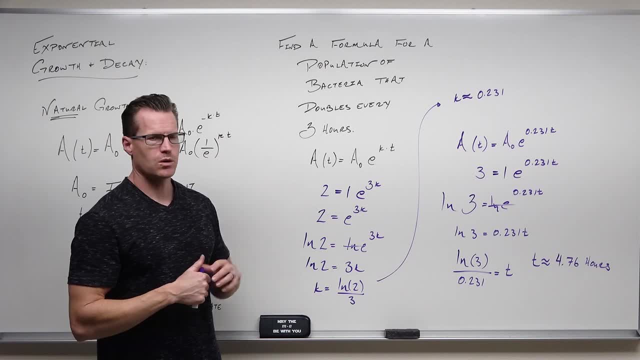 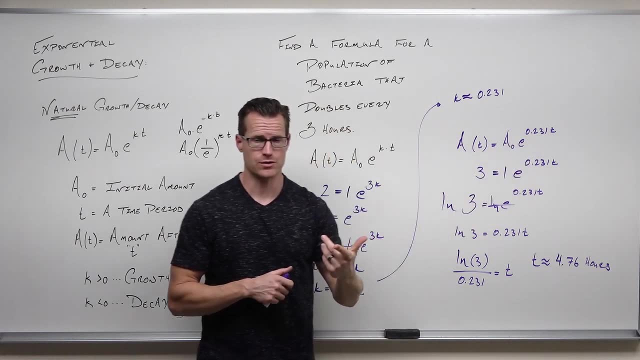 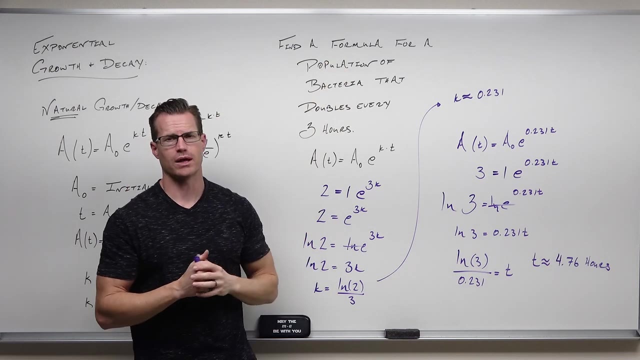 Again, if I had said: suppose you start with 50 units, how much would you have in 10 hours? You could certainly put a 50 here and a 10 there and figure that out as well. This is just designed to give you an understanding of how exponential growth and decay work. from an original question. 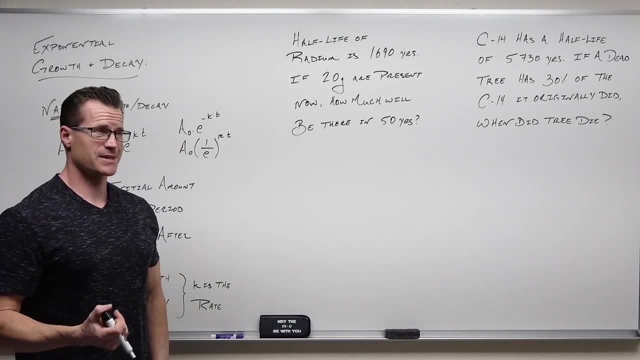 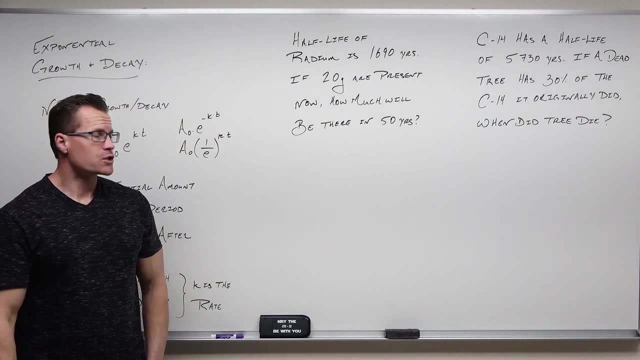 like that one. I decided to do two examples because they're slightly different and I know I would get questions on that one, So I'm going to put it up there to make sure that we understand the differences between them. So we're going to talk about exponential growth and decay. 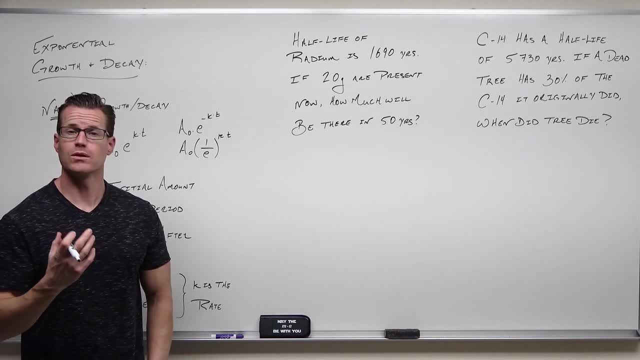 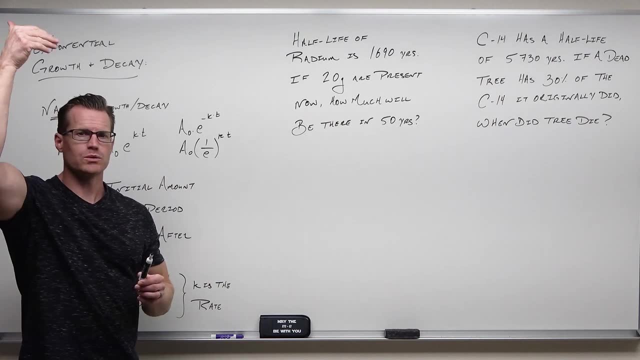 Right now, half-life, is a really good way to look at this, because if you think about something that's radioactive, something that's constantly losing stuff, it's going to lose a lot of stuff at first because there's a lot of it to lose, But as we get closer and closer to having none of it. it's going to still lose at the same rate, but there's less to lose. Will you lose everything? Not according to exponential decay. You have a horizontal asymptote, don't you? So can you ever lose all of a substance? theoretically, 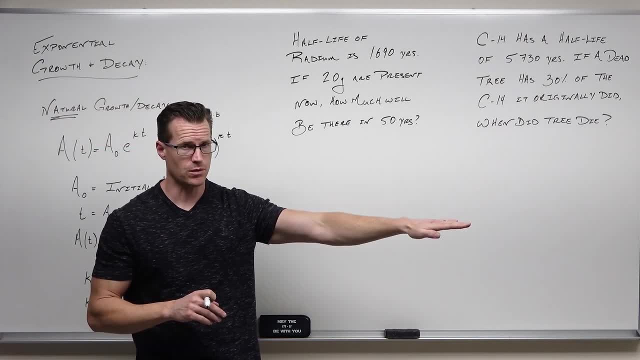 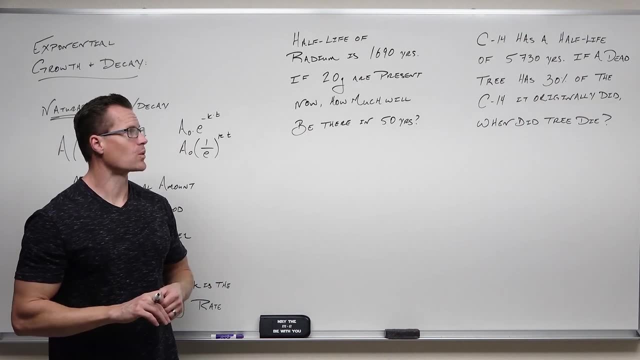 No, You'll get closer and closer to zero, but you'll never lose all of it, So there'll always be some left, And that's a decent way for us to date certain items. So how in the world do we do these things? The same exact way as the last example, but we're going to get exponential decay. 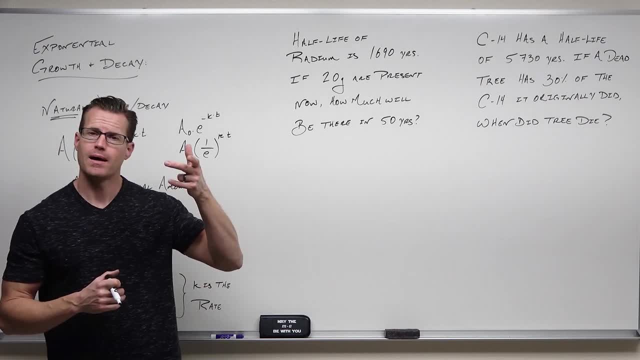 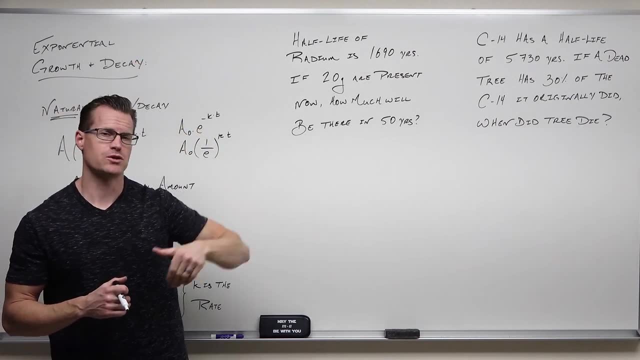 because we'll have a negative exponent And that would create, if we use that negative to reciprocate, a fraction, a base less than one, giving us a decreasing exponential graph. That's what's going to happen. So let's take a look at it. 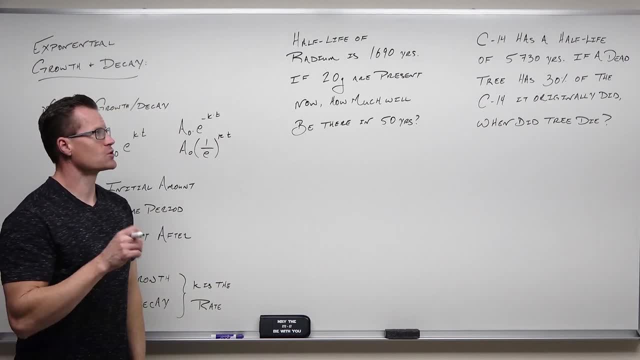 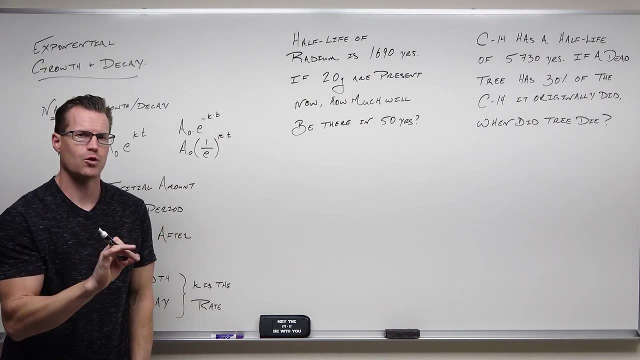 The half-life of radium is 1,690 years. If 20 grams are present now, how much will there be there in 50 years? For all of these examples where you have to make your own formula, your primary goal is to find K first. So let's start with our function. 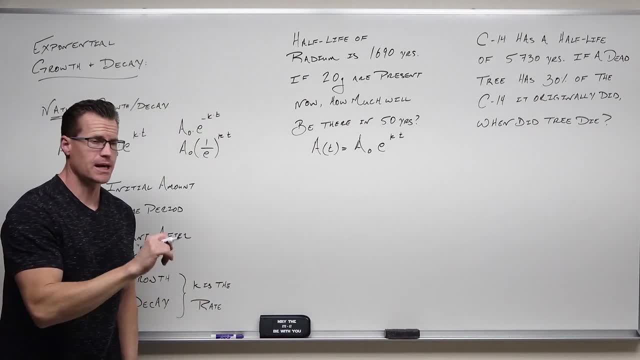 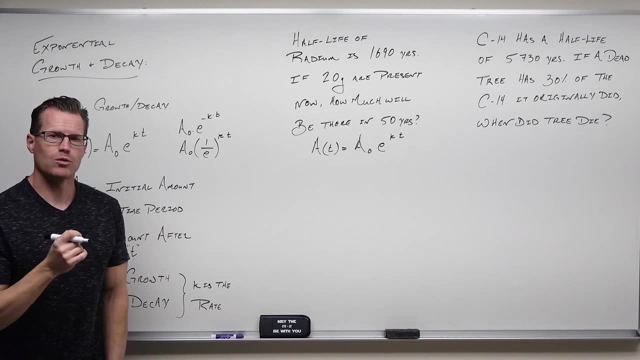 We're thinking half-life means declining. Our K should be negative, so that's important. Now, half-life: here's what that means. if you're not familiar with it, What half-life means is there will be half of whatever you start with after a certain amount of time. For radium: 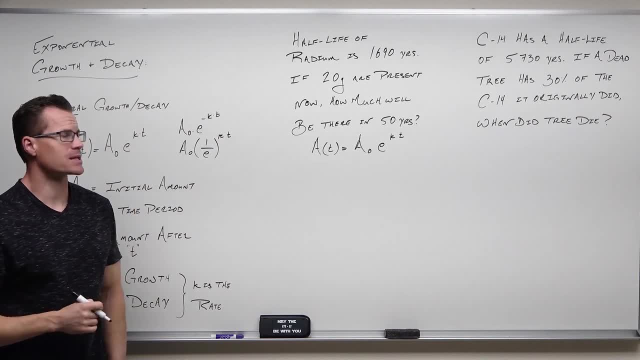 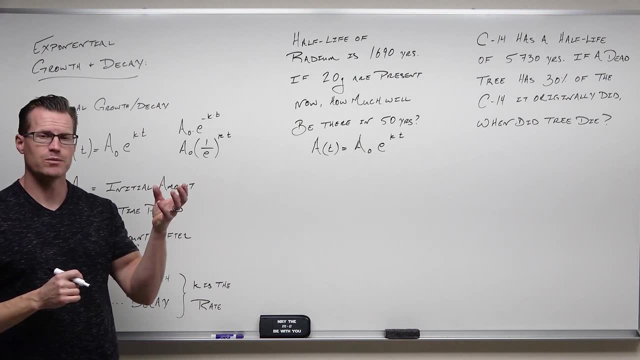 that there will be half of it after a certain amount of time. that time is 1,690 years. So if you started with 100 grams of radium after 1,690 years, there would be 50 of it left. The. 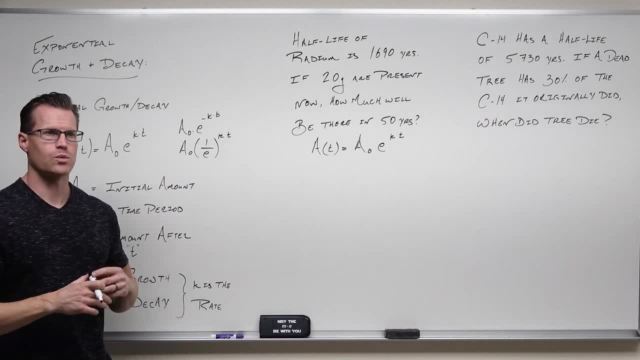 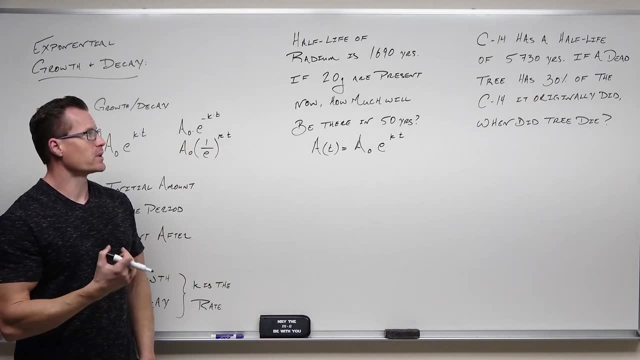 other 50 will have radiated away. and that's what radiation does These particles emanate? uh, from whatever substance that is, that's radioactive. So the half-life of radium is 1,690 years, but that gives us something, doesn't it? It says: if you have 20 grams now 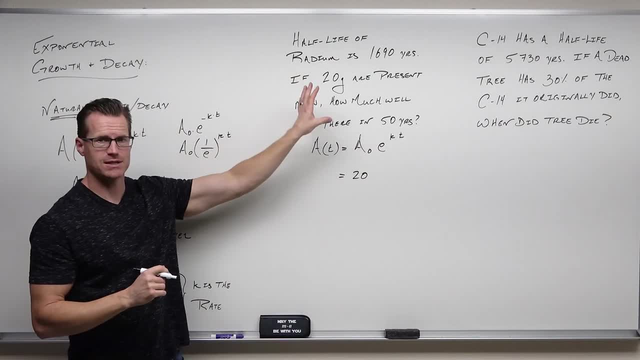 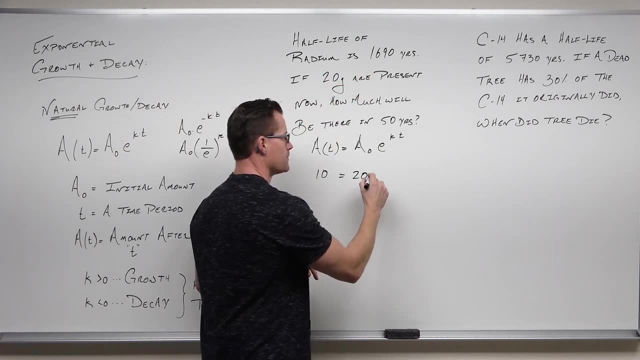 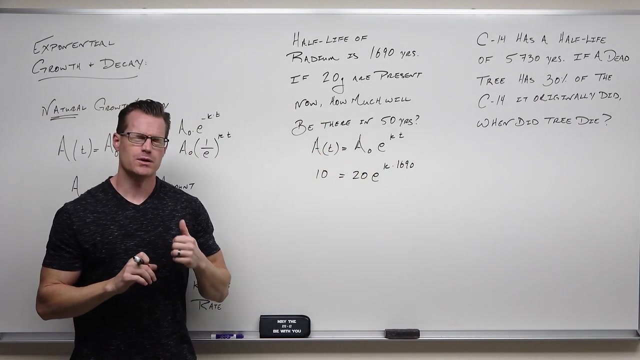 what a half-life says is there will be half of this after that much time and we're still solving for K. Notice I could give you the rate of decrease. so you'd say the rate of decrease is um whatever percentage? That'd be negative. 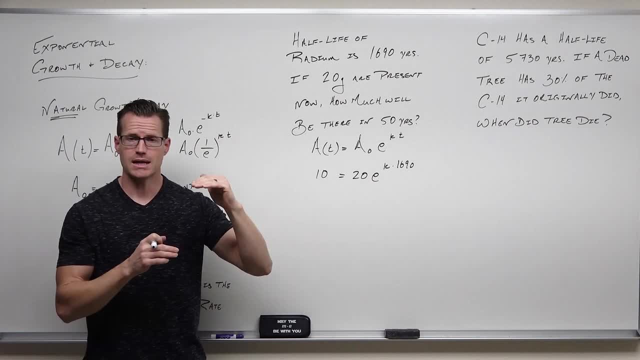 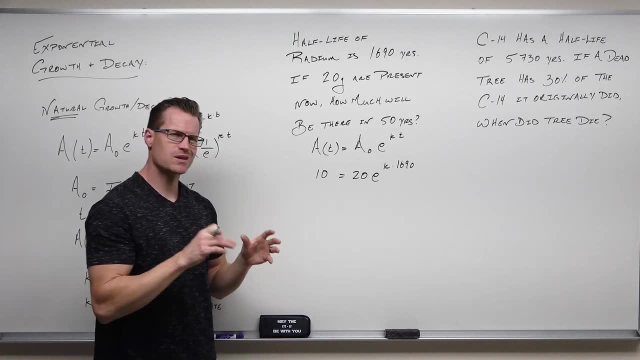 so, like, let's say, negative 15%, That'd be negative 0.15 as your K. Or if we say, decrease 50%, negative 0.15 for your K. Most of the time, though, they tell you how much you have and what. 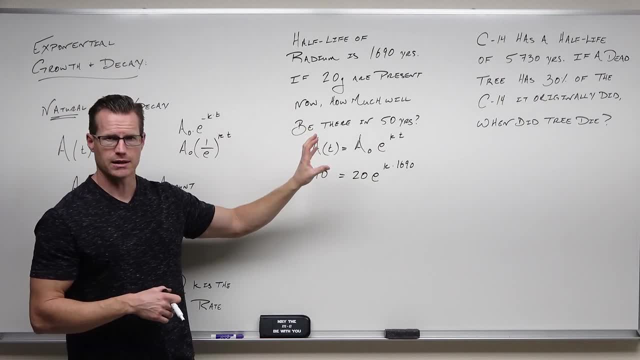 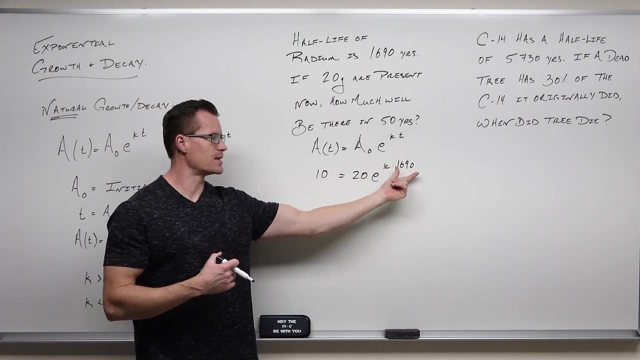 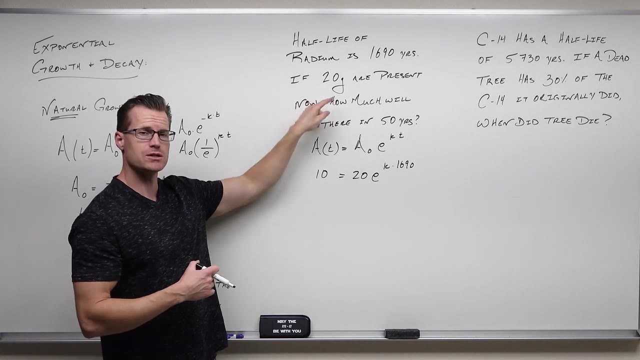 the half-life is as far as a length of time. So let's say we have 20 grams. now There will be half of it- that's 10, in this amount of time. So that's what a half-life is. Do you see? that will let you solve for K In general. they don't have to give you this. 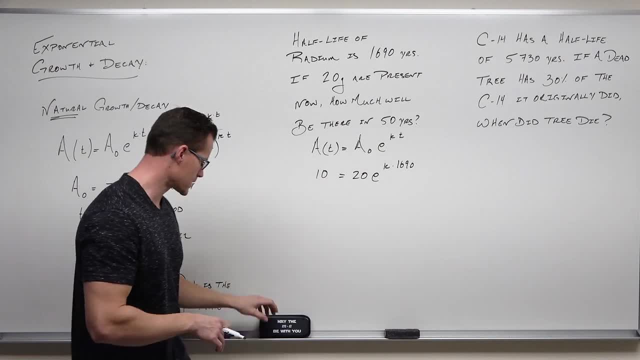 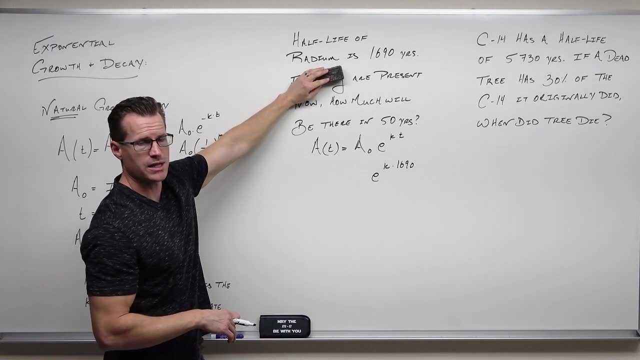 to find out half-life. I'm going to erase this, Just please watch this. What if, uh, what if they said the half-life of radium is 1,690 years? They don't tell you how much is present now. 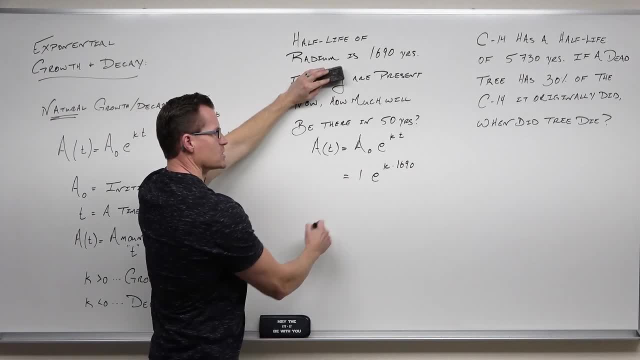 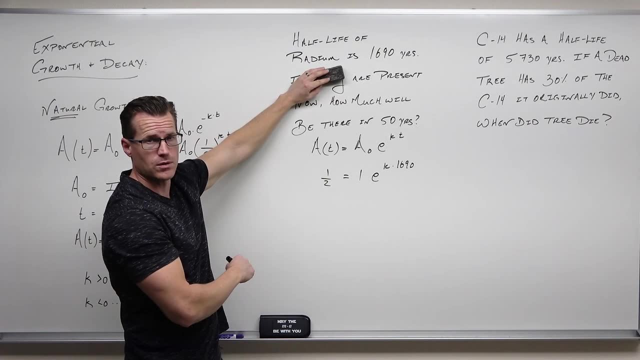 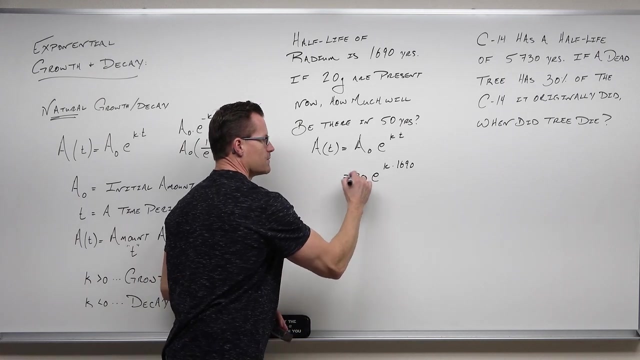 Well, what could you do? Couldn't you say: imagine I have one, one gram. How much would be present in 1,690 years? Half a gram or half of whatever That number is? You're going to see this when we go back to our hey, you have 20 in 1,690 years. 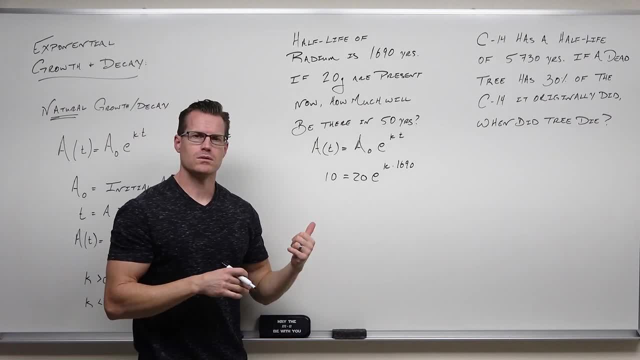 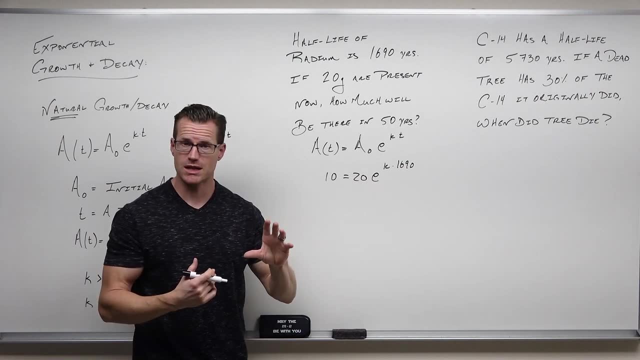 That's the half-life You'll have 10.. What's the first thing you do? Well, if we have to solve for K, we're going to need a logarithm to undo the exponential. but you have to isolate the exponential first. If we divide both sides by 20, this should be very familiar at this point- If we divide both, 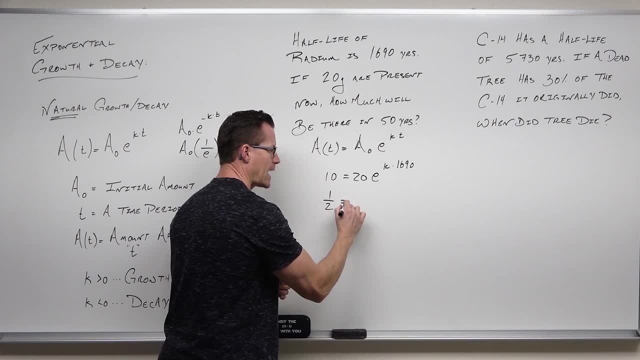 sides by 20,. 10 divided by 20 is- oh, look at that- one half. This will happen every time with half-life. That's what half-life means: There's half of it left. So if we divide both sides by 20,. 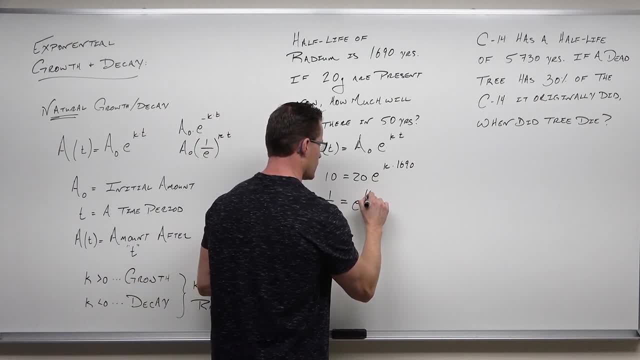 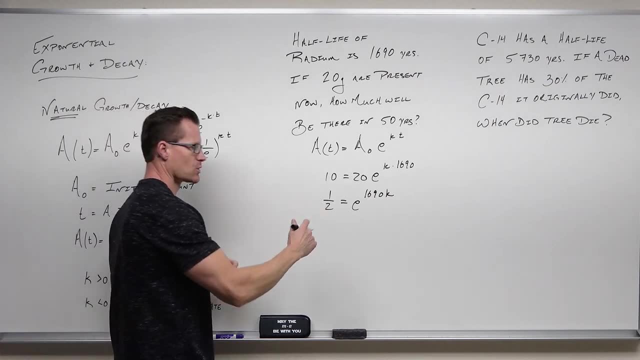 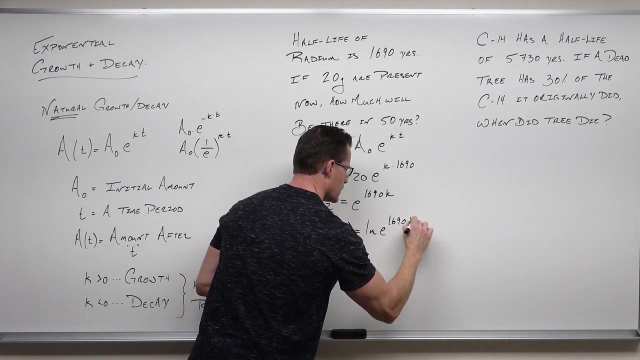 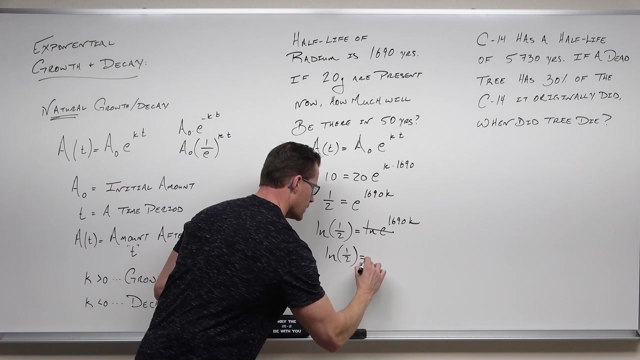 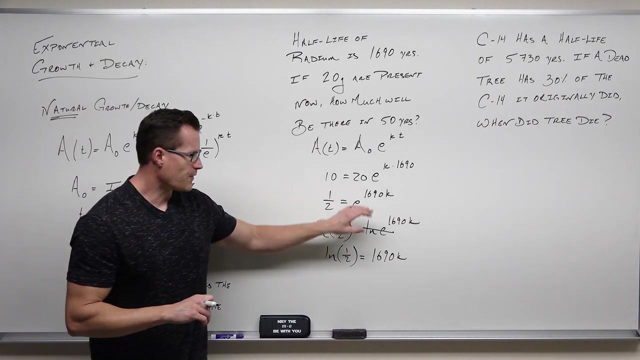 there's half of it left after that time. Now that we have an exponential isolated, we're ready for an ln, We're going to do a natural log on both sides. And lastly, because we simplify here, we can simply divide by 1690.. 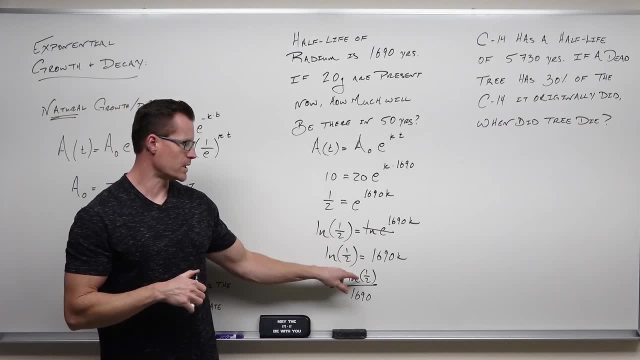 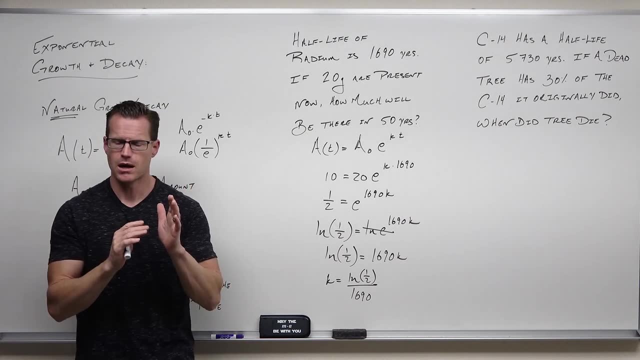 I hope this triggers something in your brain. I hope that when you look at this, you go: oh yes, natural logs or any logarithm of fractions less than one should give me negatives. Do you remember that Logarithms increase with bases that are greater than one, which we have? That's basically. 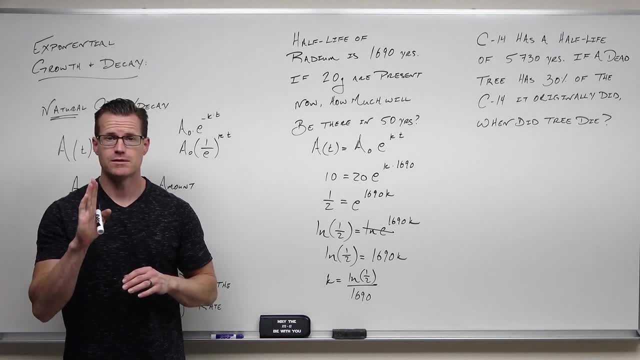 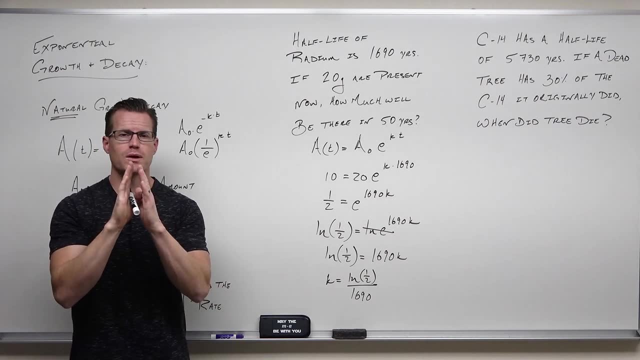 log and they are negative until x equals 1.. At that point 1, 0, they cross and then are positive. So if you plug in anything between 0 and 1, your logarithm will give you a negative here. 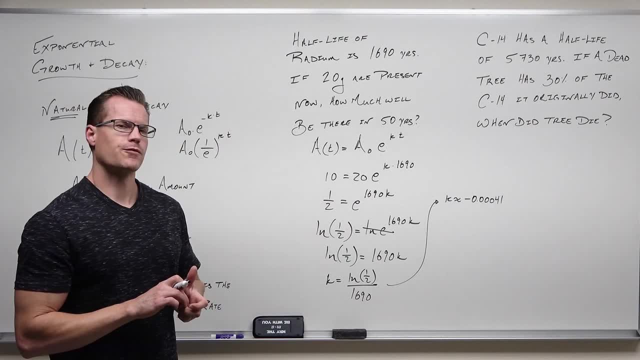 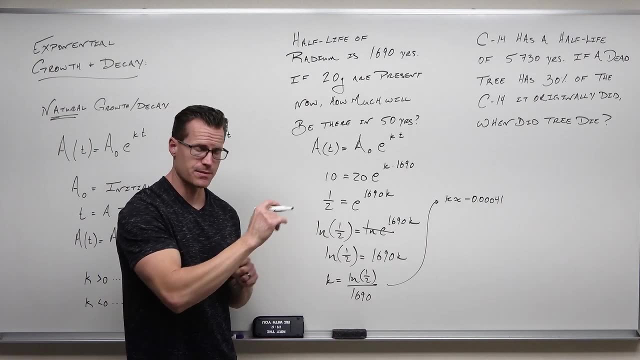 Divided by positive is still going to be a negative. Be careful with your calculators. Make sure you have parentheses. after that 1 half You want to press ln 1 half, end parentheses and then divide by 1690.. 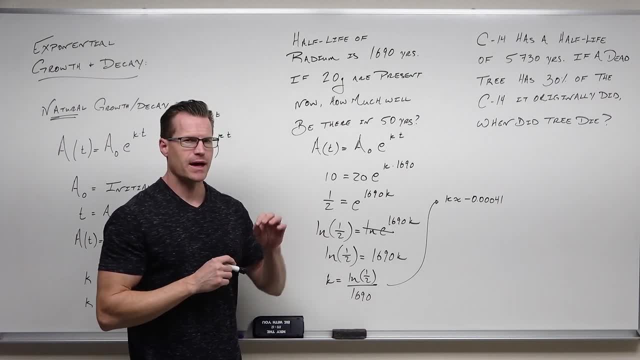 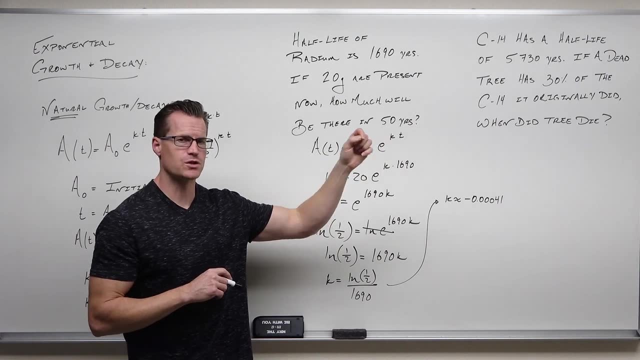 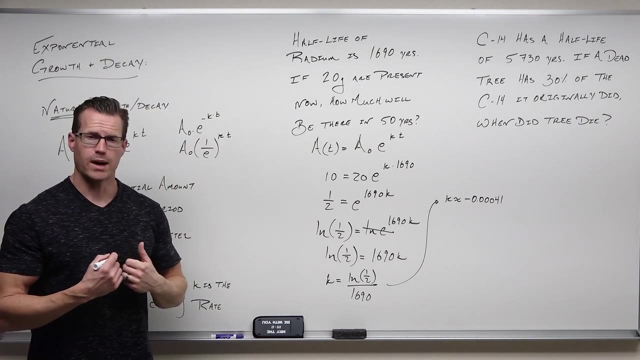 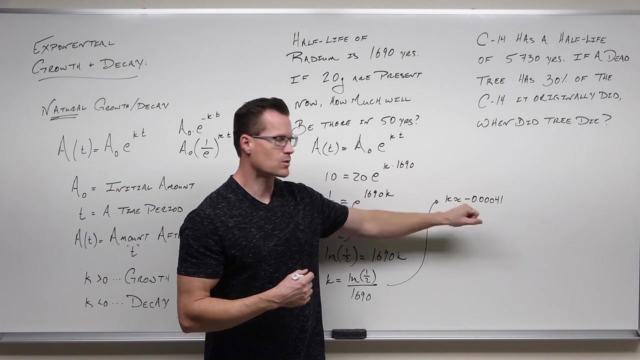 I got negative .00041.. If you get that exponential scientific notation, just remember that moves your decimal to the left if it's negative. So we move left four spaces and we get this .00041.. That is the rate of decrease. This radium is decreasing at the rate of .041% per year. 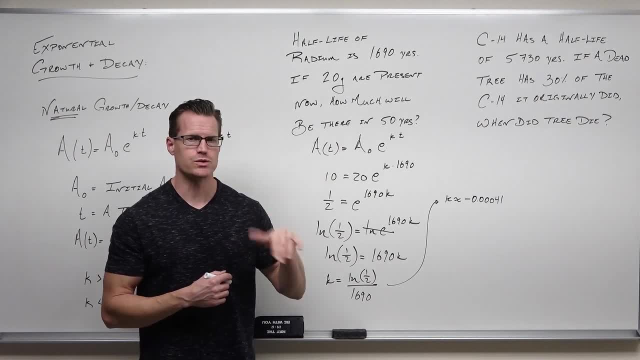 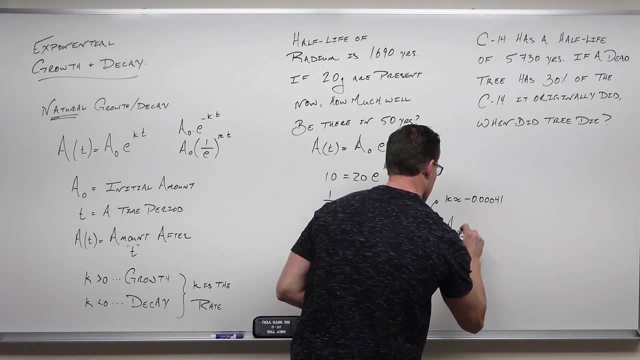 That is what that means. It's not very quick. That's why it takes 1690 years to lose half of it. So what that means for us, we can put this back into our formula. I'm leaving this blank, intentionally for a second. 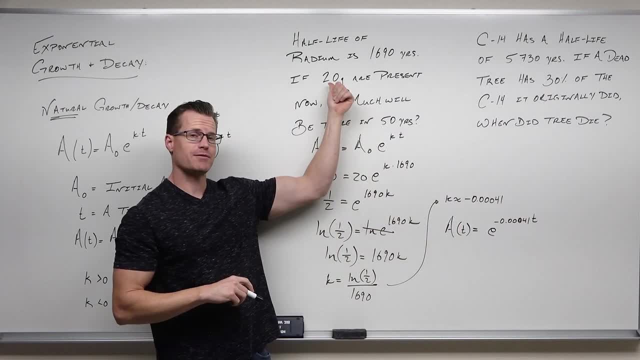 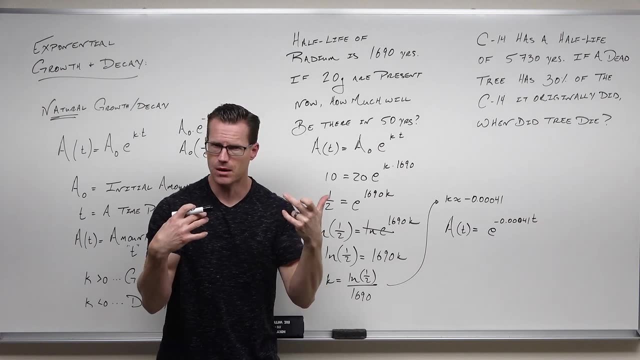 On purpose, to show you that this really did not have to be here in order for us to figure out our k. Our half-life is always done the same amount. You'll just have one half of your amount that you started with, or 50%. 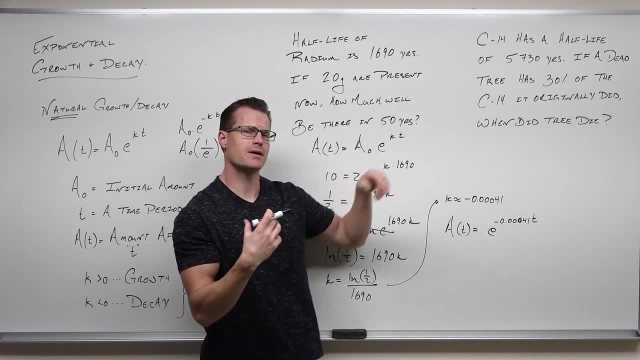 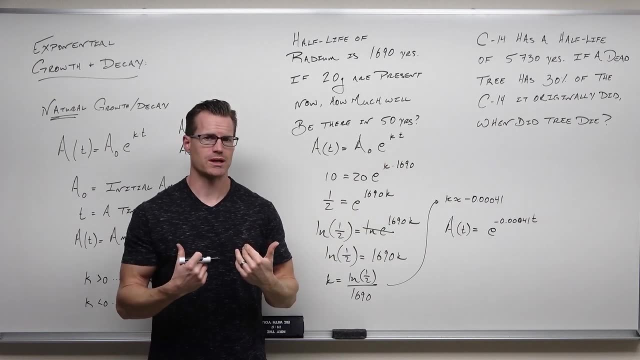 0.5 of whatever you started with. that's going to come in right there: 30%. After that you're able to find your k, you put it back in your function and then it can ask you any sort of question, like: 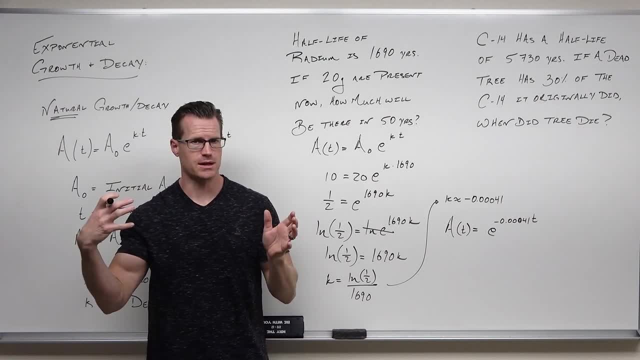 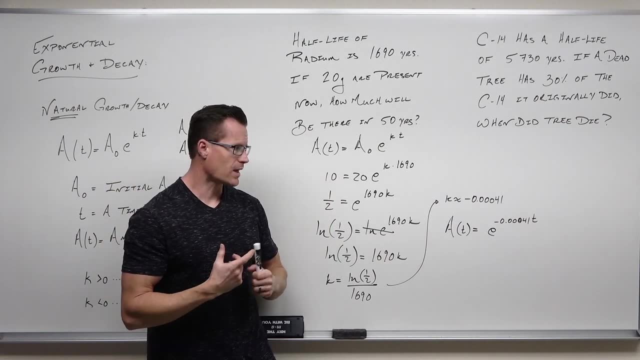 suppose you start with whatever amount, find this or how long it would take here. Suppose you want to find this amount, however long it would take, you can solve for that. We can do lots and lots of different things with these equations. 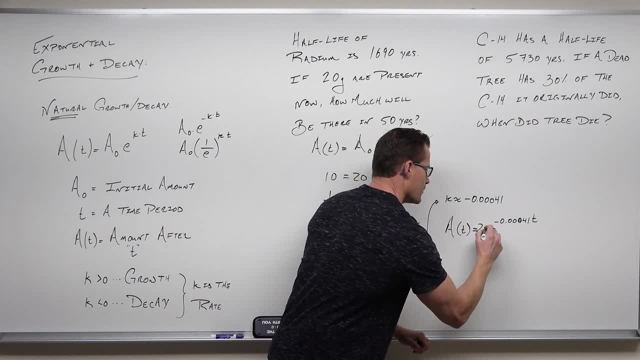 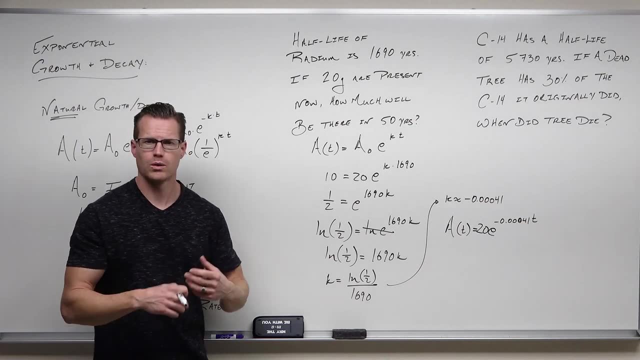 We just have to solve for k first. Now, in our case, this says that we have 20 grams of k. We have 20 grams of radium present. How much will be there in 50 years? All we're looking for is this, evaluated for 50 years. 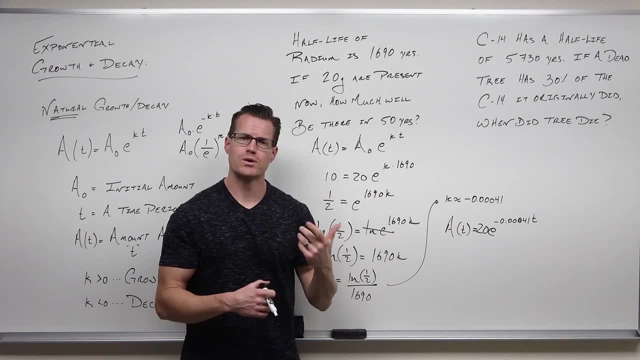 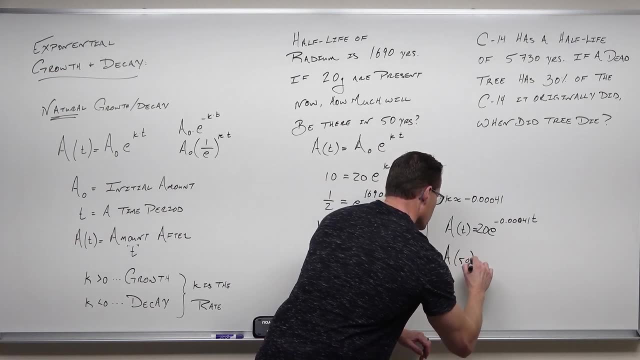 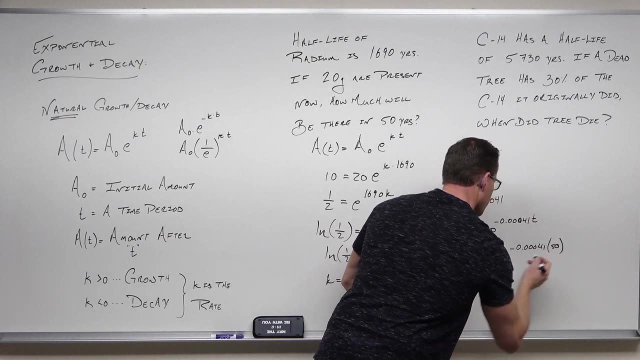 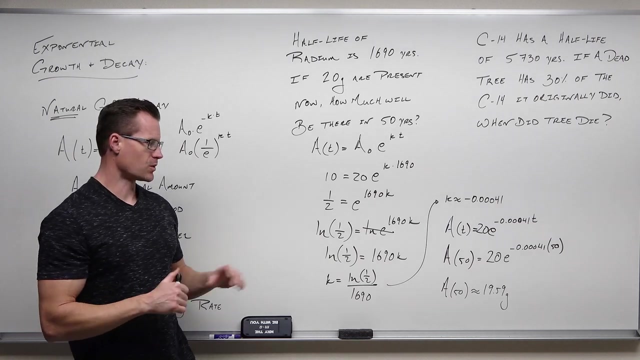 You see, this gives you the rate of decrease. It tells you how much you started with. We're saying how much will be there after 50 years has passed. So we just plug in 50 and evaluate. I got about 19.59 grams. 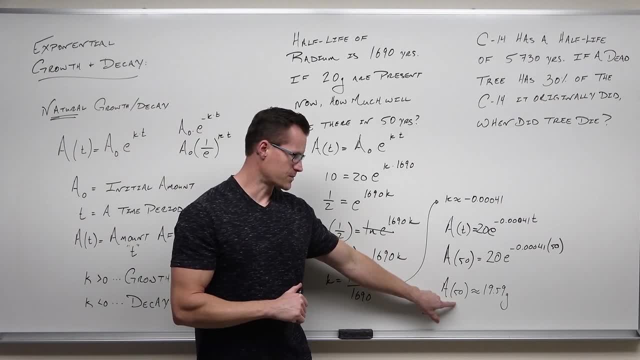 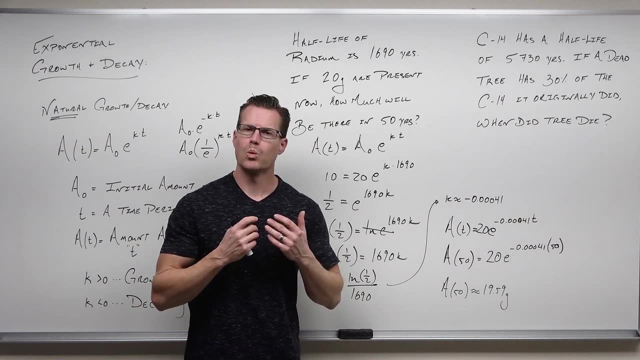 So what this means is that the amount that's going to be left after 50 years has passed is 19.59 grams. considering you start with 20 grams, That's not much. Well, I'm sorry, That's not much decrease. 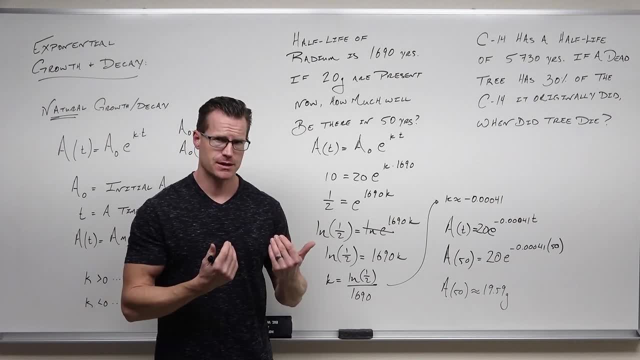 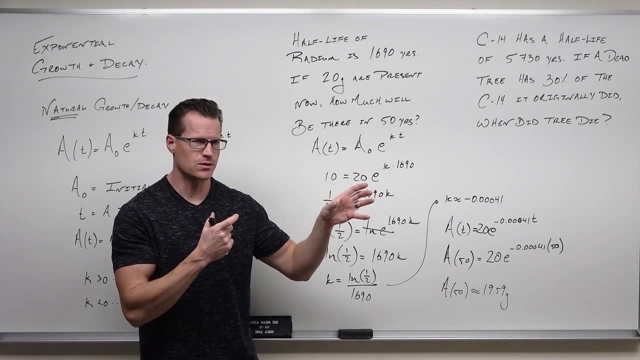 Well, that's true, But if you lose half of it in 1,690 years, that means that there would be 10 grams left after 1,690 years. right, It would take 1,690 years to lose 10 grams. 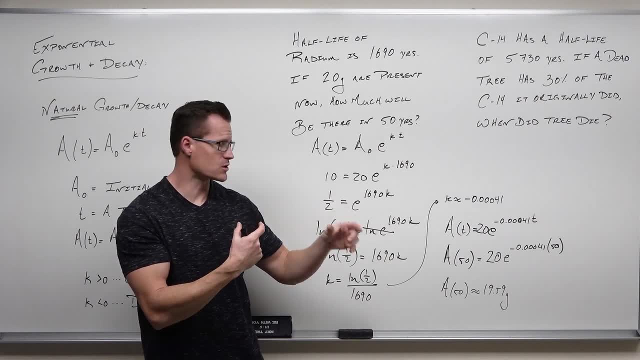 Well, that's true. Well, 50 years is not even close to 1,690, so you're not going to lose very much in that short amount of time You are losing. It is decreasing, but the rate is very slow. 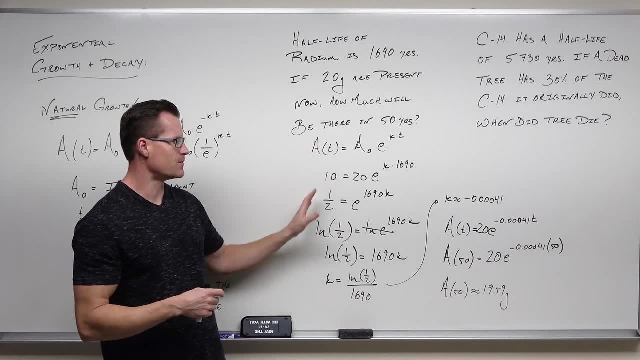 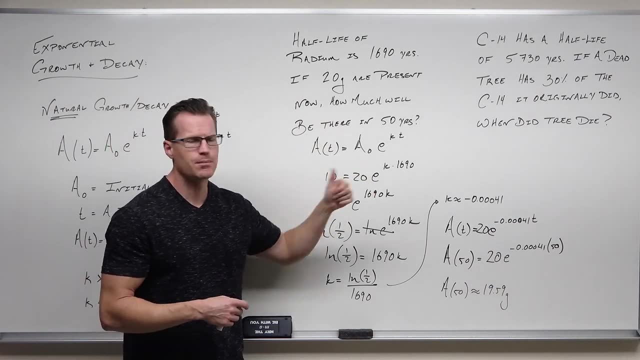 I hope that makes sense to you. I hope you're seeing the idea of: hey, half-life means one half. I can solve for K, Even if I don't tell you what to start with, you can still solve for K. Then I can ask you a number of questions after that. 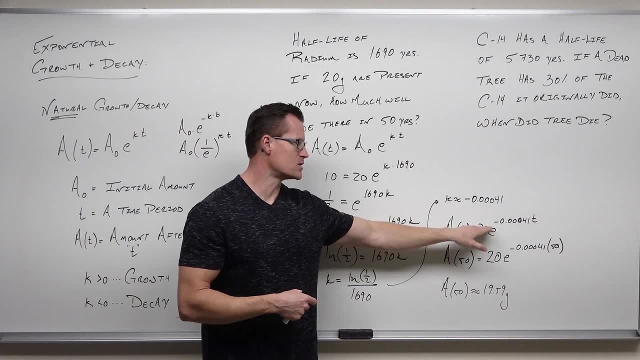 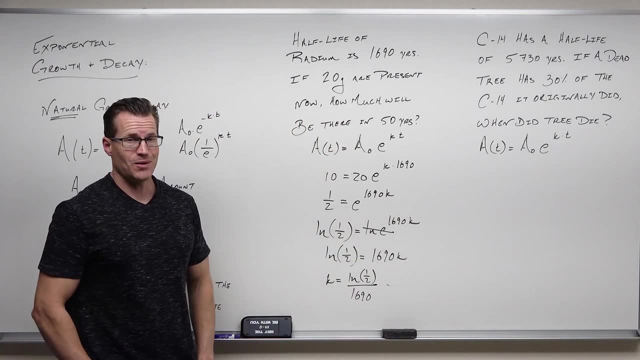 I can have you solve for how much it would take to get to a certain amount, how long that would take. all sorts of different questions on that. Okay, All right, we're ready for another example. So C14 has a half-life of 5,730 years. 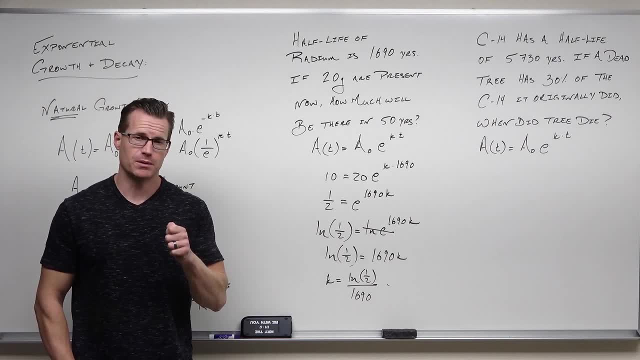 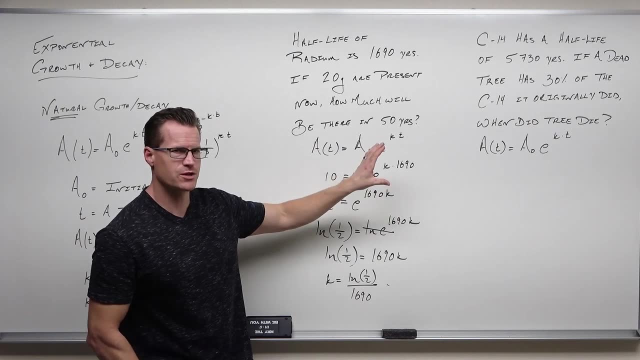 Stop right there. With just that information, you should be able to solve for K, and that's exactly what we're going to do first. We're going to solve this for K almost right now. I'm going to read the rest of it just to get an idea of where we're going. but that first. 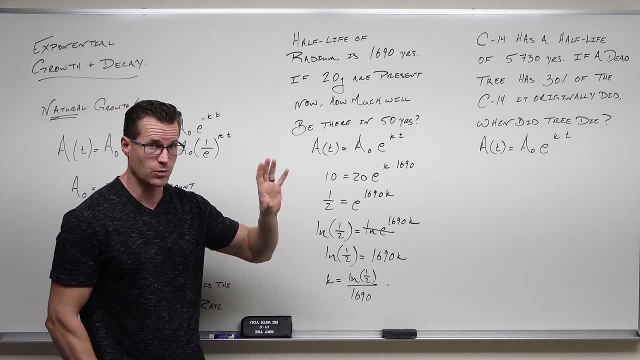 sentence lets you solve for K, and that's a must if you want to answer any of the questions. So we're going to pause right there. Now, if a dead tree has 30% of the C14 it originally did, when did it die? 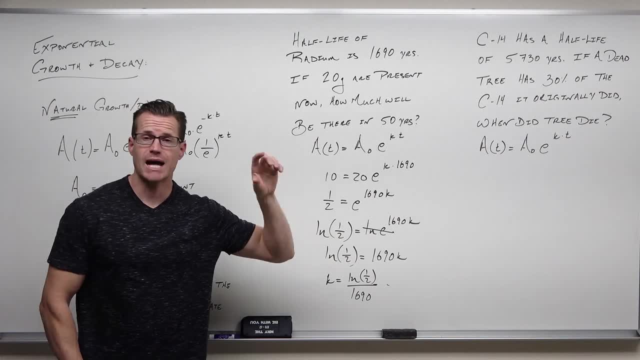 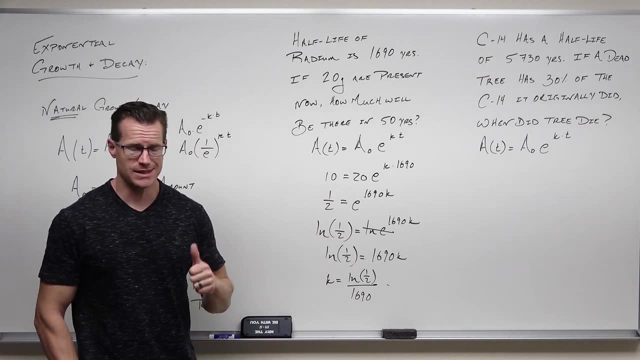 That 30% that is used after you have found K. Some students they really want to make the K 0.30.. That's not what that 30% is. I understand that because you're like, oh, that's a rate. 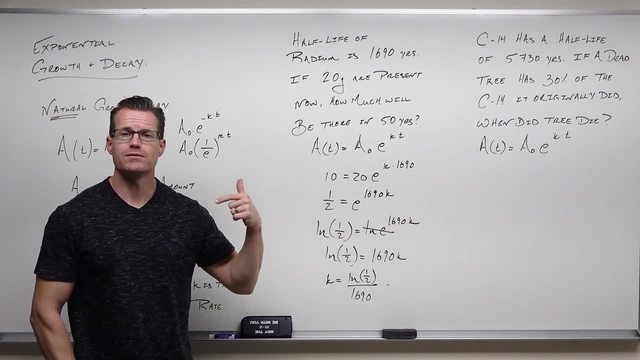 It's really not. If I had given you a rate, I would say: the rate of decrease is 30% And you could say: oh okay, that's negative 0.30 for my K. That's not what's happening here. 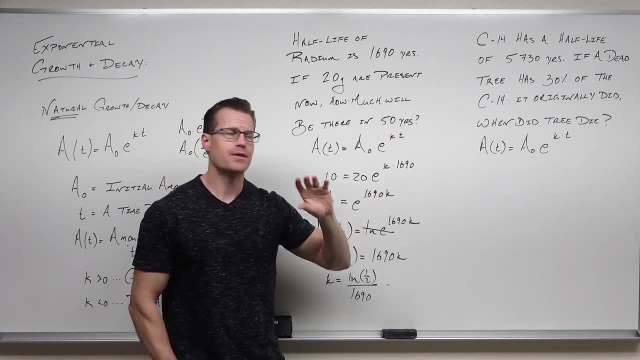 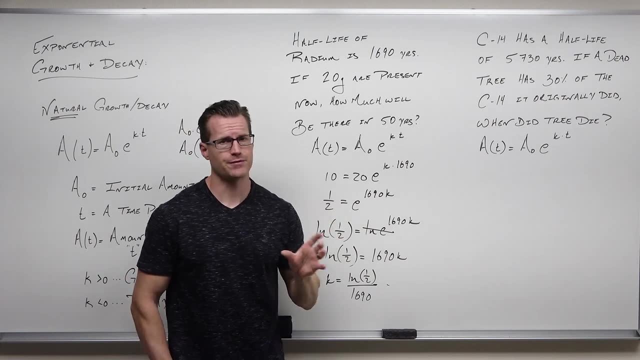 What's happening is we're going to use our half-life to figure out our K, and then this next sentence says: now that you've done that, tell me how long it takes. How long it takes to achieve 30%. That's a different story and it comes in later. 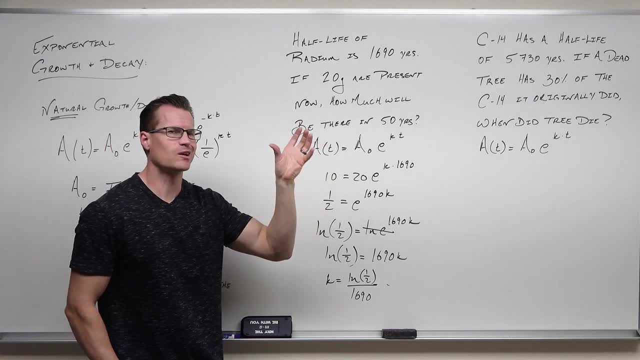 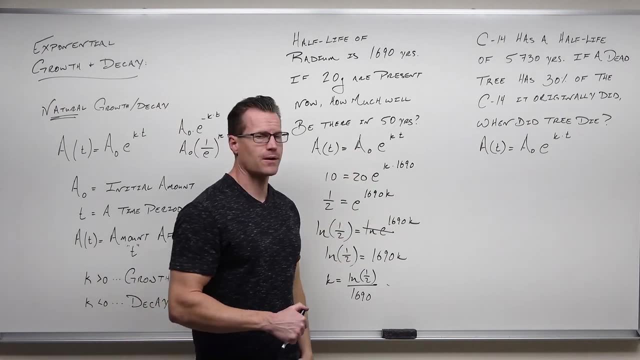 It asks something like how much is going to be present in 50 years? but a little bit differently, has you solve for a time. So, number one, you got to find your K first. The half-life statement up there is enough to do it. 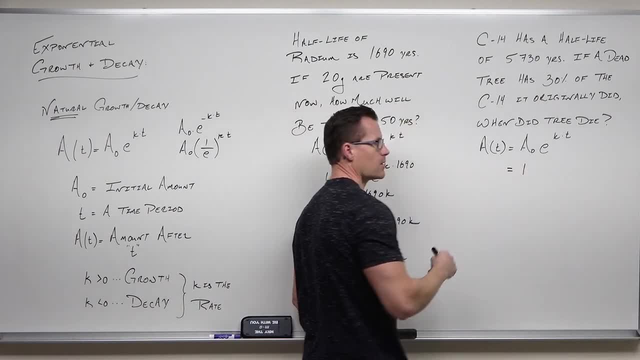 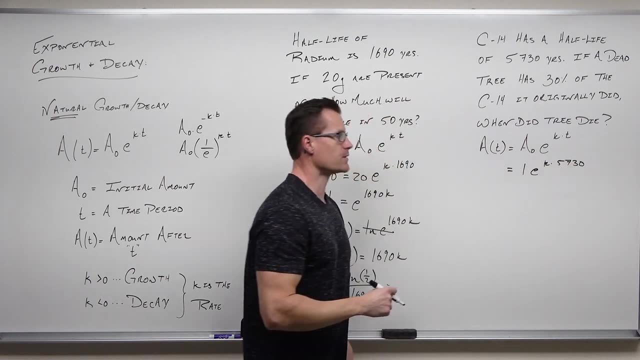 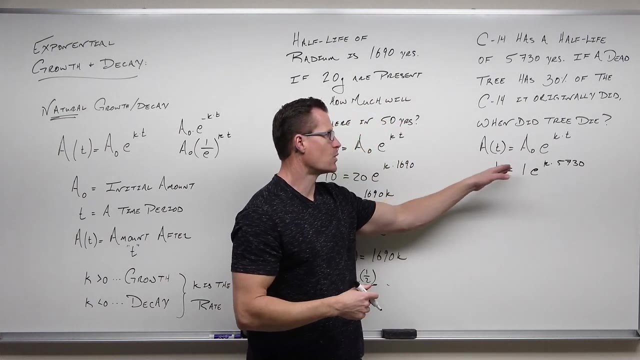 The half-life statement says: if you start with any amount- let's call it one- and you give it 5,730 years, how much is going to be left? Half of it, I don't care. if you start with 10 and you want to put 5,. start with 100, put 50, start. 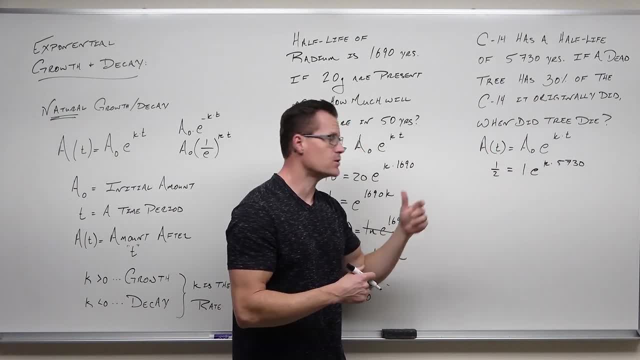 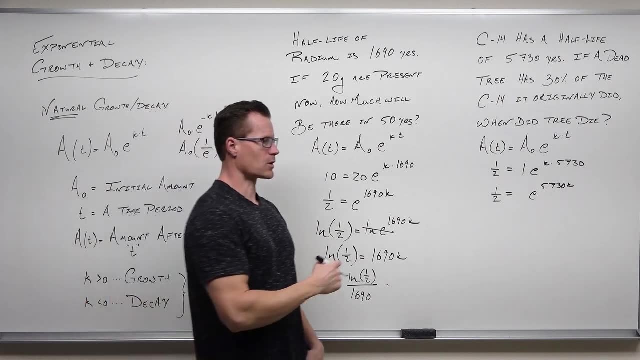 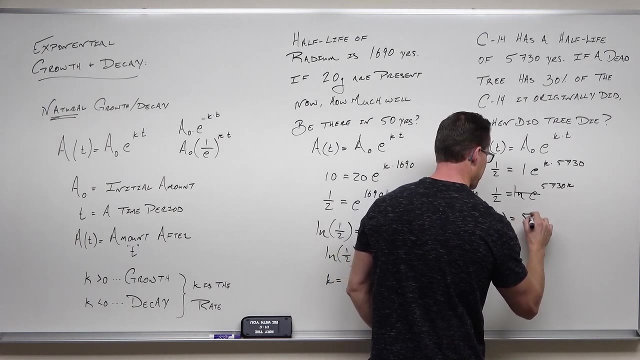 with 1,000, put 500. The first thing you do is divide and then you end up getting to one half, Because that is isolated or exponential for us. we just have to take a natural log of both sides. You probably should see at this point that half of it is going to be left. 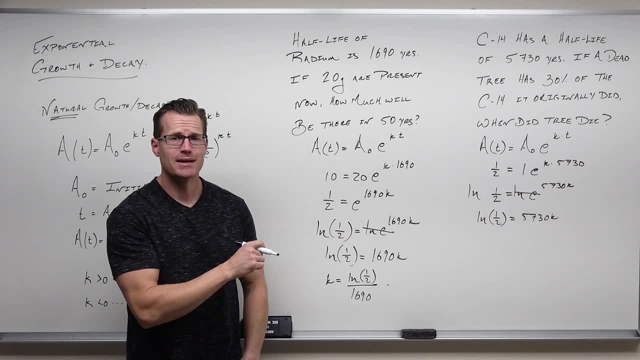 Half of it is going to be divided. Half-life is going to look a lot like this a lot of the time, because if it says how half-life is this many years, well then we know that 0.5 or one half is going to equal. 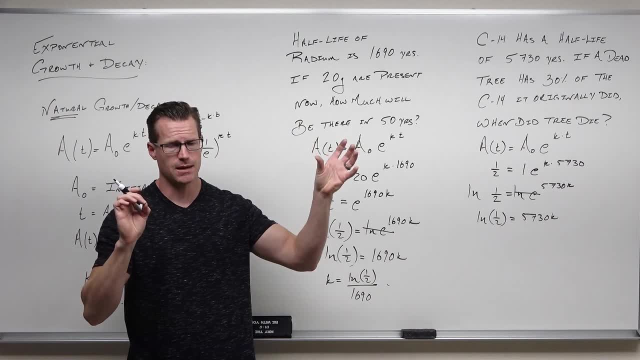 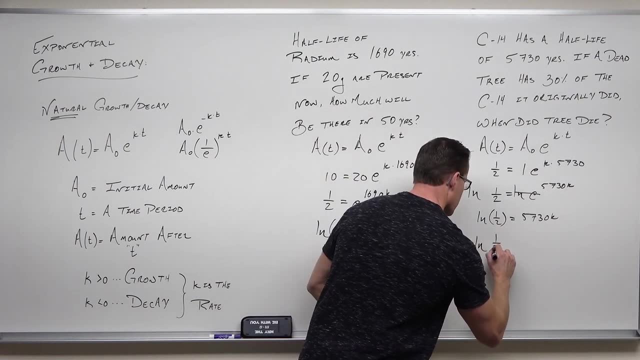 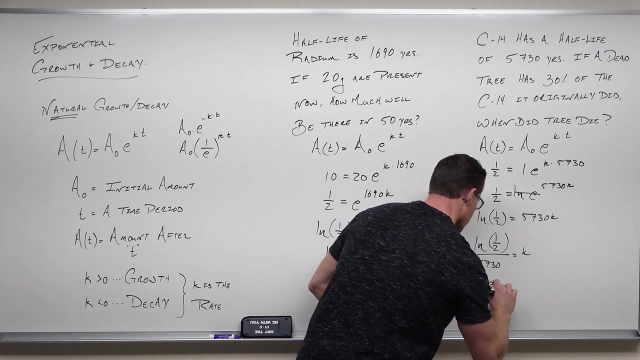 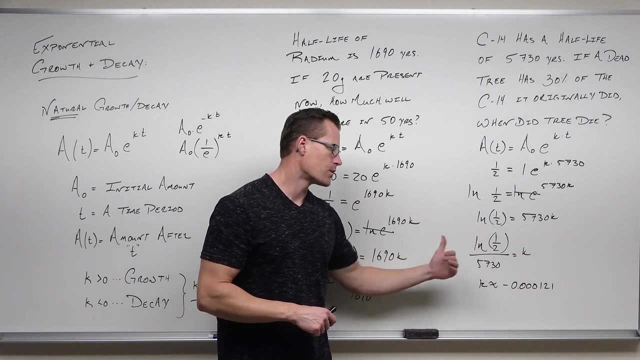 E to the. whatever the number of years is, times K, It will let you solve for the K. So let's do that. Let's divide by 5,730.. Okay, try to be as precise as possible. Don't round this as much as you're able to, because we have to deal with a really small. 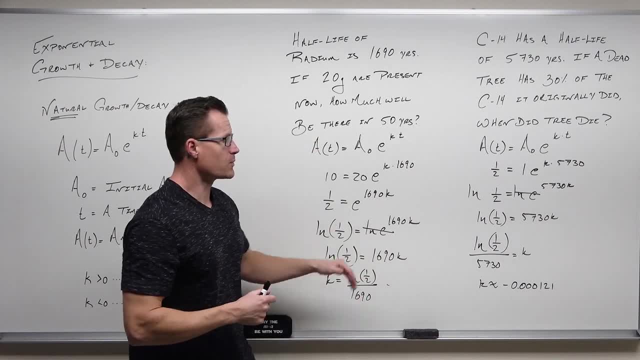 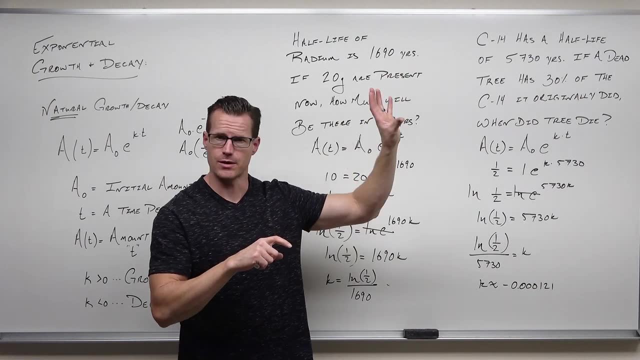 number. We really want to be as precise as we can be. So what that means is that we have this rate of decrease. Why decrease? Well, it's negative. That negative exponent would make this 1 over E to some other power. 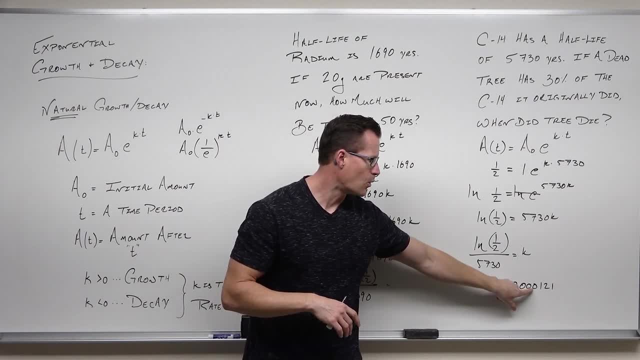 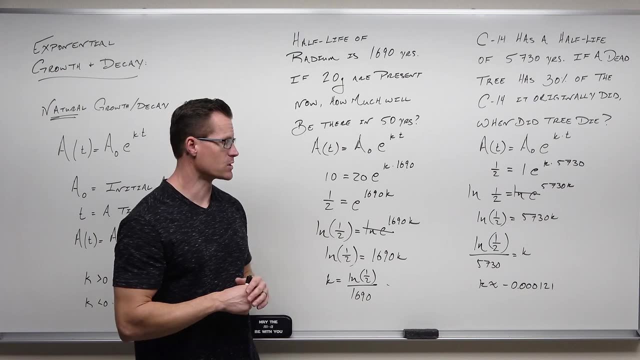 That is a rate of decrease. It's decreasing at, let's see, 0.0121% per year. That's how quickly this carbon-14 is decreasing. That's the rate of decrease, right there. So what we're going to do now is going to rewrite this formula that we have, but using 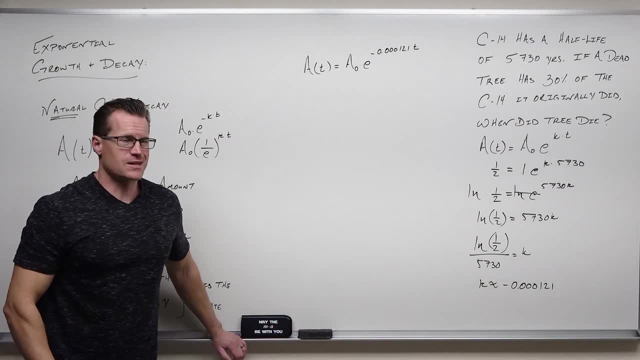 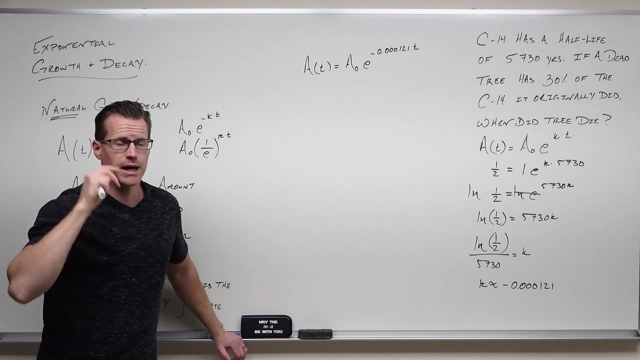 this information. I also hope you're seeing this as a several-step process. This isn't just you plug in all the numbers and you get it. You first have to use your information to figure out your K And then on your second step, like after you've found your K and after you've plugged into 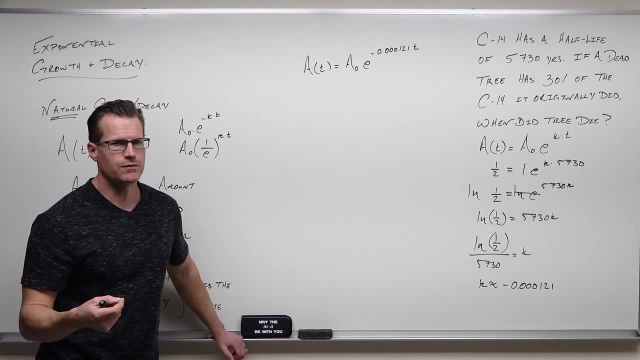 your formula, then you can answer anything else. Now the next question is a little bit confusing for a lot of people who go: well, wait a minute, What do you mean? 30%, I don't know how much I originally had. 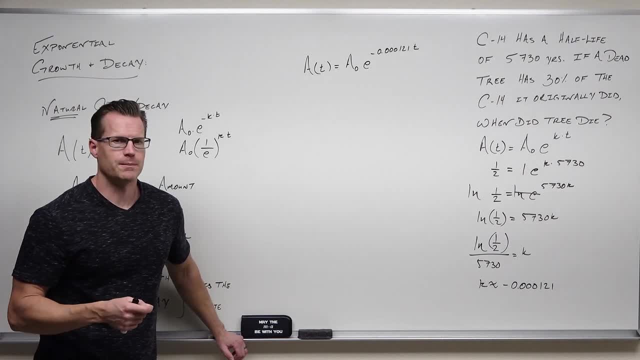 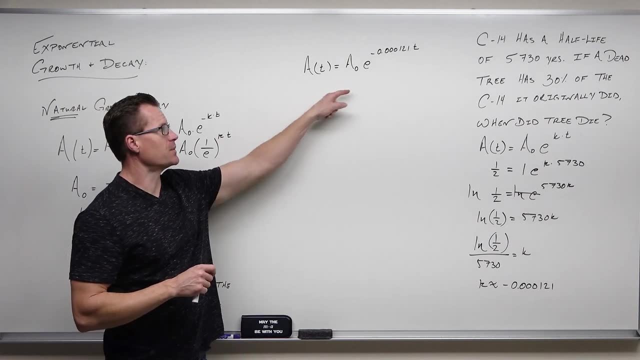 How am I supposed to find 30% of it? Well, I don't know. Well, here's the point. No matter what you originally had, if there's 30% of it remaining, this is going to end up being 0.30, equal to whatever your exponential is. 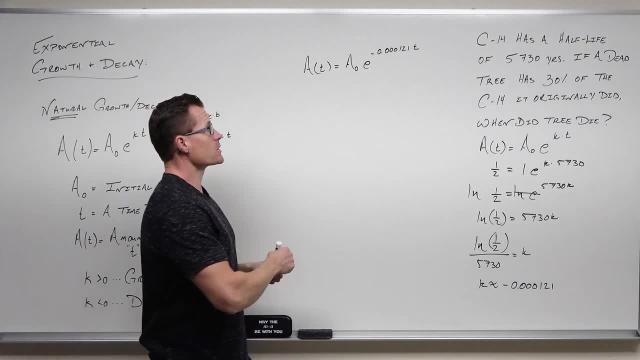 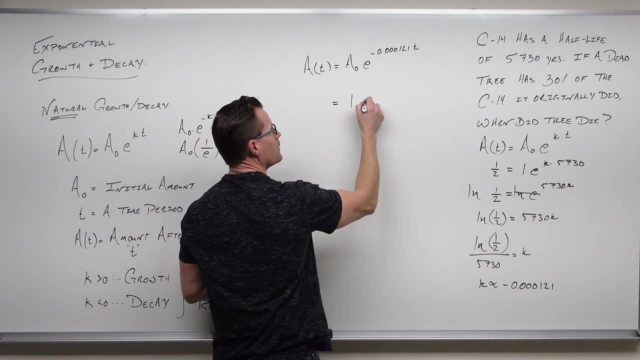 Why? Well, because how would you do this? You start with some amount. Let's call it one. Now, I don't care if you call it if it's one or a hundred or a million, it doesn't really matter if we know our rate of decrease. 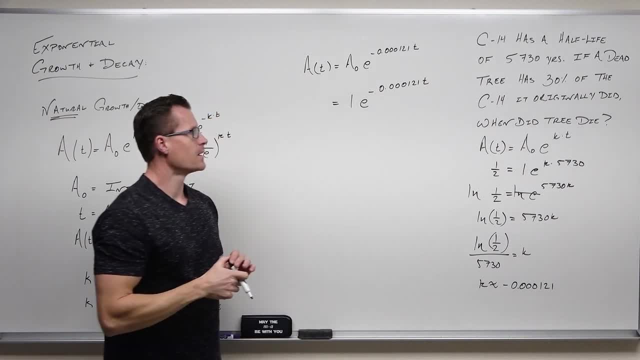 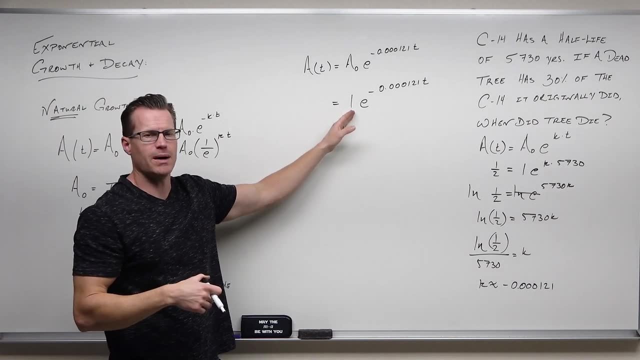 Okay, Okay, Okay. Let's say we know that the tree had 30% of its original carbon 14.. So if we start with- let's pretend, this one gram, how much would be left? 0.3 grams, That's 30% of what I started with. 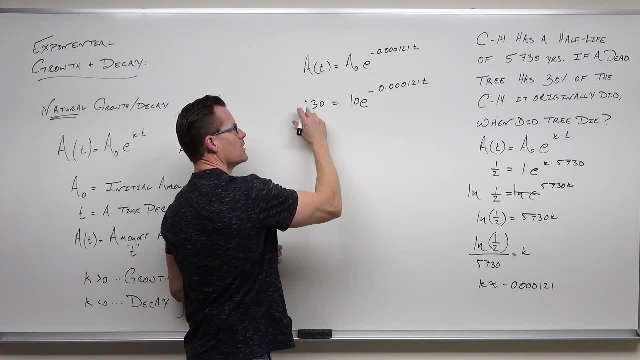 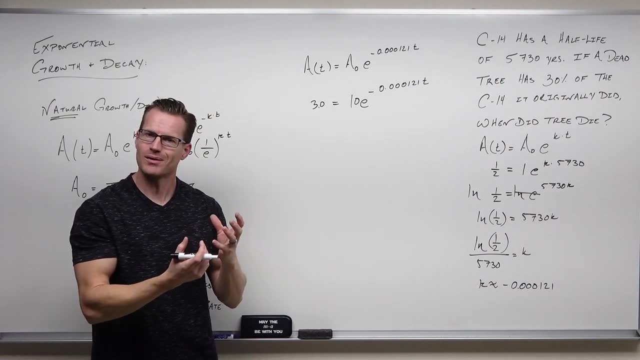 Now, what if it wasn't one gram, if it was 10 grams? well then, what's 30% of 10? Three? What about a hundred grams? What's 30% of that? It would be 30. But the very first thing that you would do in any of the cases is you'd have self exponential. 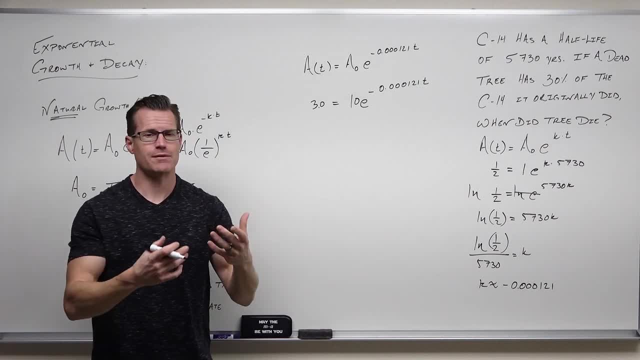 You have to self exponential. You have to self exponential, You have to solve for t. So if you did that, you have to isolate it. If you isolate it, you have to divide both sides by 10, but wait a minute. 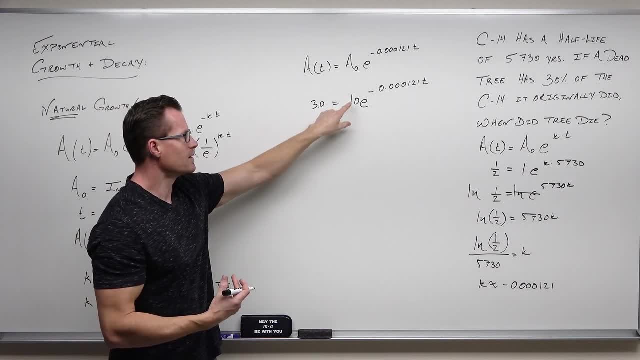 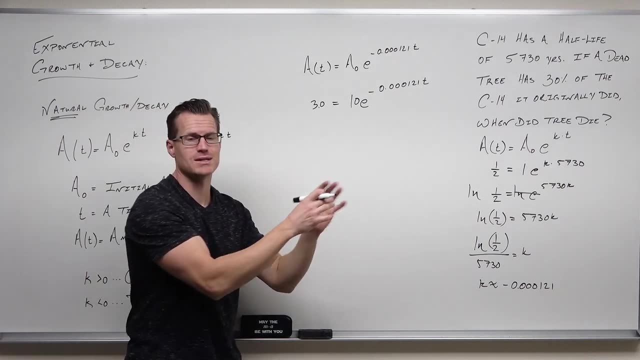 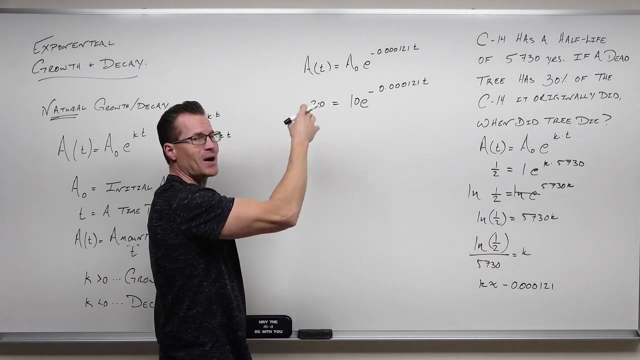 If, in this case, if if you are going to find 30% of this number and then divide it by this number, you're going to get 0.30 or 30% or whatever percentage is every time. So if I divide 3.0 by 10 or 0.30 by one or 30 by a hundred, I'm going to end up getting 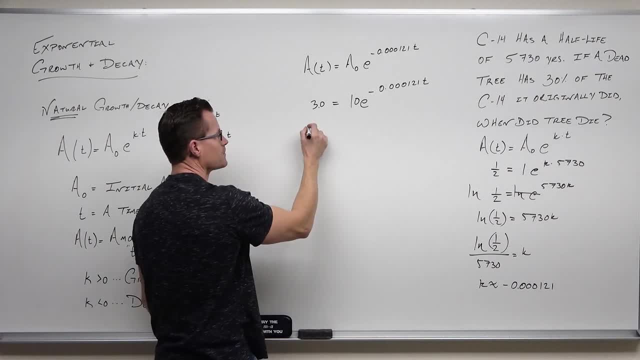 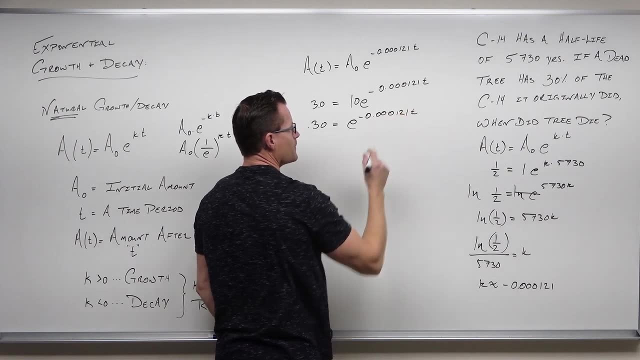 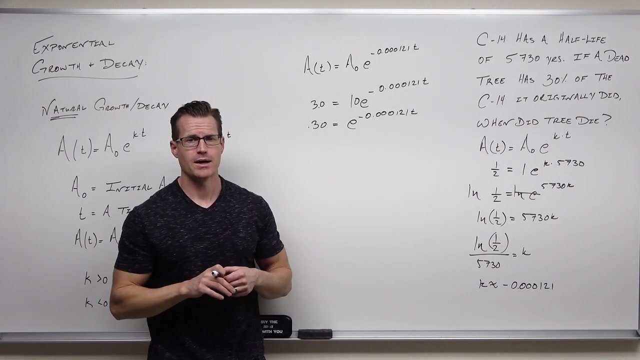 0.30, no matter what, as I isolate that exponential. Okay, I guess that's just to say that when they give you a percentage it's much like doubling. It's actually much like half-life. If you did, if you remember the half-life this said: you have half of what you started. 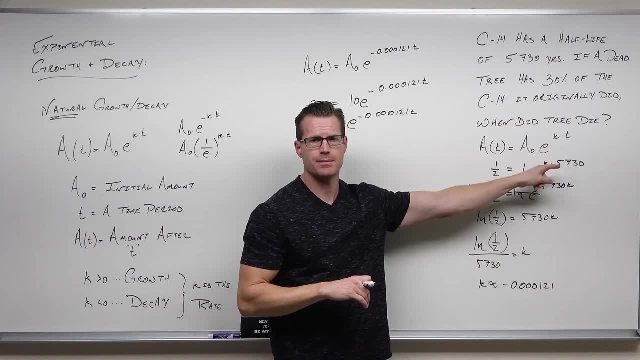 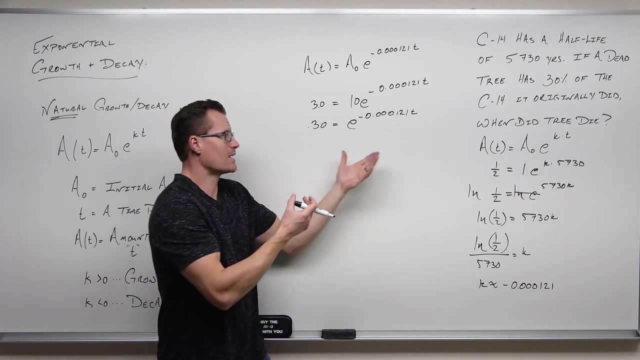 with 50% of what you started with after that amount of time, unless you solve for K. now it's saying: okay, uh, you have 30% of what you started with, 0.30 of whatever you started with. That's what I wanted. 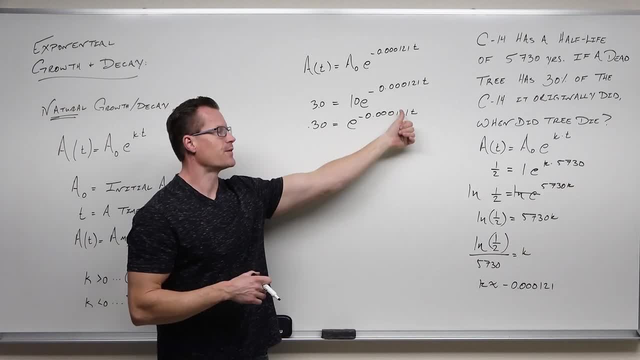 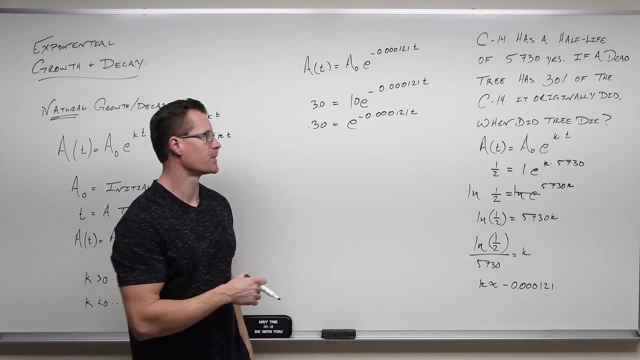 It doesn't really matter because what's good. What's it saying is: you have 30%. now figure out the time that it took to get that 30%. So same exact idea. It's just now you're looking for the time it's taking. 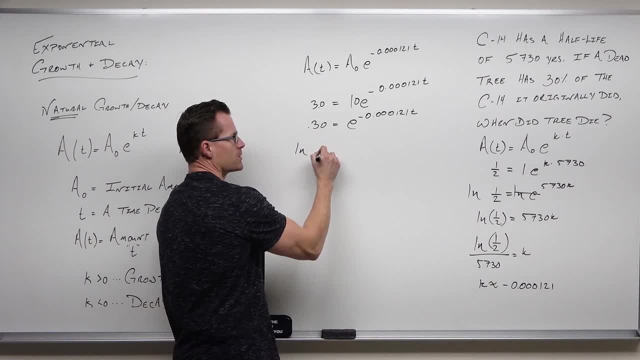 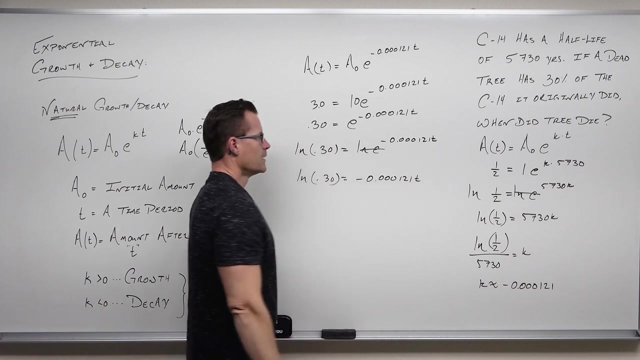 And since we have the K, we're allowed to do that. Let's do a natural log of both sides. Okay, Okay, Okay, Okay, Okay, Okay, Okay, And I'm just working that down- We do an LN. Of course, this composes a function: inverses, cancels. 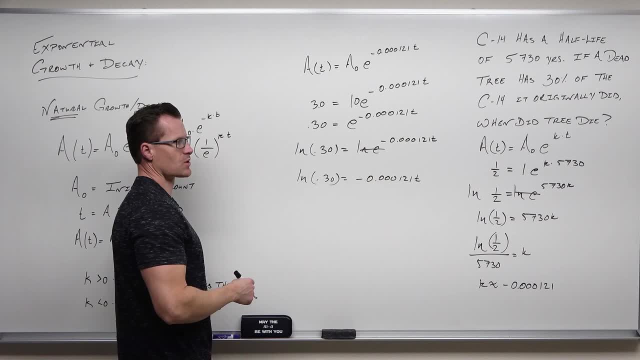 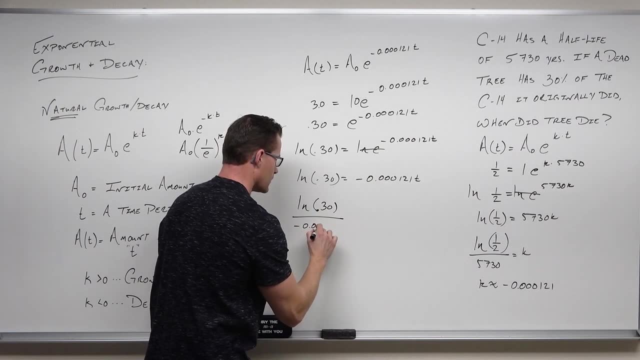 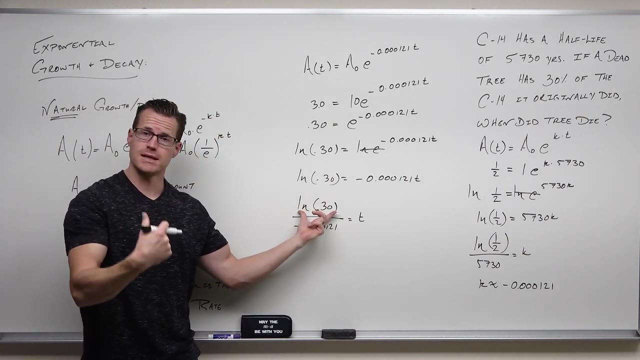 If we divide both sides by that negative 0.000121,. hopefully you recognize I have an LN of some value, less than one. That's a negative divided by another negative should give me a positive. That makes sense. Time should be in the future here. 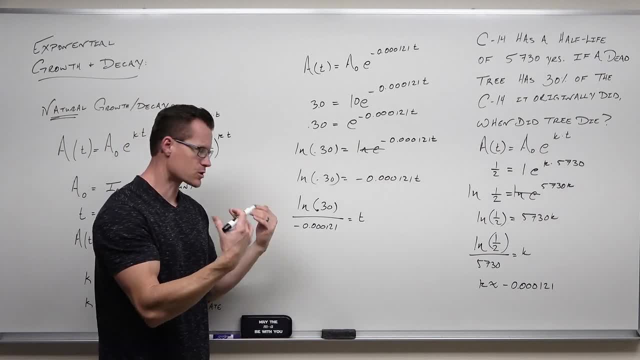 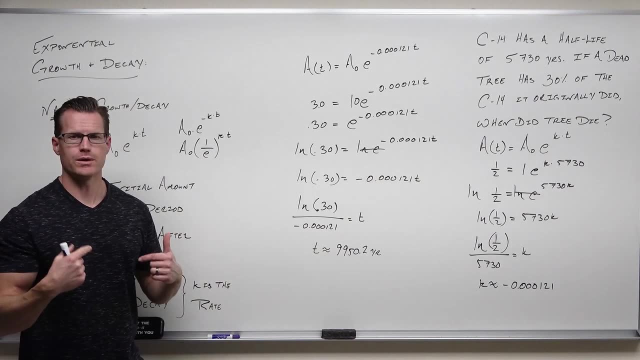 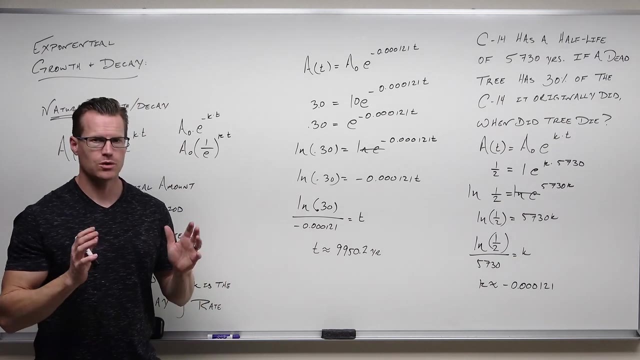 or some positive value that's saying this is how long ago this tree died. I am getting 9,950.2 years ago is how long ago this tree died, And what that means is that that long ago this tree would have died and it would have 30% of the original carbon 14 that it 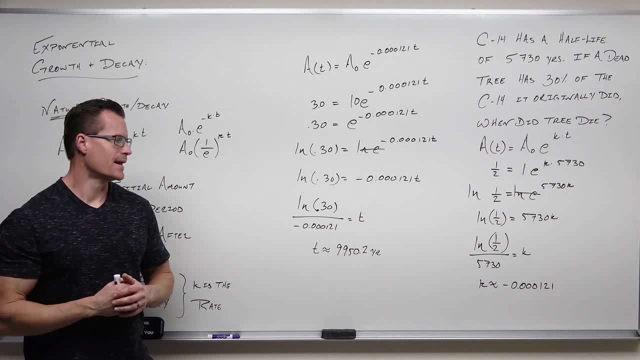 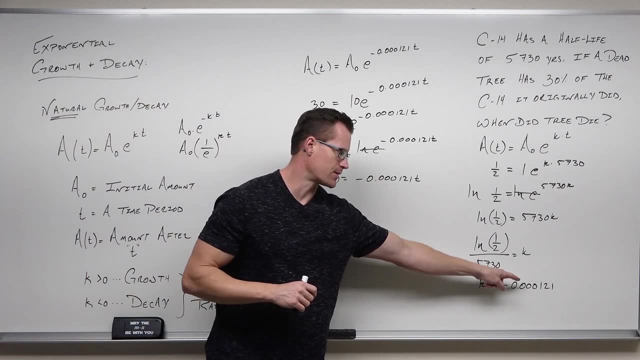 had back then, And so they go backwards to try to date that. The last thing I'm going to mention is this number is is definitely off, And the reason why is because I rounded pretty heavily right there It didn't look like. yeah, I went to like the what sixth decimal place, but I cut off a lot. 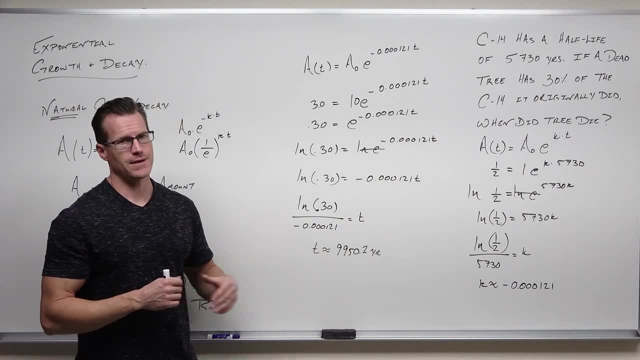 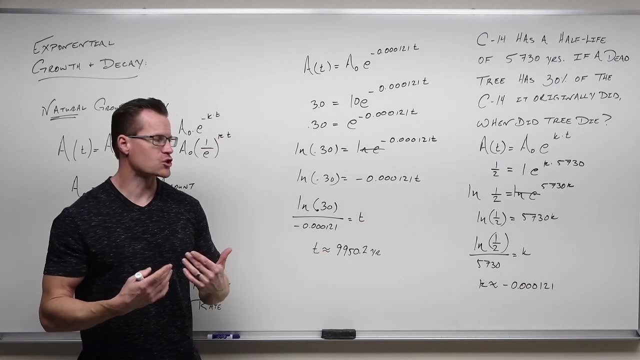 of numbers. So when you do that, you're going to really affect this outcome. So I'm saying about 9,950.2 because I didn't want to write out a whole bunch of digits, but in actuality you probably shouldn't round this at all, to be honest with you. But that's. that's just what I had to do to. 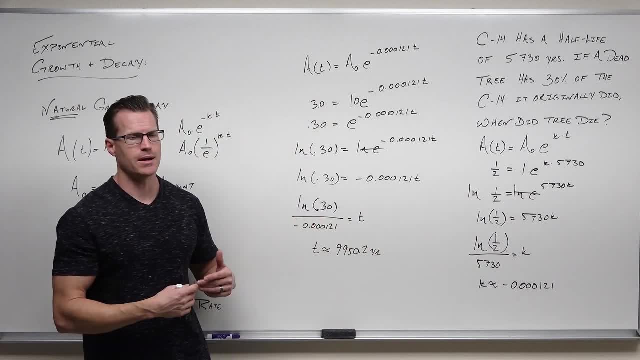 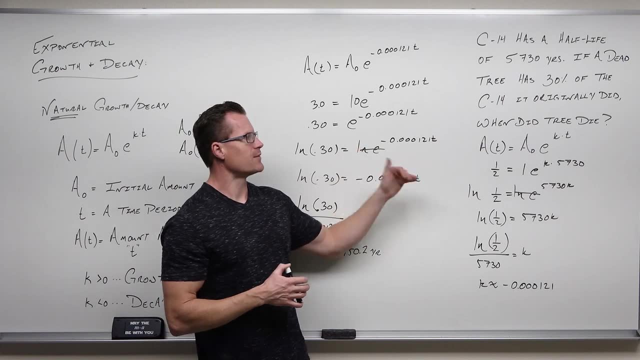 make you understand what the rate was here. So I did that, but this is probably off by- I don't know- two or three years. So anyhow, I hope that makes sense. I hope that you're seeing that half-life takes a percentage after a certain amount of time. So that's for K And. 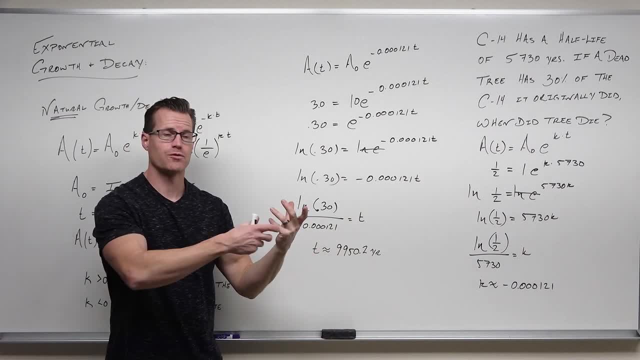 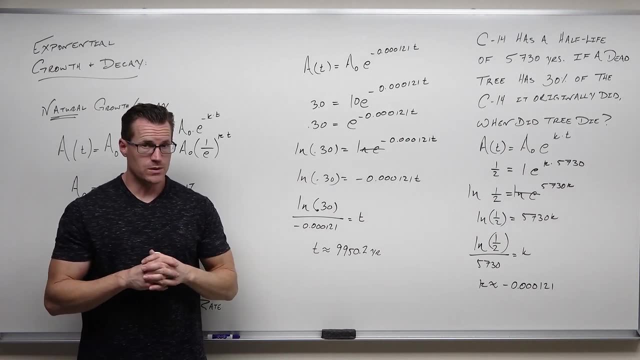 that's exactly what this is doing. It's saying: what is the amount of time for which you to get that percentage? So I hope I've cleared that up. What we're going to do- in your mind at least. what we're going to do now is come back with one more example, kind of fun one, And then 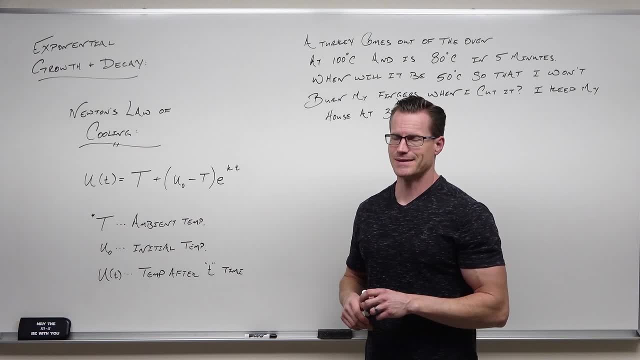 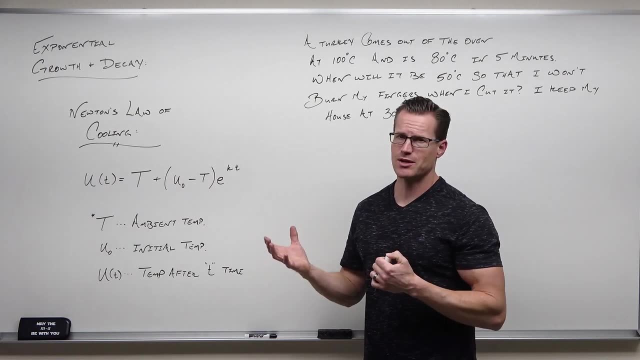 then we'll be done. Last one: We're going to talk about a Newton's law of cooling problem. I kind of like these. I also want to tempt you to get into differential equations, because we cover this much, much, much more at length. We talk about where this actually comes from. It's pretty. 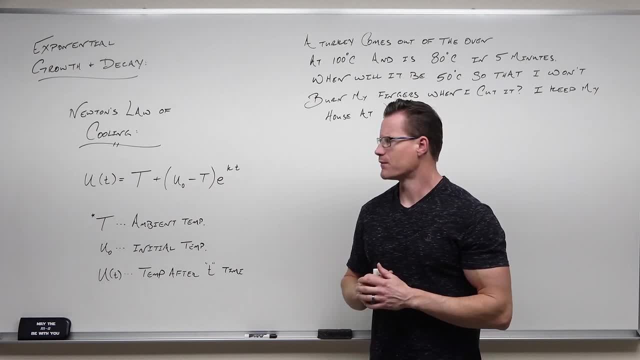 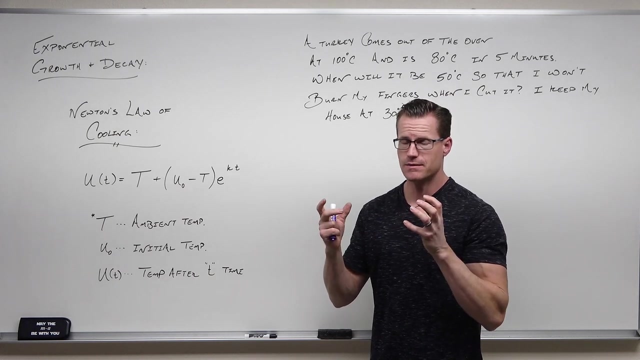 neat. So Newton's law of cooling is is kind of cool. Obviously this comes from how long it takes big Newtons to cool once they take them out of the oven. So anyway, Newton's law of cooling says how long is it going to take if something, that is a different temper temperature from the ambient, to 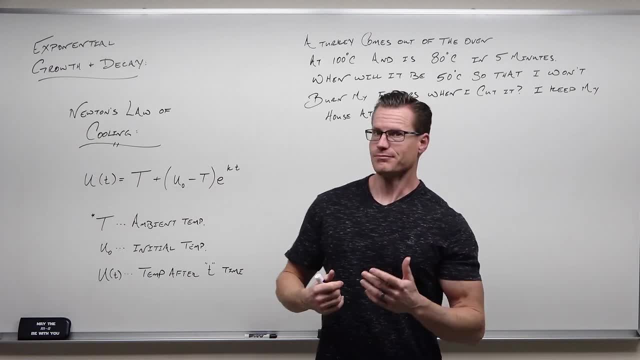 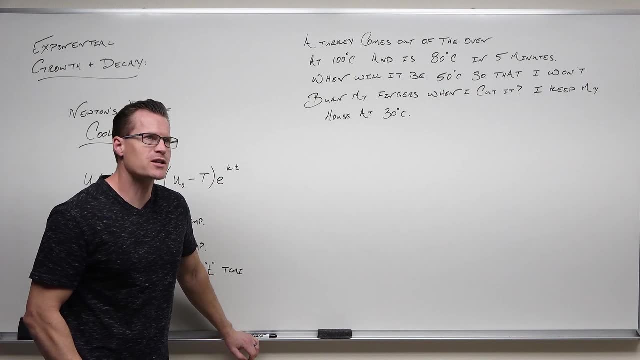 reach a certain temperature. So let's imagine Turkey. I don't actually like turkey comes out of an oven, but some people do, And I am always responsible for carving the turkey. I don't know why, but that's just my job, I guess. 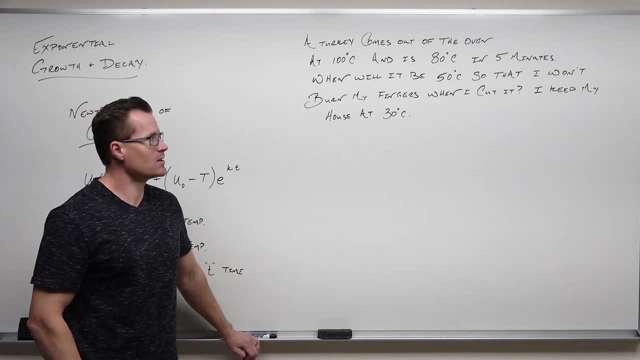 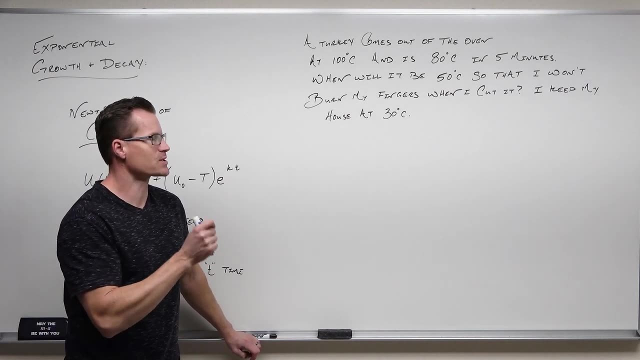 So a turkey comes out of the oven a hundred degrees Celsius and it's 80 degrees Celsius in five minutes. When will it be 50 degrees Celsius? So that I don't burn my fingers when I cut it and I keep my house at 30 degrees Celsius. So I'm going to time this so that 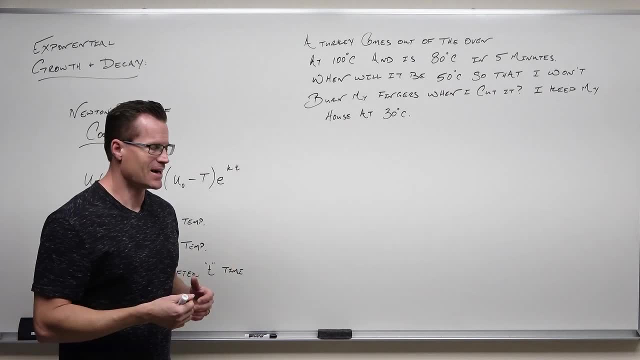 right when I cut it. I cut it, I can serve it. It's nice and hot, People tend to enjoy it, And if you don't think that I actually go through the math to figure this stuff out in your head, you're dead wrong. 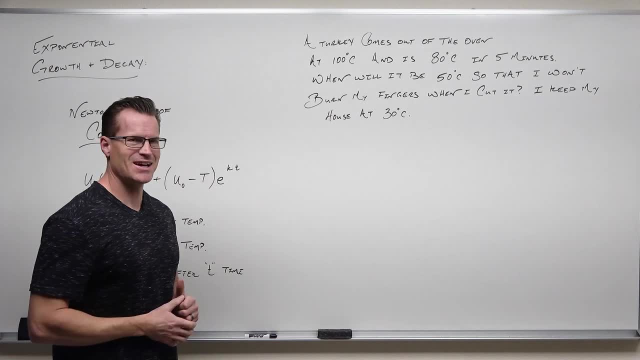 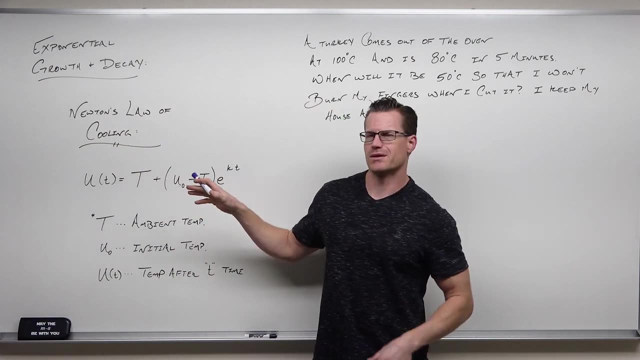 Cause I would certainly do this on Thanksgiving day to make sure that it's just right. So, anyhow, let's go ahead and figure out what all this stuff means. When we deal with Newton's law of coolness, there's a one more variable that you really need to understand. It's the T. T stands for 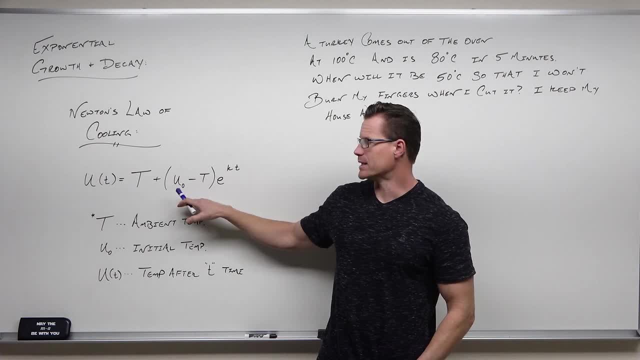 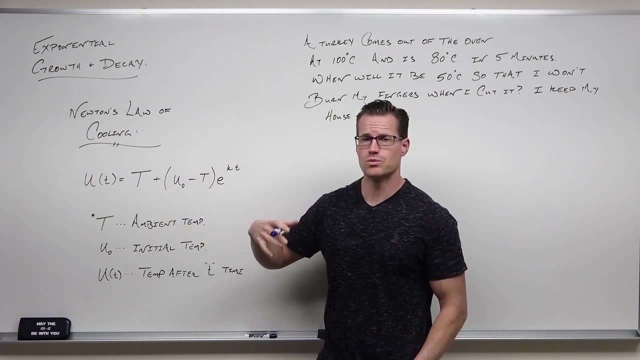 ambient temperature, And so what we do, whether something is higher than or lower than, Newton's law of cooling will tell you a relationship for how long it takes to reach a certain Temperature, or what the temperature will be after a certain amount of time. Now what? 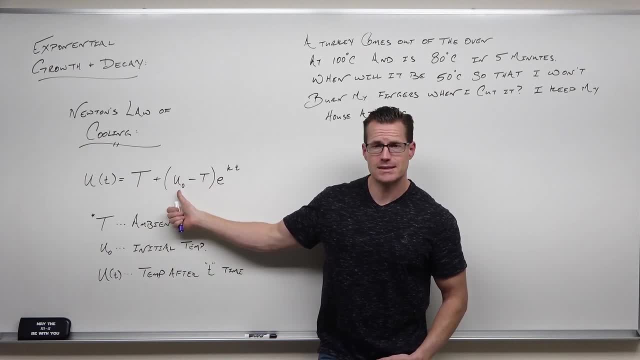 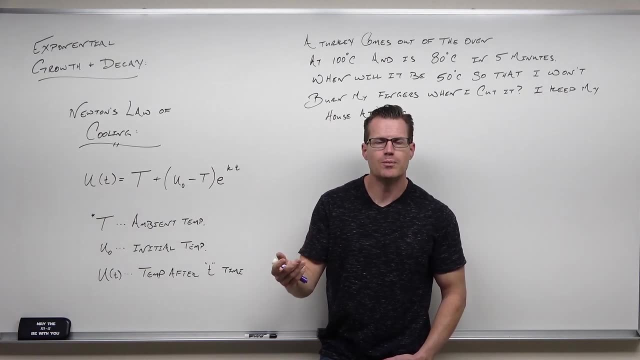 about if that's negative. Well, if you plug in something less than your ambient, then it's cold enough like taking something out of the freezer. Well, that's reverse cooling. It's called heating, but Newton's law of cooling will still work for that. So it compares the. 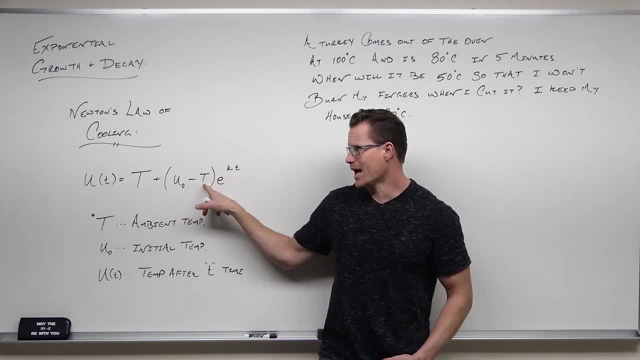 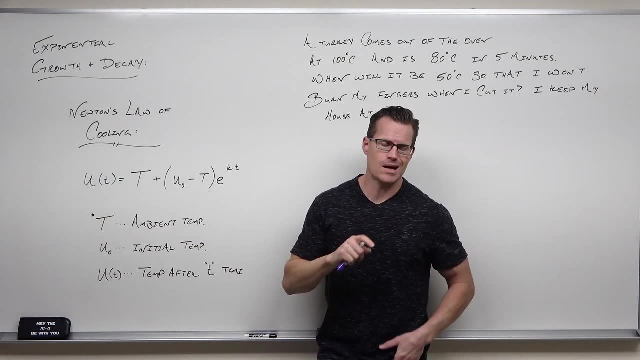 initial temperature of your item with the ambient, And then that is also your ambient temperature. So we're going to fill out a couple of things right now to make sure that we understand that When they say ambient, they mean the temperature of the item. When they say ambient, they mean 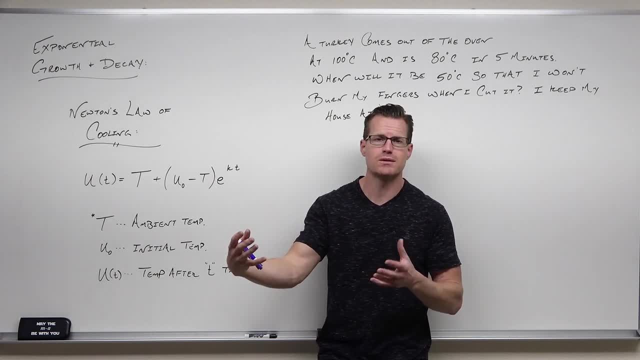 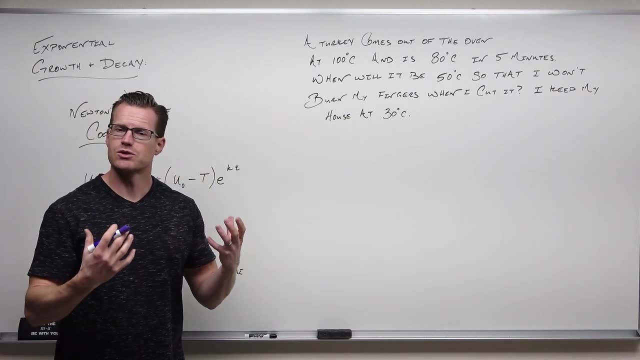 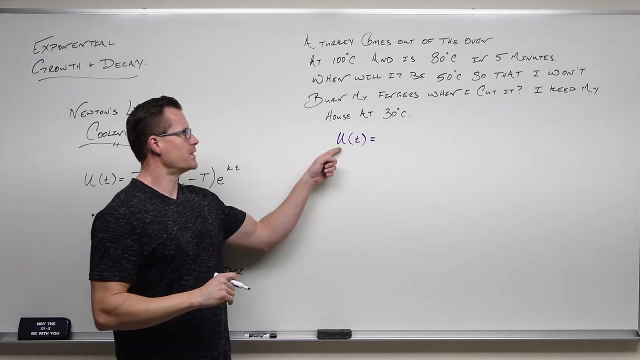 that is the surrounding temperature to which you are exposing this thing that you want to heat or cool. So when we read about the Turkey, the ambient temperature would be the temperature of the house. So the temperature after a certain amount of time is given by. 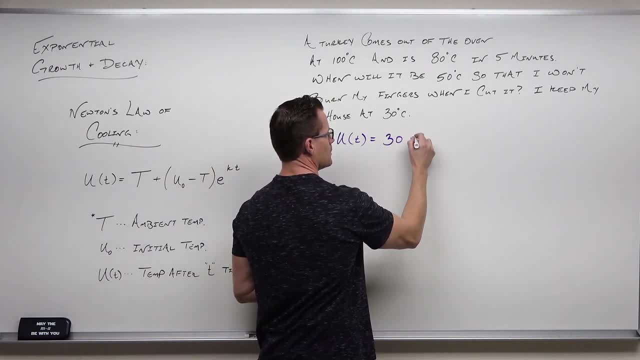 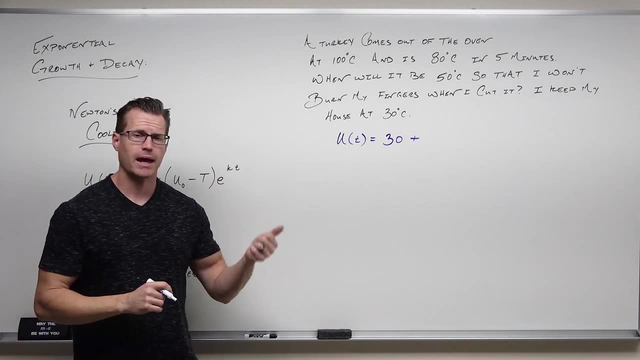 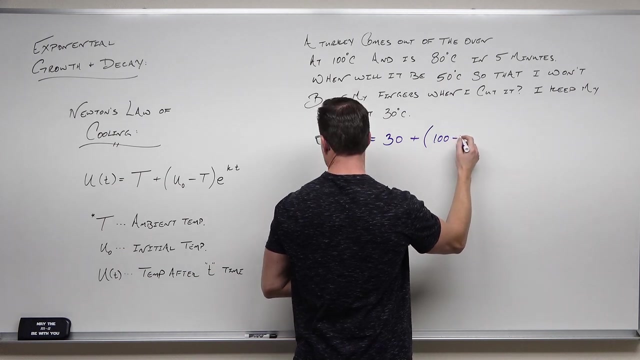 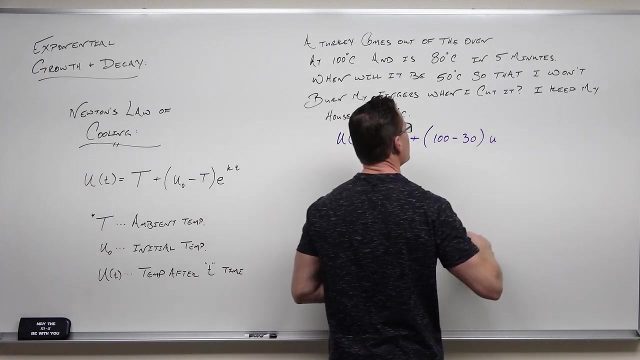 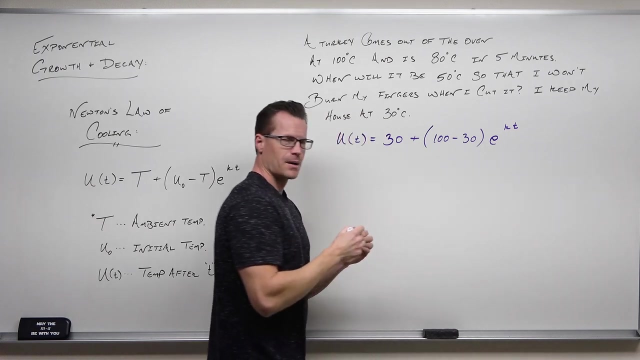 the ambient temperature plus the difference between the thing that you're heating or cooling- in this case the Turkey- and the ambient temperature Going a little slower here because it's newer. So here's what we would say. We'd say the ambient temperature is 30.. 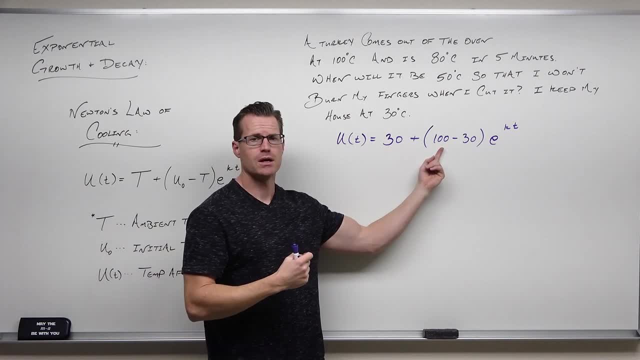 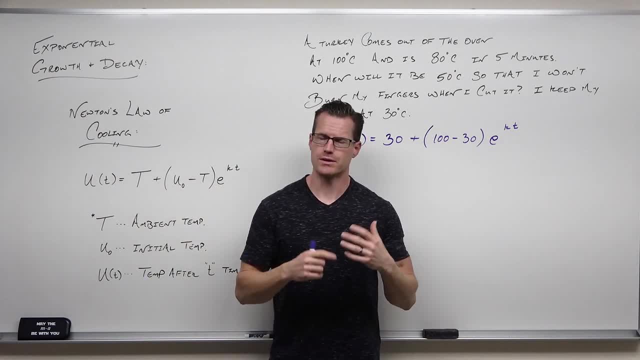 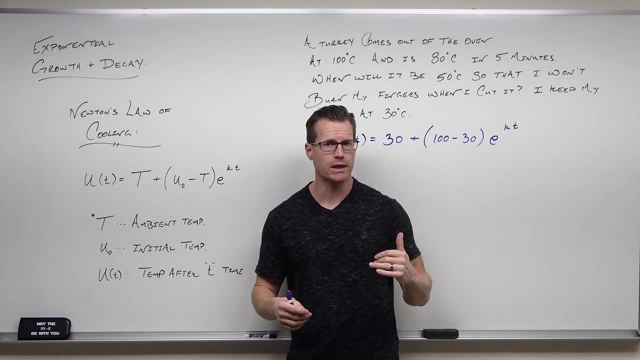 would be 30.. 100 minus 30 is going to give a西. Now keep in mind what we need to do. We have to solve for K first. It's a must. You got to find the rate of cooling or Anticooling heating in this situation First, So we're. 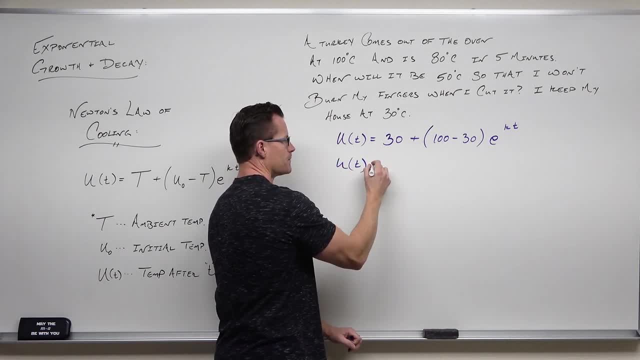 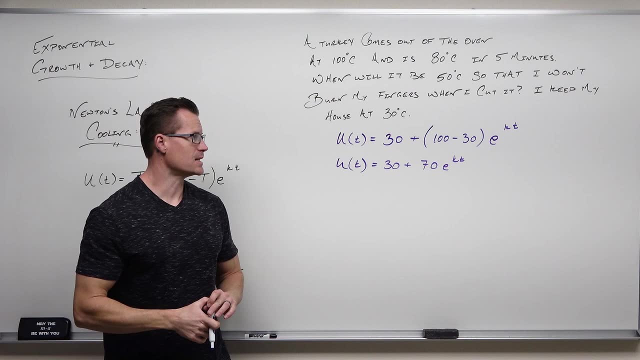 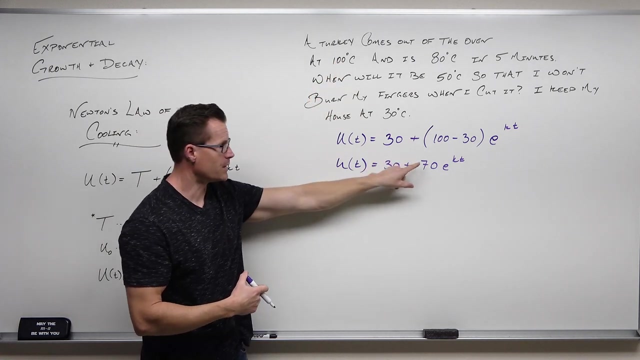 not there yet. I'm just cleaning this up a little bit. So we get 30 plus 70 each of the KTい heat is coming through the end zero. this next statement. So we've said the initial temperature, the initial temperature, right here. 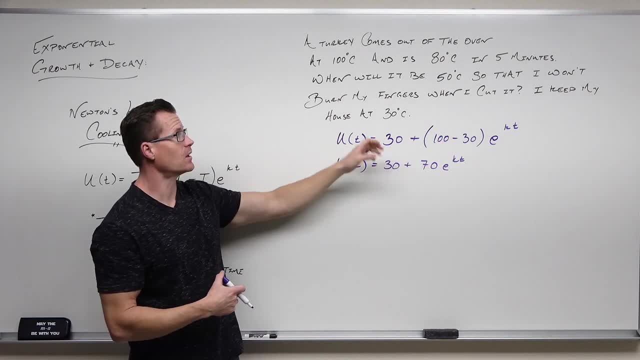 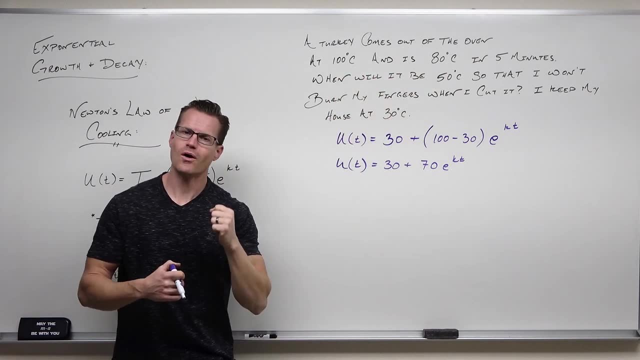 is 100 degrees minus ambient gives us 70.. Okay, Ambient was 30.. We knew that here. We knew that here. Now this next piece: it's 80 degrees in five minutes. Oh, that relates a future value with a time. That is how we go and solve for K. That's how it's been every time. 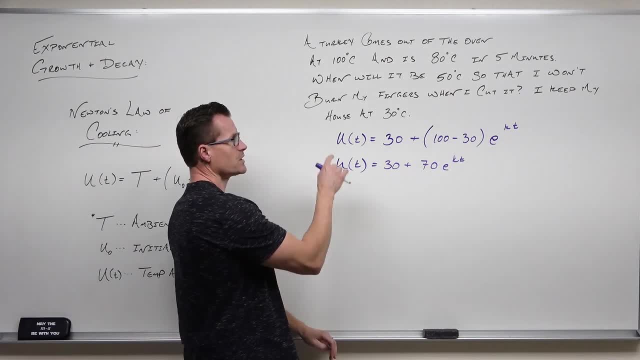 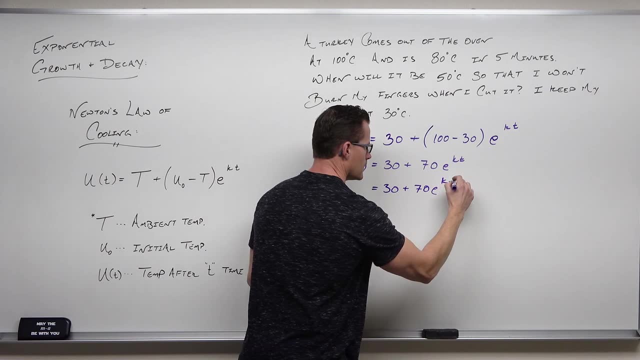 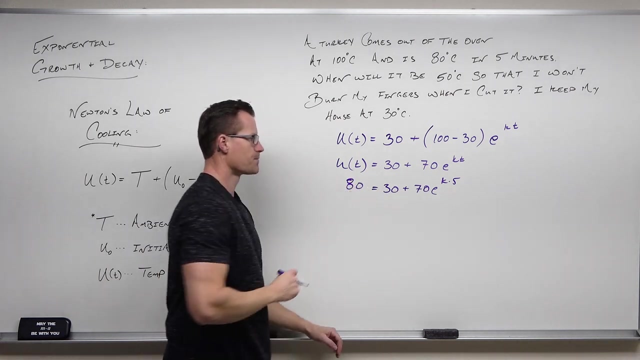 with um extra growth or decay. So in five minutes. so our time unit is minutes. in five minutes, This stuff will equal 80 degrees. That's all there is to it. So it's going to be 80 degrees in five minutes. You still have to obey this. 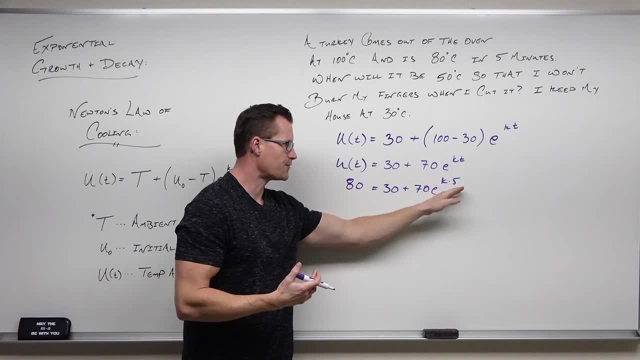 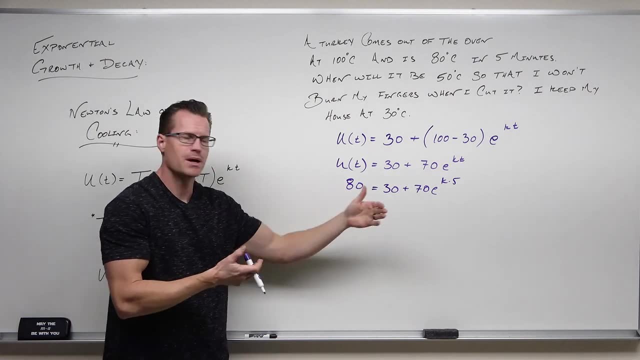 right You still. ambient temperature is still 30.. The difference is still 70. in five minutes It will be 80 degrees. We're going to solve for that K right now. Of course, you have to isolate the exponential right. There's just one more step: Subtract your 30.. 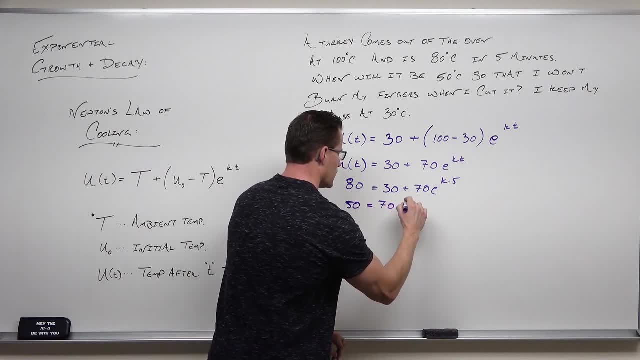 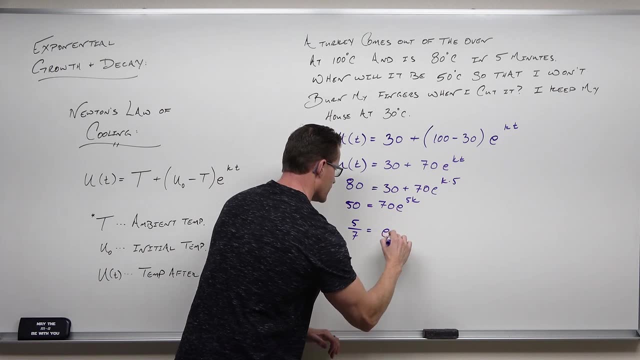 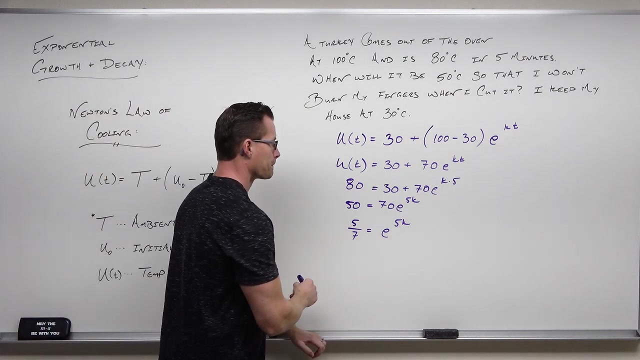 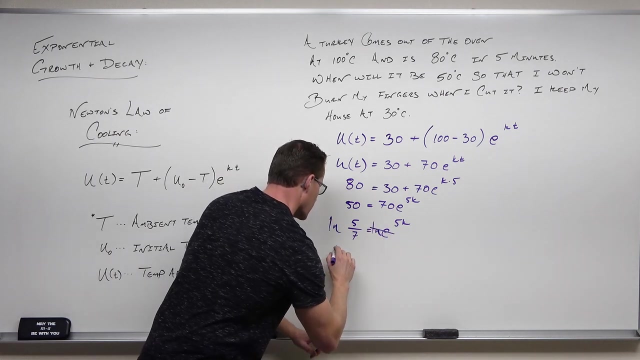 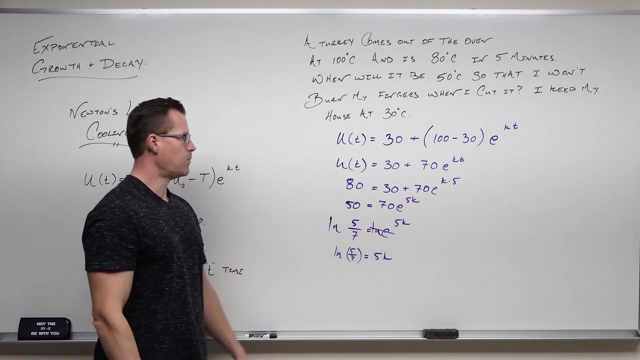 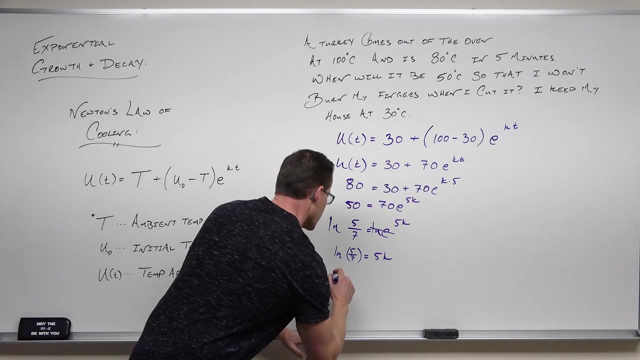 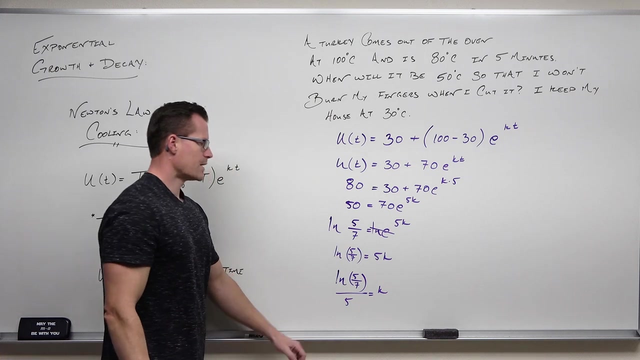 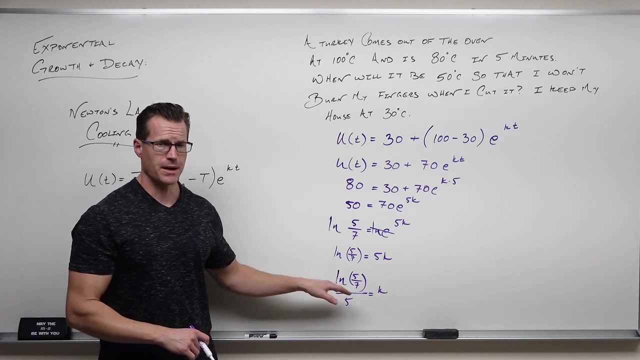 If we divide by 70 and we take an LN on both sides and, lastly, if we divide by five, we have a good expression for K. Now, if I wanted to be very accurate, I wouldn't approximate that, I would leave it, I would put it right there And then, when I 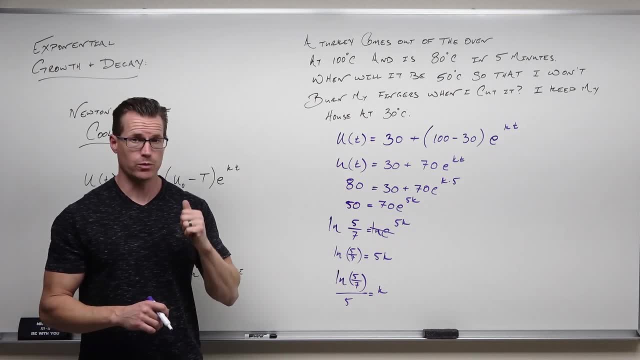 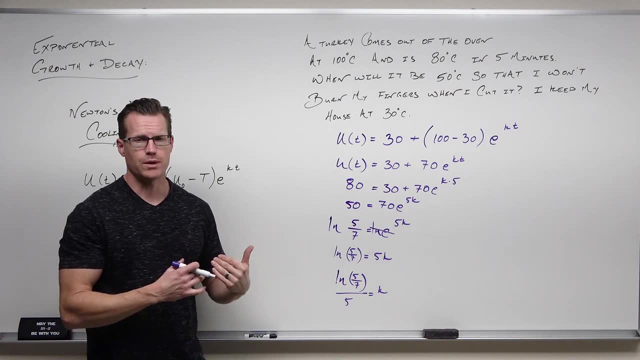 multiplied. when I saw for T, I'd have a very awkward thing to use, but it would be more accurate. I'm going to write a decimal right now, even though I'm going to lose some, some exactness. I want to show you the rate, So that's why I'm doing that. 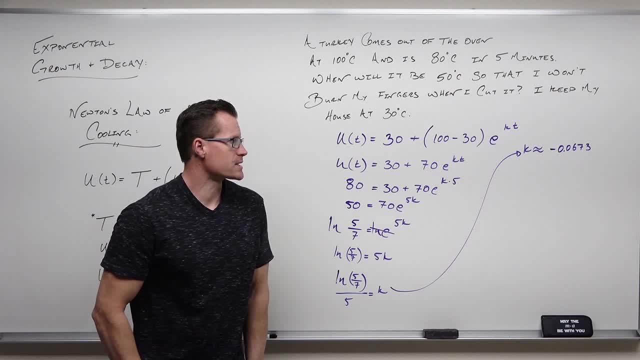 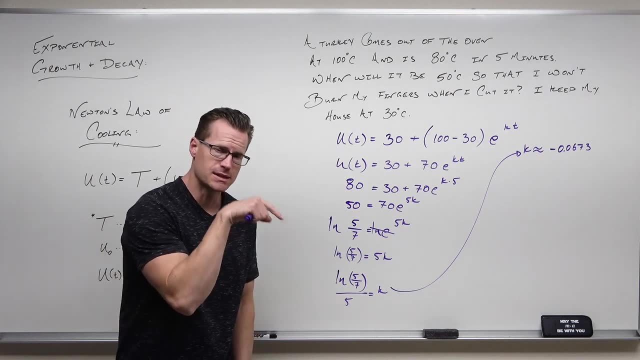 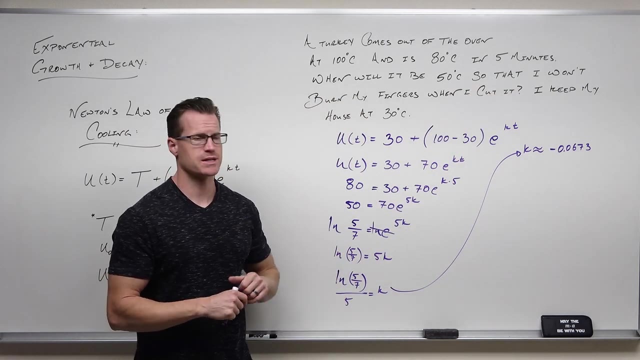 So I got K is about negative 0.0673.. What that says is that there's a a negative 6.73% decrease in temperature every whatever the time period is, every minute. So every minute solution, 6.73% of its temperature. Well, as based on a scale of a hundred. So what that allows us to do. 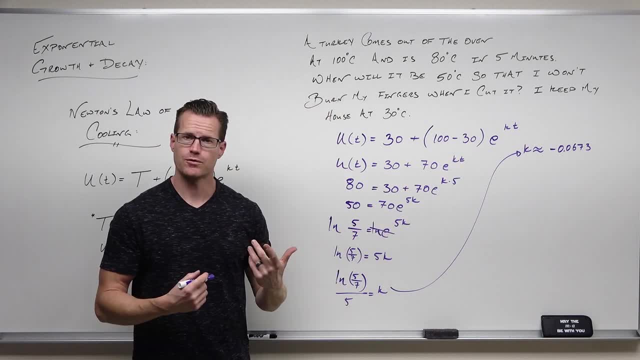 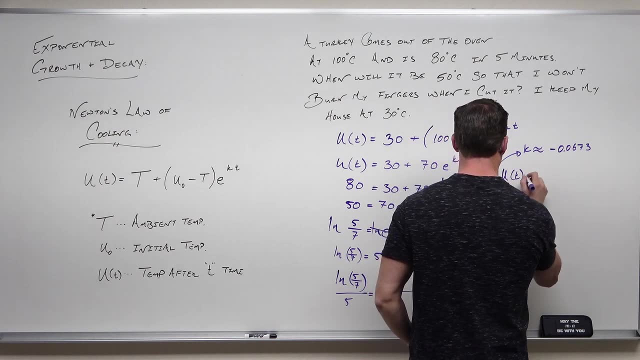 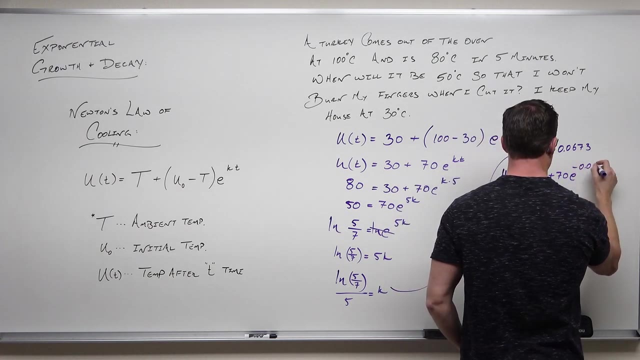 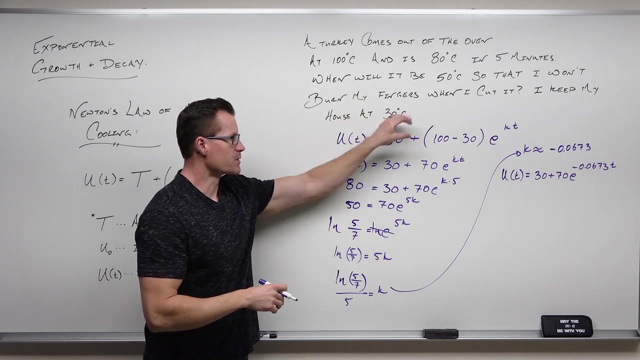 though that allows us to put this right here and then solve for the time it's going to take to reach 50 degrees. So we've understood it. we've put some numbers in the correct place. We've used another piece of information to solve. 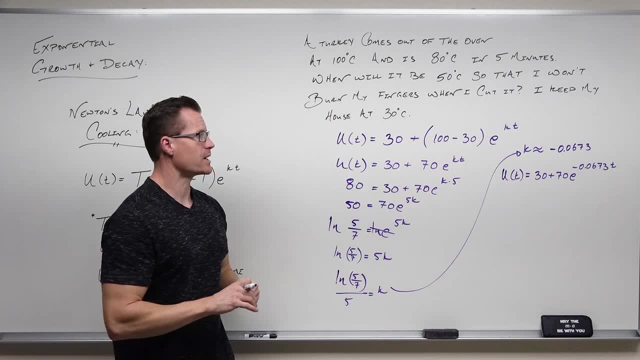 for K, And now we have a formula that's usable for us. So now we're going to answer the last question: How long will it take in order for it to reach 50 degrees? So all this is set: How long says what's? 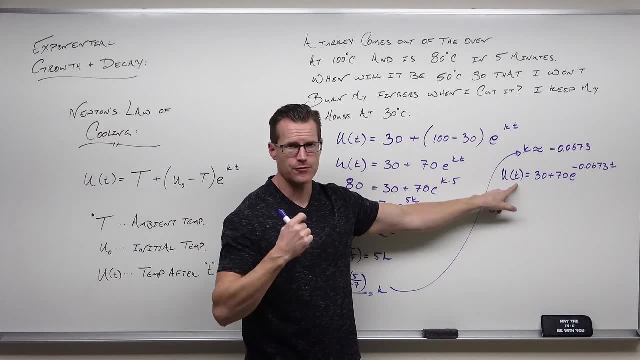 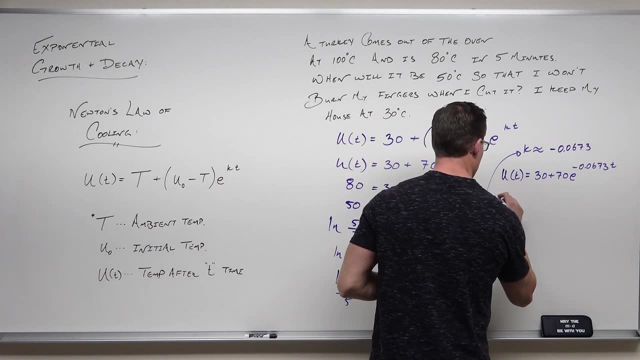 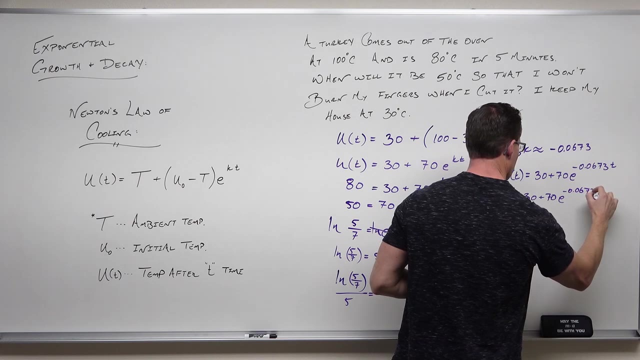 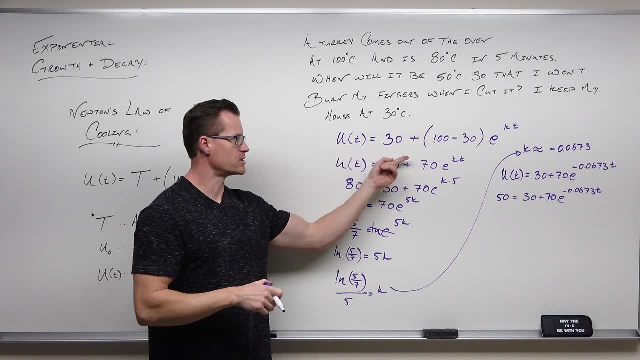 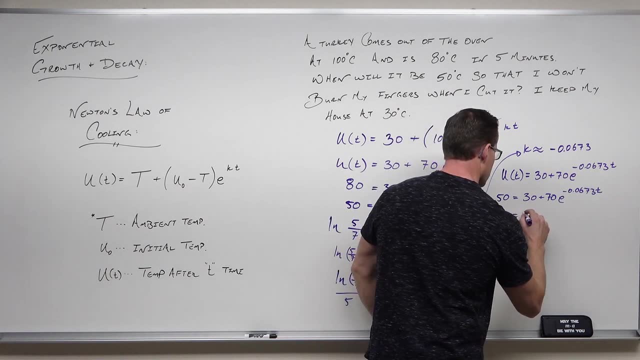 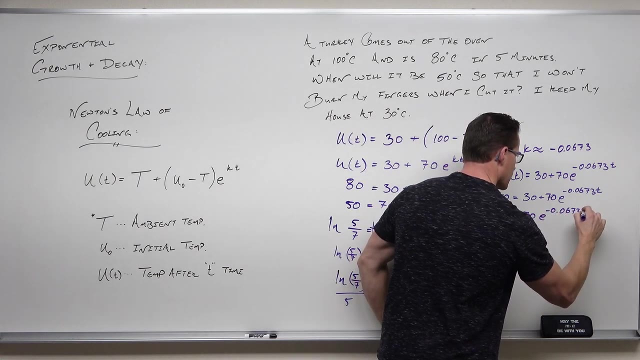 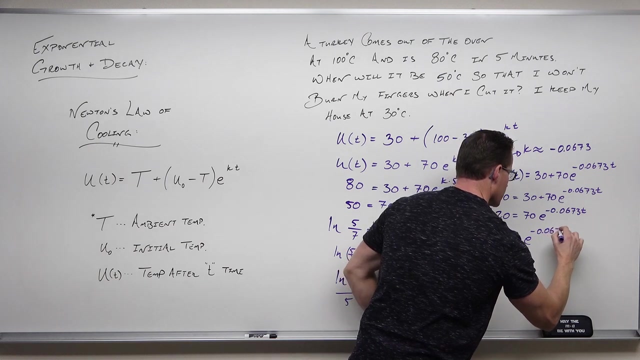 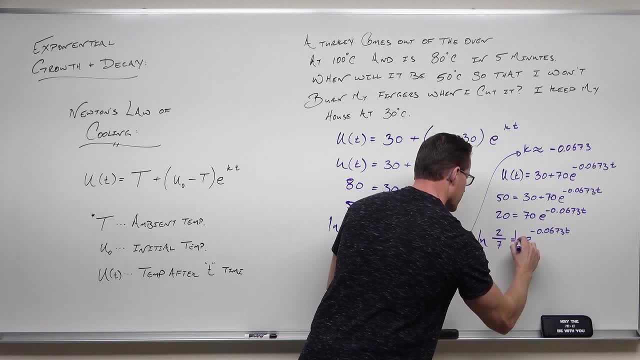 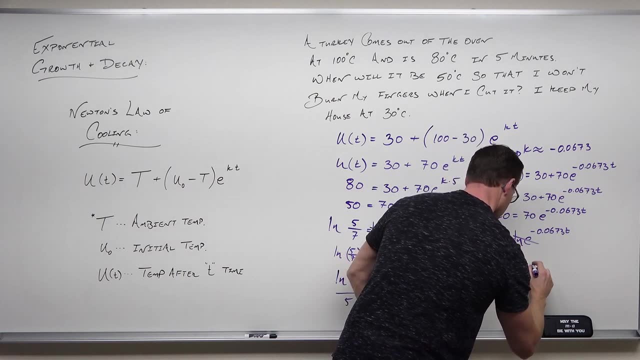 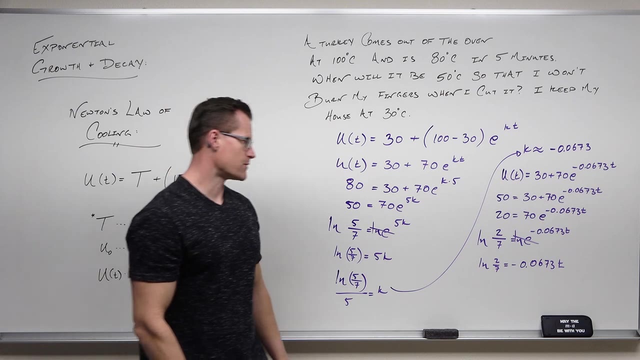 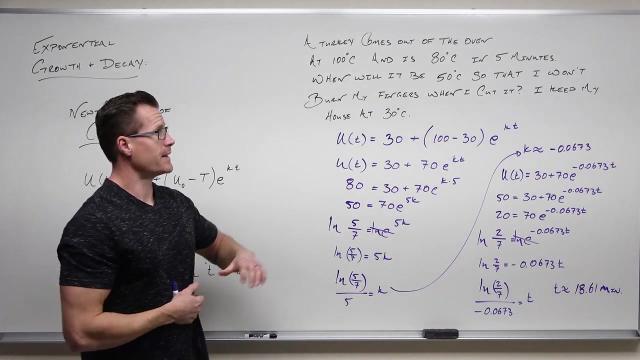 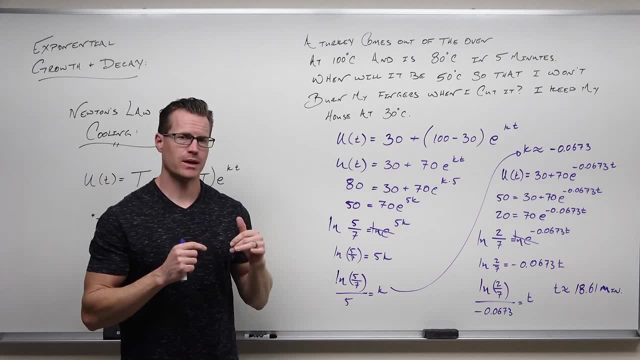 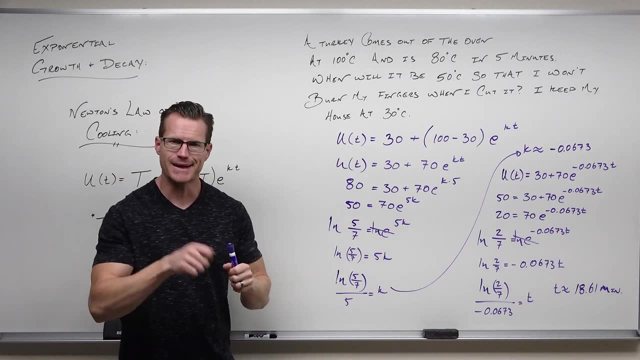 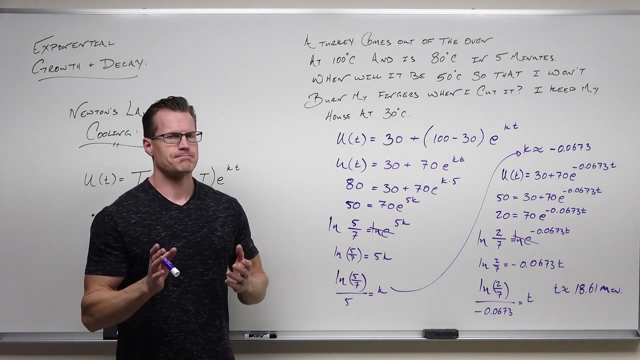 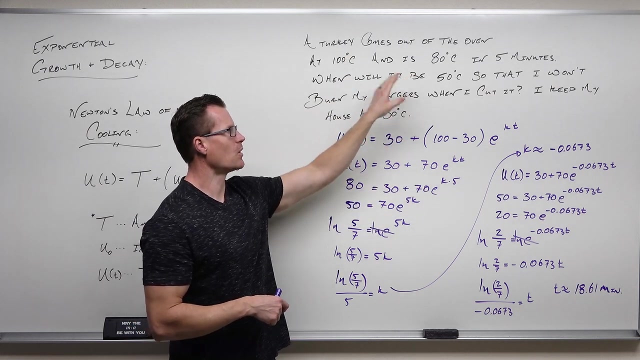 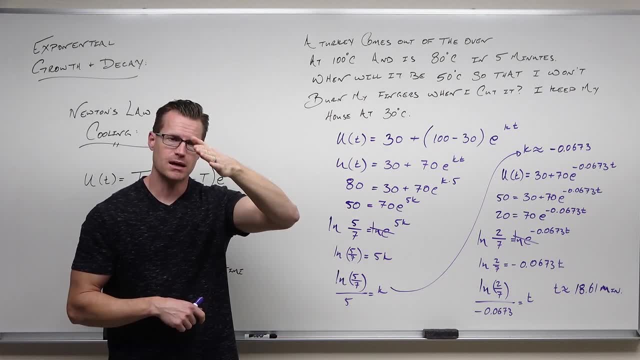 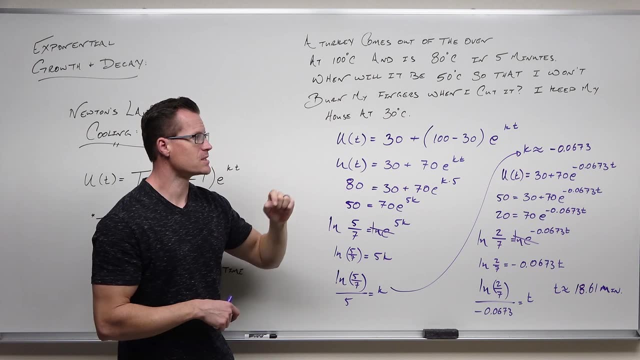 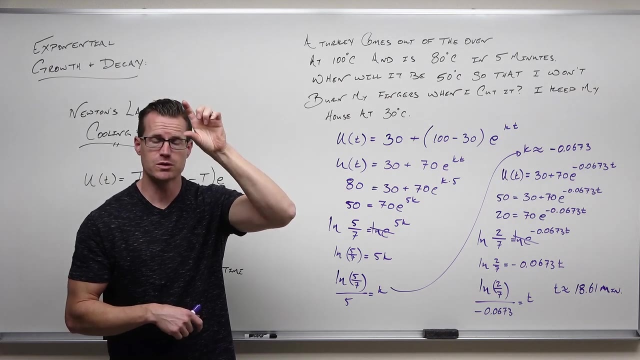 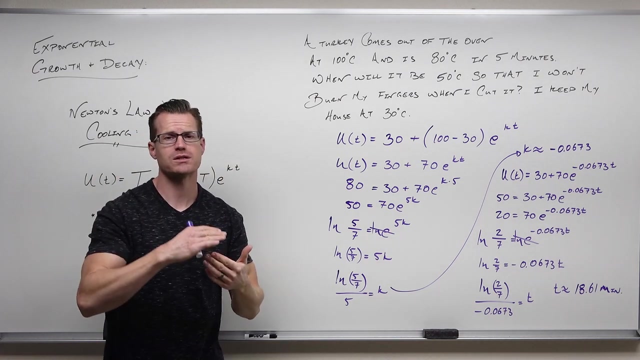 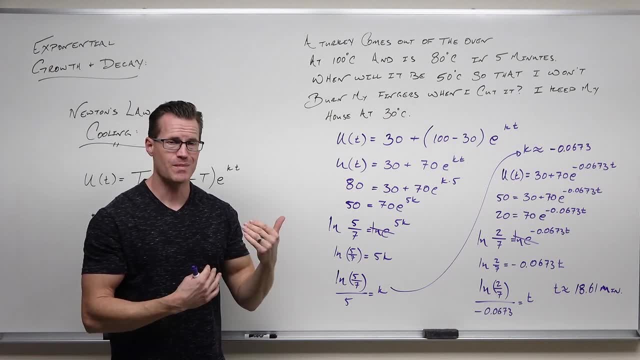 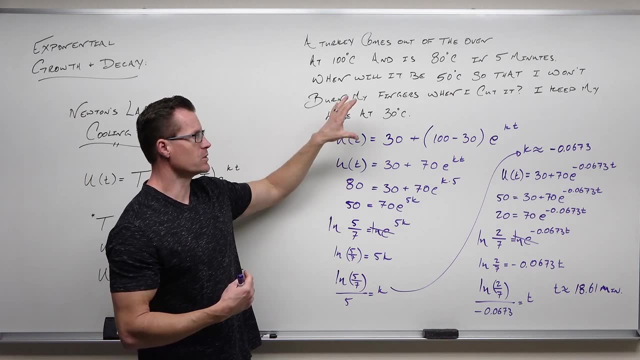 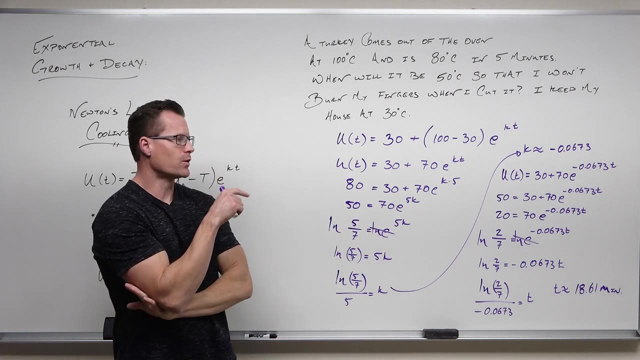 Okay, Okay, Okay, Okay, and less and less, or taking less and less and less away. So it should take longer. it should take longer to lose the same amount of temperature as you start getting cooler or heating up. Theoretically, will this turkey ever reach 30 degrees Ever? Will it ever get down to the point 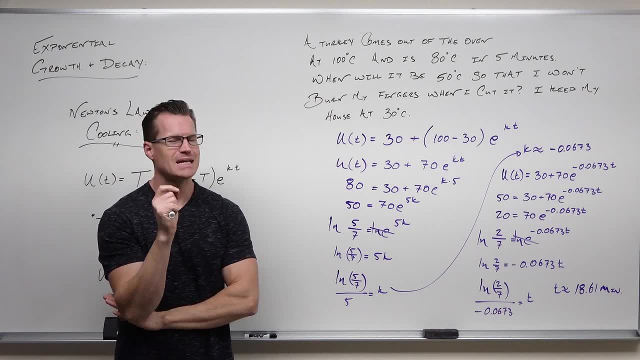 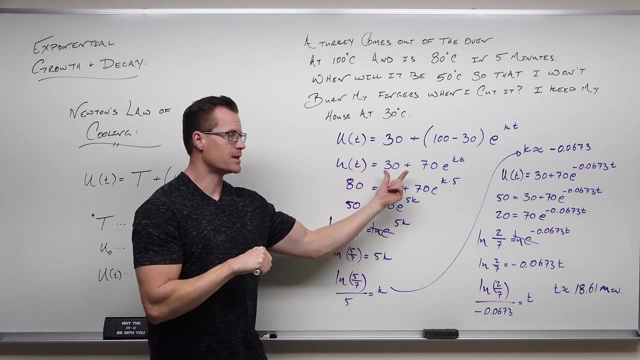 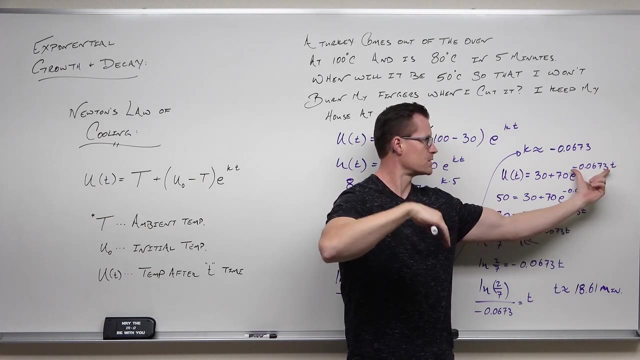 where it's equal to the temperature of my house. theoretically, Practically yeah, Theoretically no, And I need you to see the last thing I'm going to point out. Look right here, This is an exponential. This is an exponential with negative, so a downward exponential decrease in exponential. 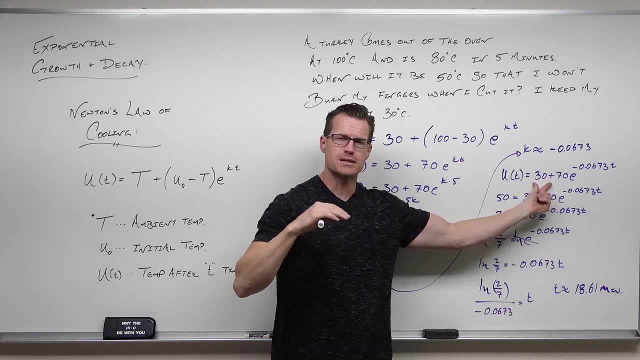 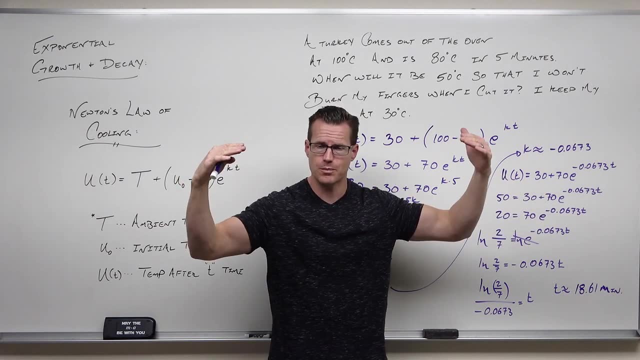 This is a vertical stretch and this right here is a vertical shift. Oh see it, That's a vertical shift up 30.. That's a horizontal asymptote: shift up 30.. This has a horizontal asymptote: It will never theoretically reach 30 degrees. It'll always lose. 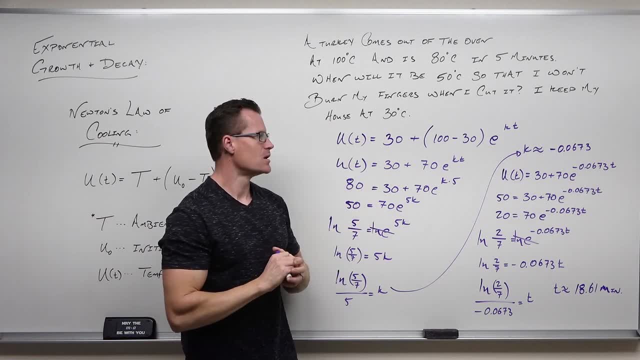 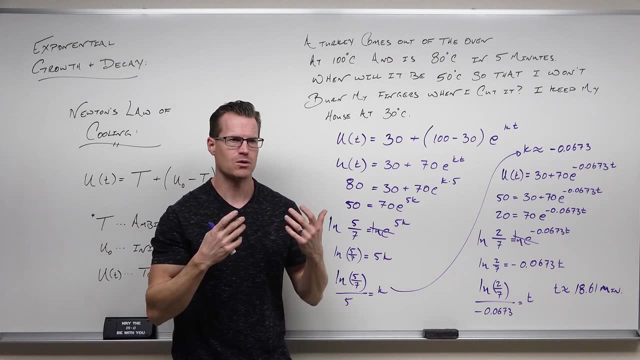 But it'll never. never get down to that, Isn't that interesting? So that's all that interplays with this. I hope that you've seen the exponentials. I've explained it to you. I've really tried to make it as thorough as possible without giving you a background in differential equations. 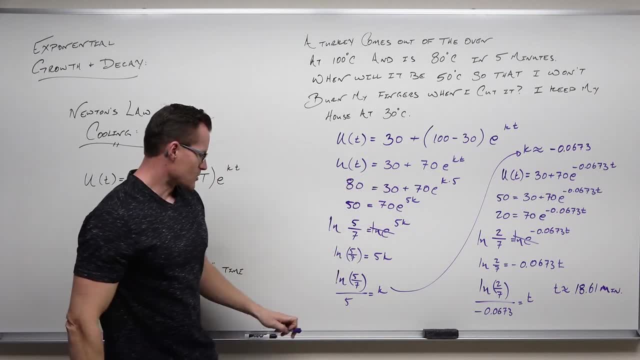 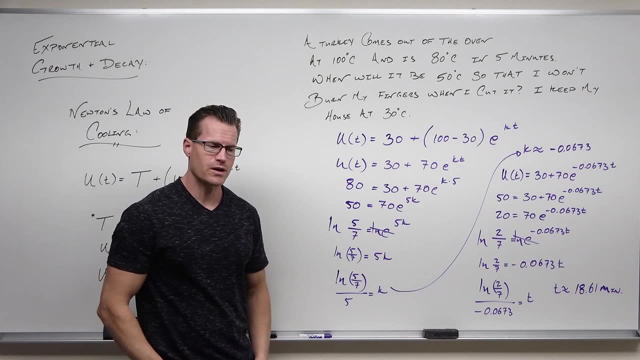 because that's just not the scope of this class. So hopefully it's interesting, Hopefully it made sense to you. And we are now. we're really done with our exponentials. That's about as much as I can teach you. We're going to move on to something completely different. We're going to 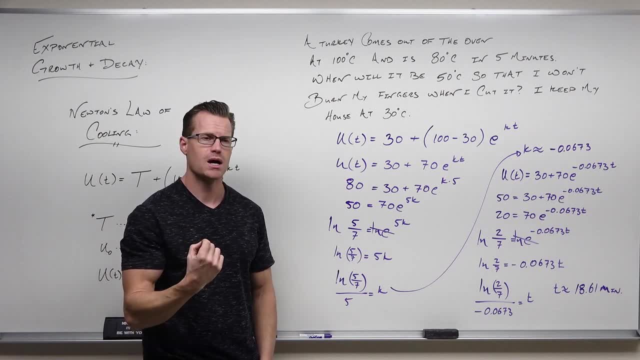 move on to sequences and series. Now. they do relate to exponentials, but they are a different thing. So I'm going to move on to a series Now. they do relate to exponentials idea, So we'll talk about those. I'll give an introduction to sequences, an